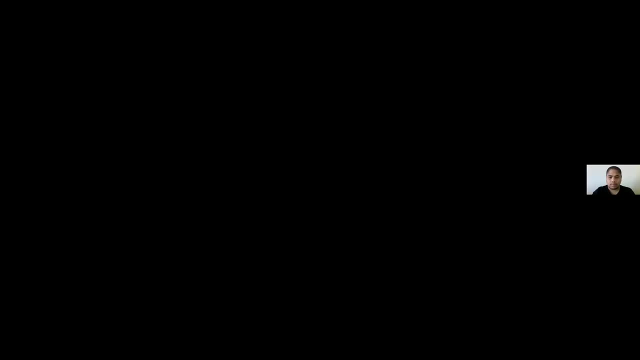 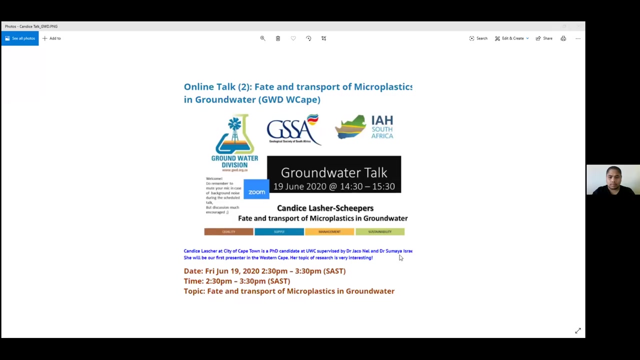 Good afternoon everyone. So we've had about a hundred people show interest in the event and we are on just over 60 at the moment. I think we'll give a few moments. As you enter, would you please add your name and surname in the chat here. 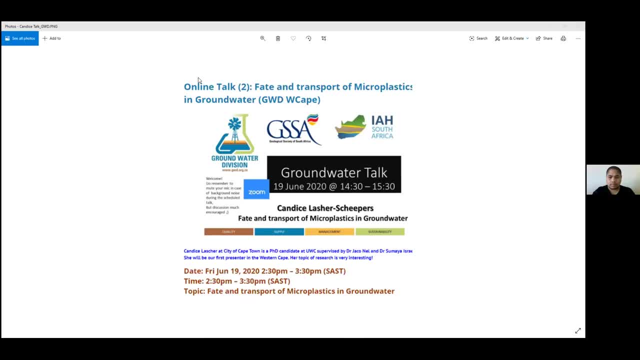 It's for record purposes and to ensure that you can earn CPD points for attending. I think that will be a great idea, Yep, And you can watch. Thank you, Ms Michelle. Hello everyone, I'm Michelle Latham. 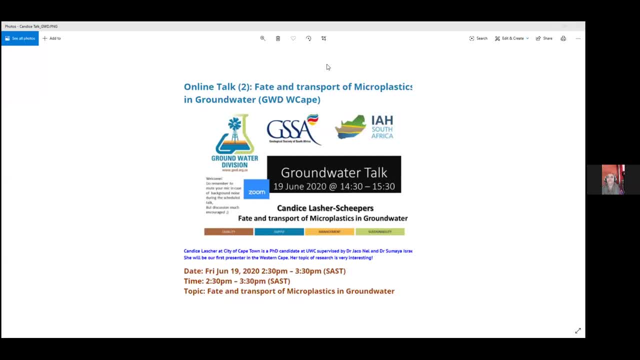 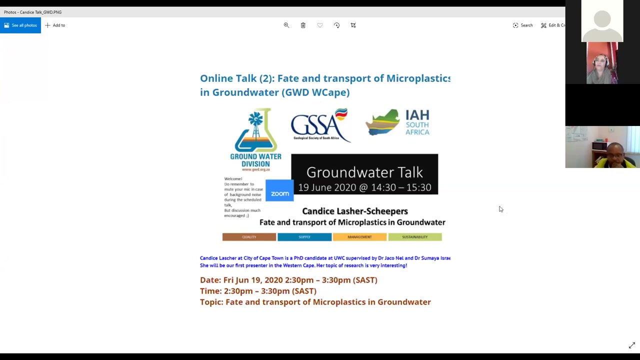 I'm the logo officer for the Lear County School District. Thank you, And this is a presentation of the format. Thank you, Thank you, Thank you. Good afternoon everyone. We are going to be glad to join To those of you who are already in the session. 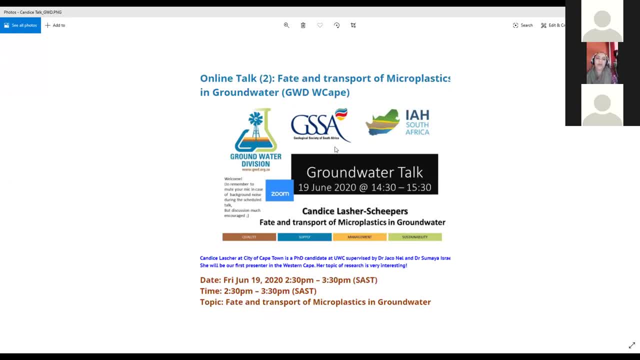 please add your name and chat area for your purpose, in which you can receive your CPC for the next few days. Thank you, Thank you. Thank you. This was a conversation we had in the middle of the event. The events had been discussed. 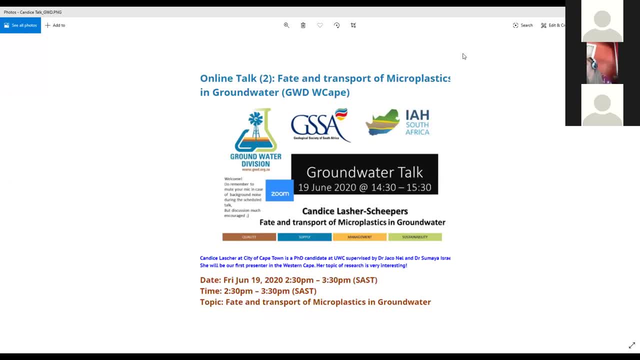 So please join us, Thank you. Thank you, We'll be starting in the next minute or so. People just enter your name in the chat area. Thank you, No volume. Why did you turn it off? Good, I see some people are having difficulty. 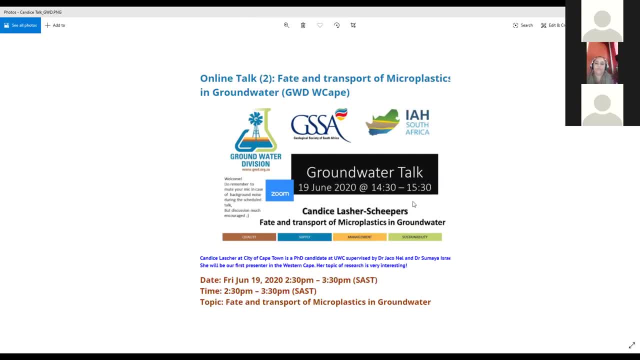 Okay, Okay, Good afternoon everyone. So as not to waste time, I'd like to start and welcome everyone to the webinar. Thank you, I welcome you all. Thank you for joining today's session. It's the first of its kind for the groundwater division for the Western Cape. 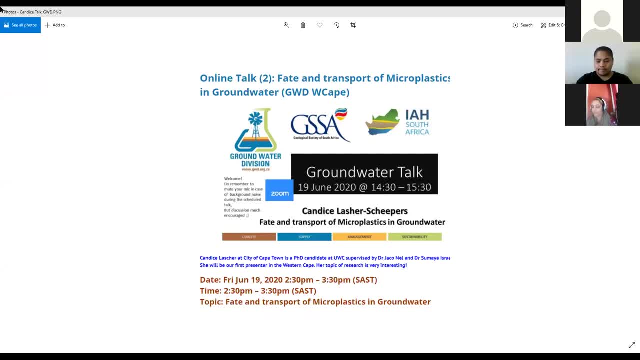 I'd like to give a special thanks and welcome to the members from other parts of the country. We have the pleasure of having our national chairperson with us today, Mr Faunus Buri. Thank you for joining us, Thank you. 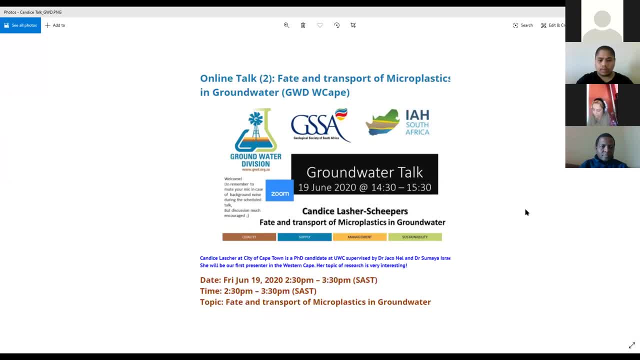 Thank you, Mr President. Thank you, Thank you so much. I appreciate your introspection. It's been very useful. Thank you very much. Thank you, Thank you. Thank you, Ms Buri. Um just a few rules or few important pointers. 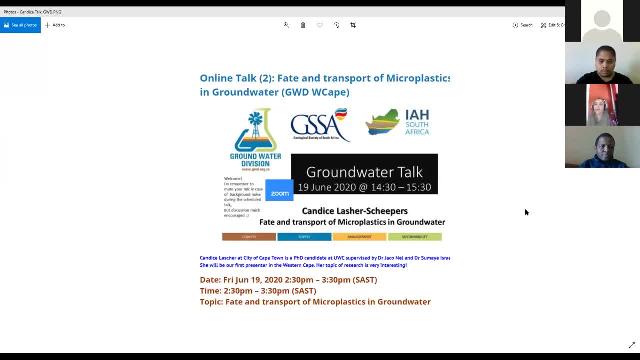 For those who are new to Zoom, please mute your mouse, or the co-host will be muting your mouse so that we minimize interference. Um, people who are new to groundwater division, or if this is your first ever, you are welcome to join by the dry lipsera. 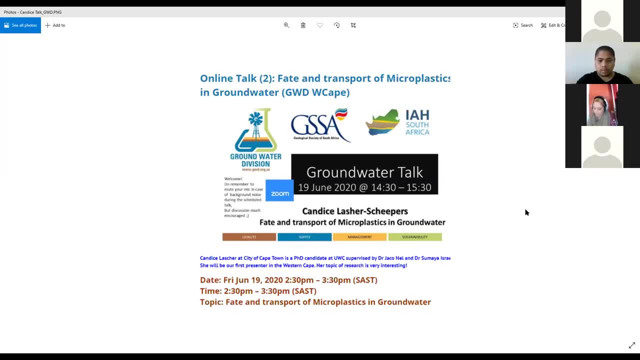 The most important thing is that we want to remind everybody that they can't use their earphones. You can't do it without them, Oh, and you can't do it without your earphones, So they're. because you can't hear from your earphones, so you can't hear from their. 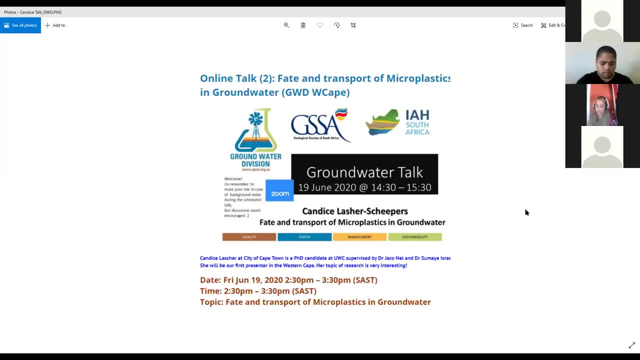 You are welcome to join by the dry leather blousons. Today we have Mrs Lasher. she is from the city of Cape Town, a registered PhD student at UWC, and she will be talking to us about the faith and transport of micro-elastics in the groundwater. 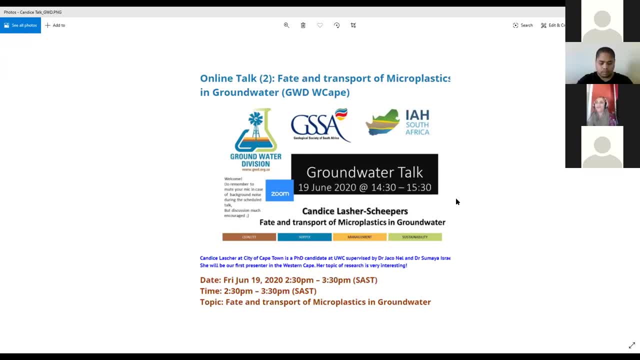 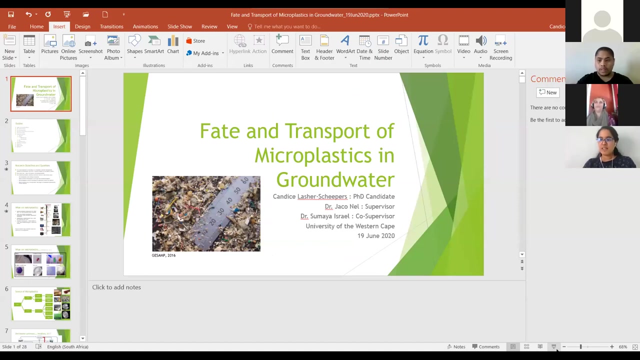 I will now hand over to Candice. Hi, good afternoon everyone, and thanks for joining. Okay, so I'll just get into it. Can you hear me? Everything's fine. Okay, Please forgive me. I'm very nervous. I haven't spoken to a lot of people in a long time. 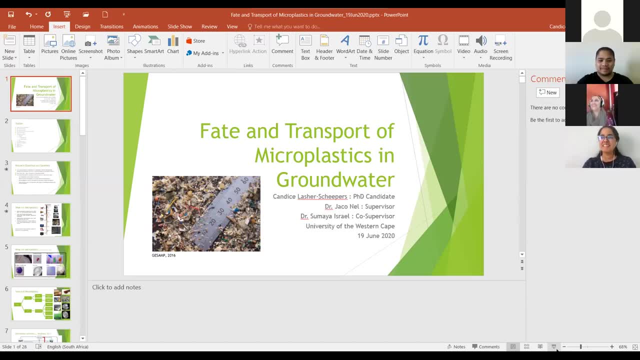 It's been locked down for a few months now, And I also got out of my pajamas today for you guys. So yay, here we go. So the title: faith and transport of micro-elastics in groundwater. I'll just give you an overview of the literature review that I've done so far. 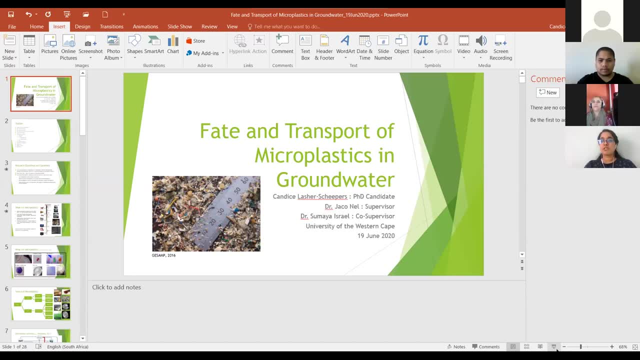 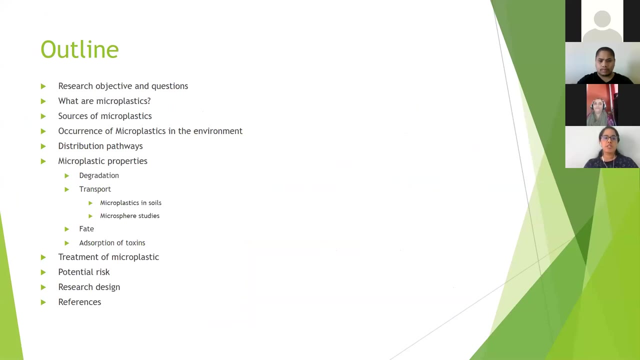 And a little bit of progress to date in terms of the project and what we've done so far. Yeah, So I'll go through the outline quickly. So we'll just go through research objectives and questions. We'll talk about what micro-elastics are, where we find them, how they travel. 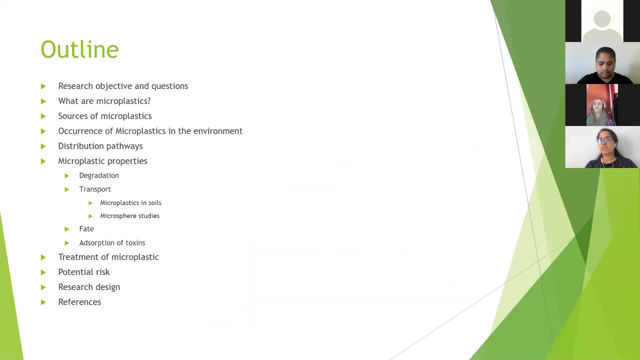 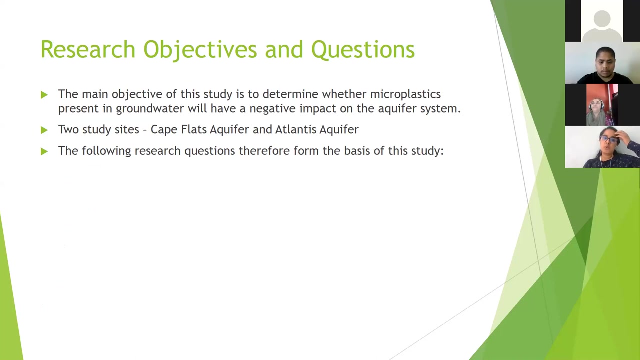 And then some of the properties like degradation, transportation, and then the faith. We'll discuss a short, brief discussion on micro-elastics and then potential risks And then we'll go into the research design. So the research objectives and questions. So the main objective of the study is to determine whether micro-elastics present in groundwater will have a negative impact on an aquifer system. 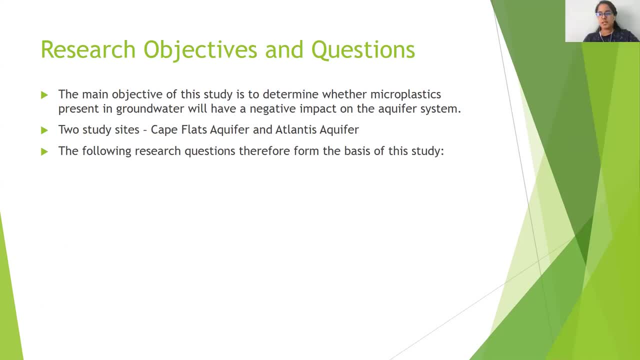 So I'll use two case studies. I'm using the Cape Flat aquifer And I'm using the Atlantis aquifer, And so the following questions. So we all know that with the city of Cape Town, The city of Cape Town is developing two managed aquifer recharge schemes. 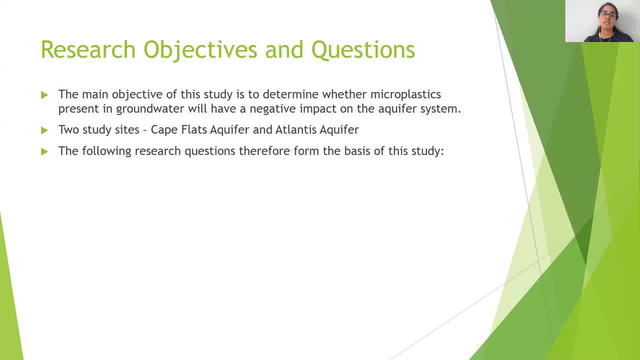 One is already developed, operating for almost 40 years now. The other one is the new one, which is your Atlantis managed aquifer recharge scheme. So the study will definitely benefit the city in understanding and determining whether there will be an impact. 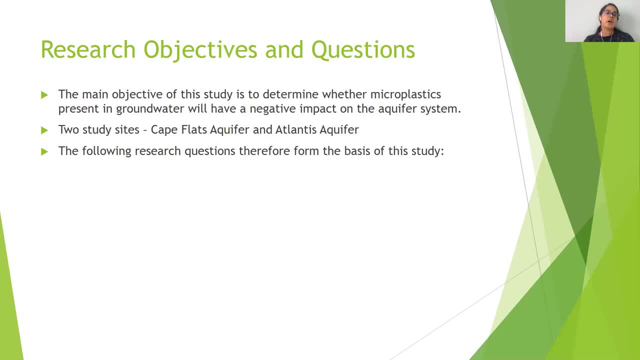 And then we know how to manage and control the problem. So the following research questions Therefore form the basis of the study: Will micro-elastics move through the aquifers? What is the fate of micro-elastics in the Cape Flat aquifer and in the Atlantis aquifer? 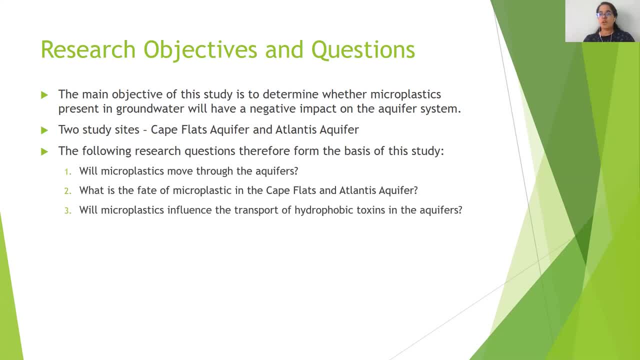 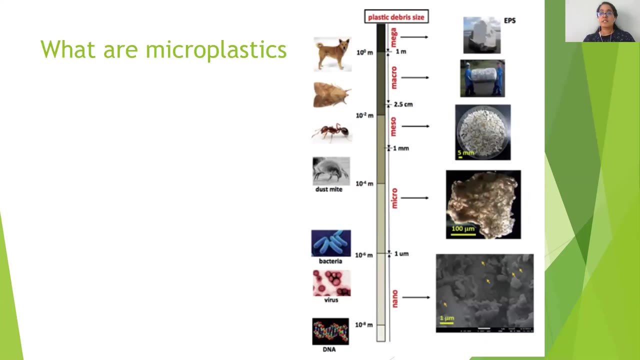 Will micro-elastics influence the transport of hydrophobic toxins in an aquifer And what is the best way to manage and or limit impact of micro-elastic contamination in these aquifers? So we did have a look at the scale. What are micro-elastics? 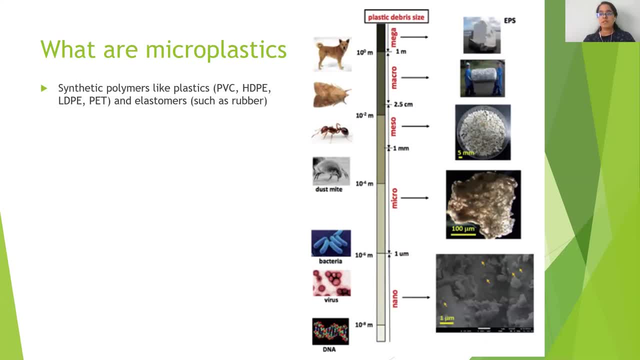 So we know that micro-elastics are synthetic polymers like plastics or elastomers, Plastics- we're all familiar with them. So we've got HDPE, LDPE, polyethylene, PET- I'm not going to say these names because they're very tongue-twisting. 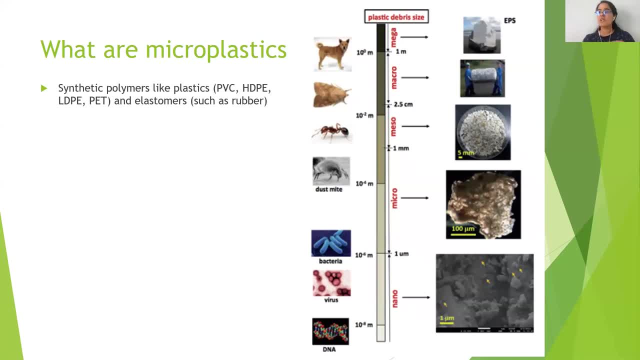 We've got PVC. As a hydrogeologist, we know PVC. We use it all the time in paintings of well points and so forth, And we know HDPE as well, And then a lot of them. we see it every day. 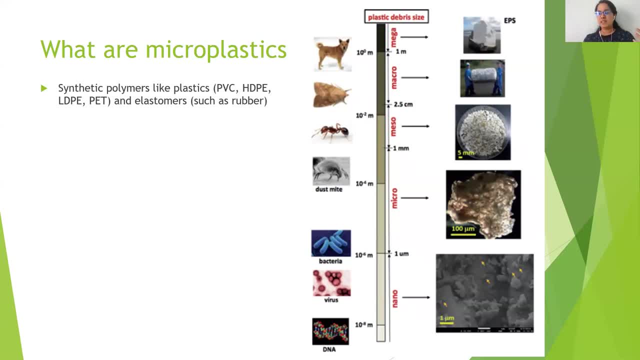 Like: look around you at this very moment, Somewhere you are touching plastic or it's somewhere around you. There's just no running away from plastic, It's all over. And then plastics have additives in them. Why do they include additives in plastics? 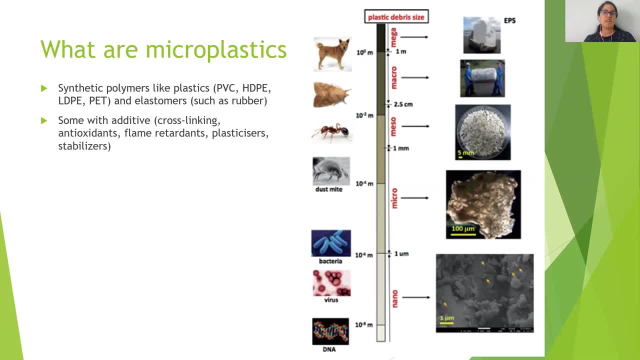 So it's either to make it flame resistant, So you'll have a flame retardant in. You have long chains of polymers, So you've got cross-linking additives which join the chains. You've got antioxidants so that they don't break down. 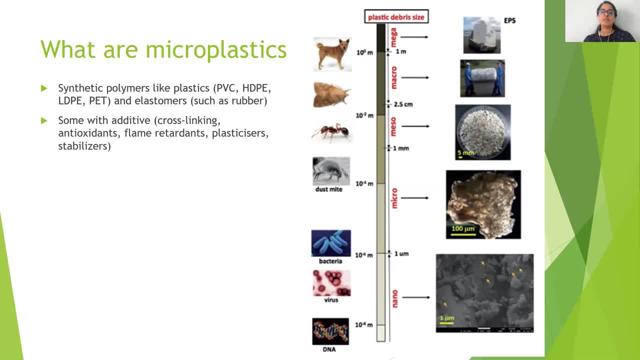 In certain environments. You've got pesticides, You've got stabilizers, So it can either make it flexible, It can make it hard. So that's why you add, So that's why they include additives to plastics And then. so, basically, the overall topic is plastic. 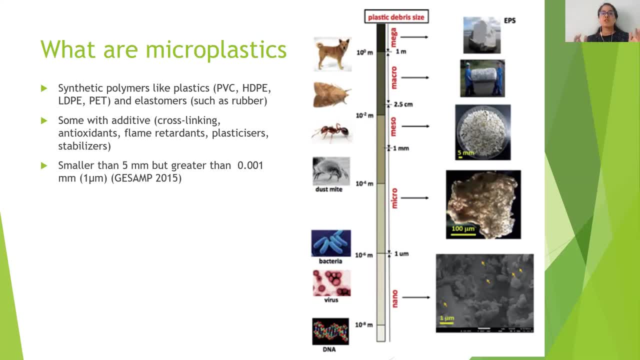 But then it's broken down into microplastics. So microplastics They don't belong in which categories. So microplastics are put in in cemeteries. So microplastics will, can actually and can easily in European countries. 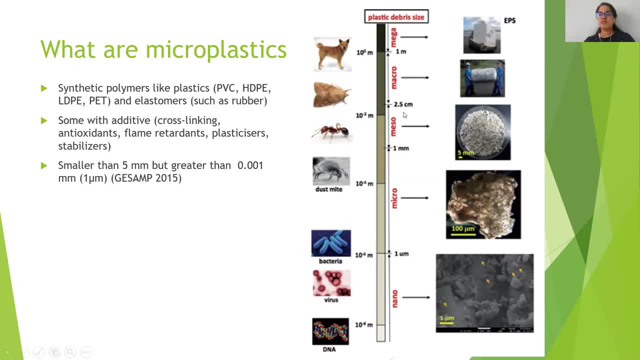 However, they usually cannot be mixed into plastics Or it can be accidentally mixed into the subjective factors. For instance, most semi-perishable plastic bales millimeters, and we've just got a comparison to ants, and then we've got your micro sizes. 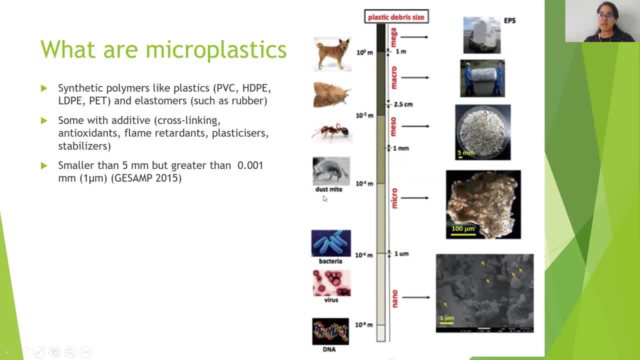 which is you've got a comparison to dust mites, and then we've got nano sizes, which is your bacteria, your viruses, your DNA. so we get really, really small particles um dust. research will focus on microplastics. um not sure we'll do nanoplastics um it is. 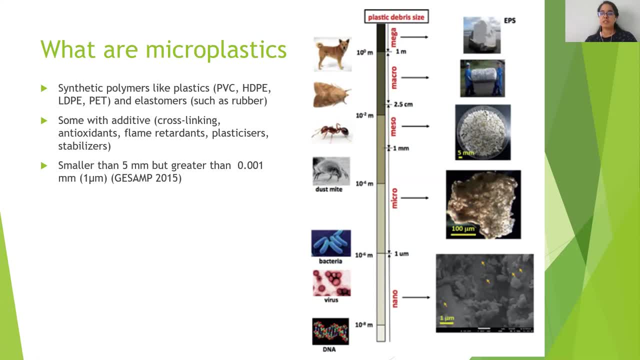 I mean, detecting it is a problem, or at least it's still something that that we work, that's that the researchers are working on. so for the study, we'll work on microplastics, and then plastics itself have different things, so you've got like really, really light plastic. so you've got your 0.06 density. 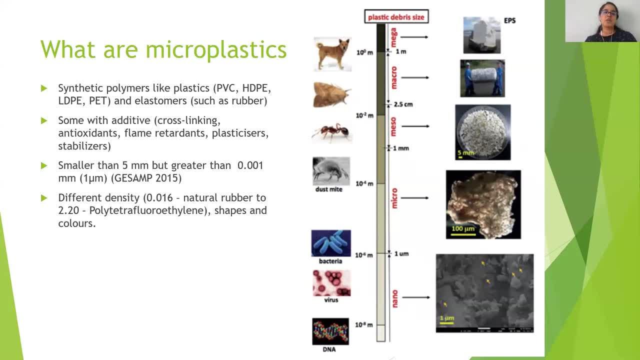 um, which is natural rubbers, and then you've got um a density of 2.2, which is your poly tetra flora ethylene. that um, they, they kind of they use that to coat pans. so you've got the, also known as teflon. so plastics come in different types, it comes in different types, and then you've got. 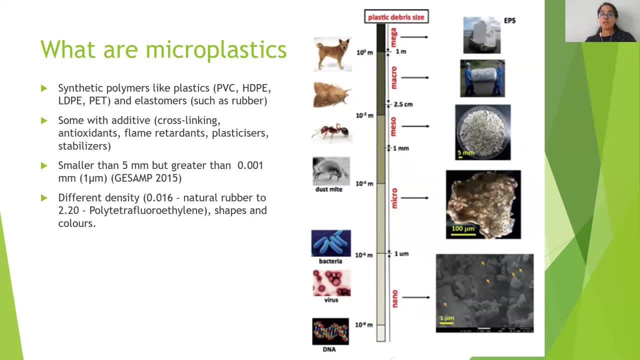 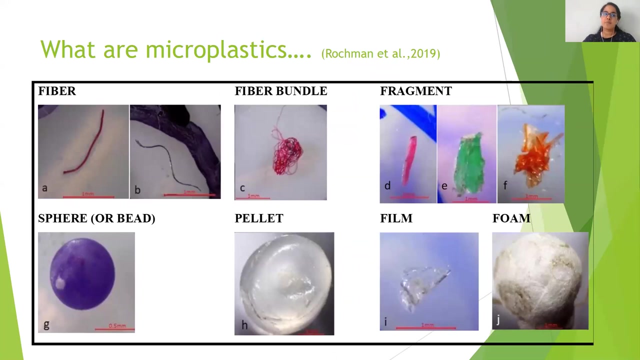 it has different densities. um, your microplastics itself comes in different shapes and then it also has different colors, and I've mentioned this- that anything smaller than one micrometer is then referred to as nanoplastics. so we've got a look. we have had a look at um different types, shapes of microplastics. 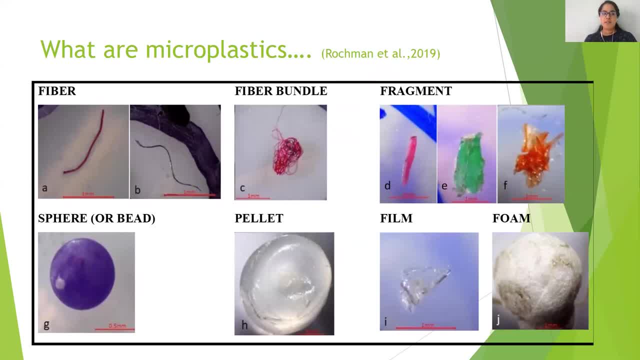 and so we can see: we've got fibers, um, but then fibers are also classified. you've got your clean cut edges of fiber, and then you've got your frayed edges of fiber- um. then you've got your fiber bundles, and and research shows that fiber bundles almost really like untangled, so they stay in that. 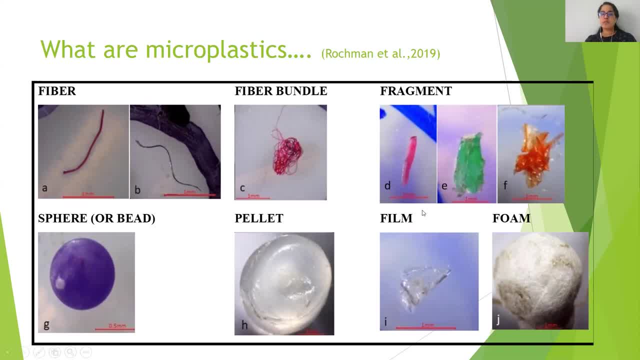 knot form. then you've got your fragments which occur in foam as foam, and sorry, oops, sorry, sorry. you've got fragments. so d, e and f. you've got your rigid and your irregular fragments, and then you've got spheres, or known as beads. they're round and smooth. we've got pellets. 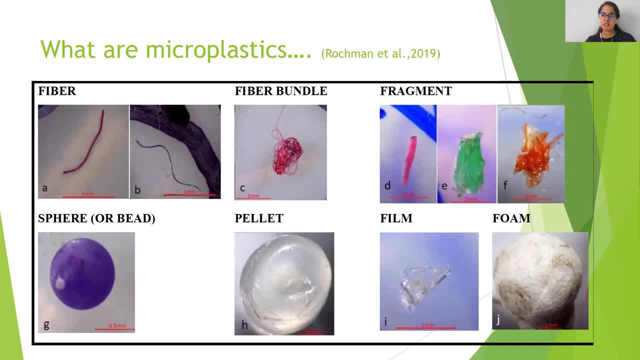 also round and smooth, but they can also come in cylinder shapes. and then you've got your foams which are flat, thin and malleable- malleable, um. and then you've got your foam which is soft and compressible. I'm sure all of you are looking at this now and you can somewhat 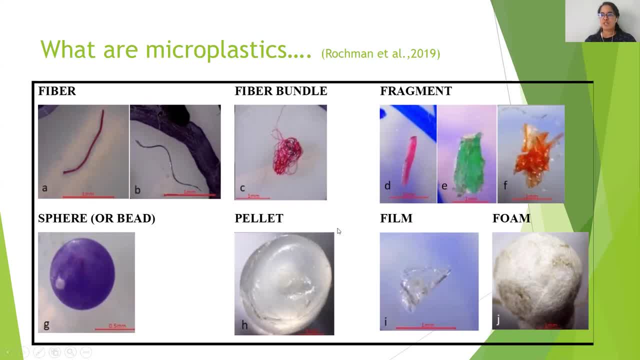 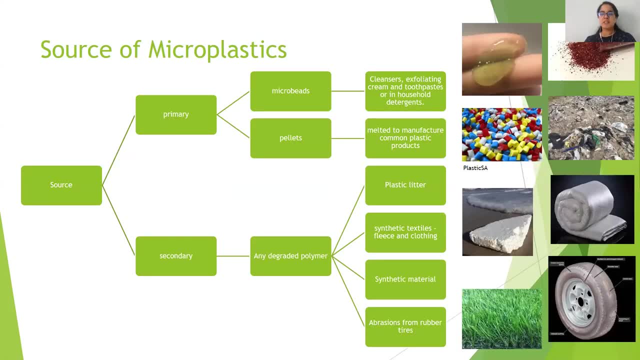 identify where specific shapes come from or what type of plastics is broken down from um. but then if you go further into microplastics um, you will pick up that there are two sources. so you've got your primary source of microplastic and you've got your secondary source, which is the 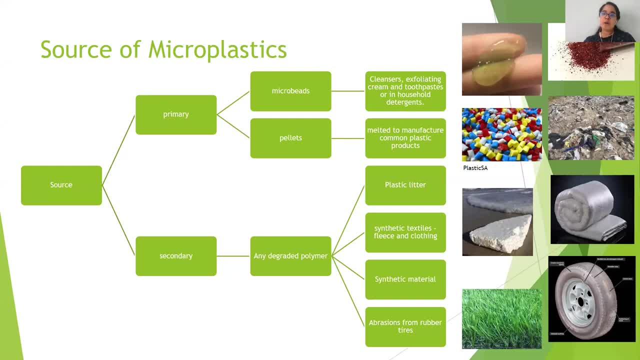 source of microplastics. So your primary source of microplastics is any plastic that is made with the intention to be really, really tiny, And I've got two images there of you'll see over here. it's like some gel with very small polyethylene microbeads in them. That is. 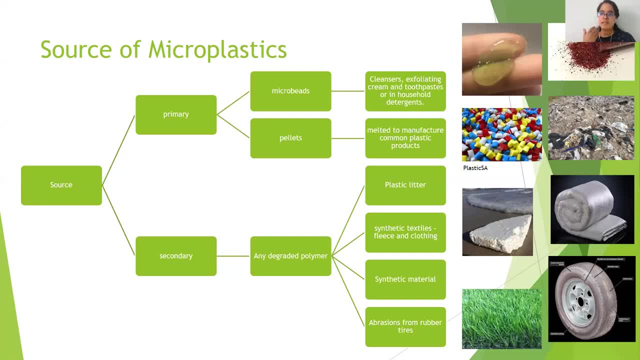 you'll find them in face washers, exfoliating scrubs. So that's plastic, it's microbeads that they add in your cosmetics, And it's made in that form. it's made to be small. And then you've also. 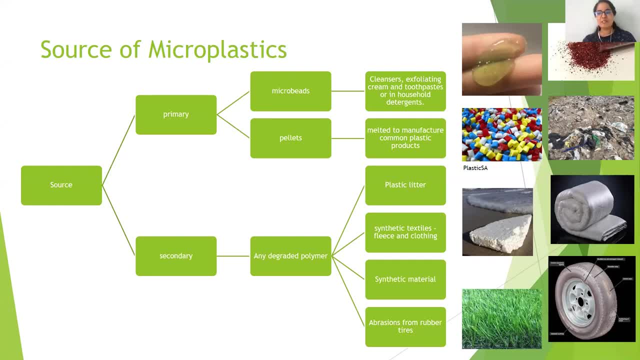 got your glitter, And if you're a parent, you know that glitter sticks for a very long time. it's not fun. So glitter is made in its micro form as well. And then you've got your microbeads, And then you've got pellets. So pellets are made. they make it small. I showed you a round. 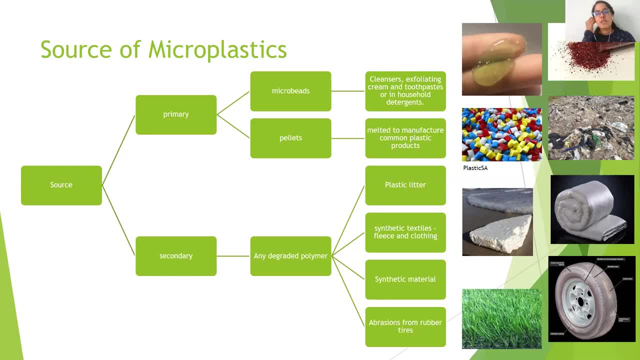 pellet. and then you've got your cylinder pellets. They use that and they melt it to manufacture other plastic products. And then we've got secondary microplastics. Secondary microplastics are larger plastics. They degrade from larger plastics So they break down from. 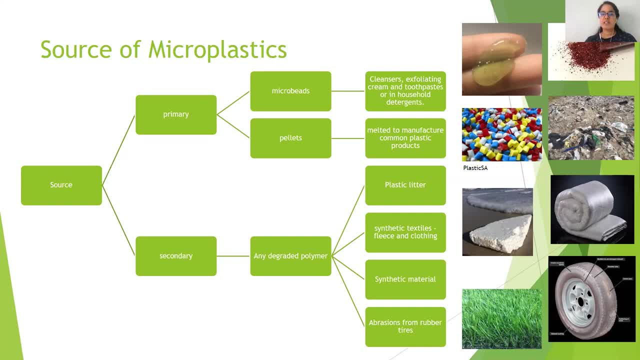 larger plastics, So they degrade from larger plastics. So they degrade from larger plastics. And I've also got examples on the side So you can see plastic litter. You can see synthetic materials, like your synthetic grass. a lot of people are putting in synthetic grass during the drought, And then you've got your rubber from tires. 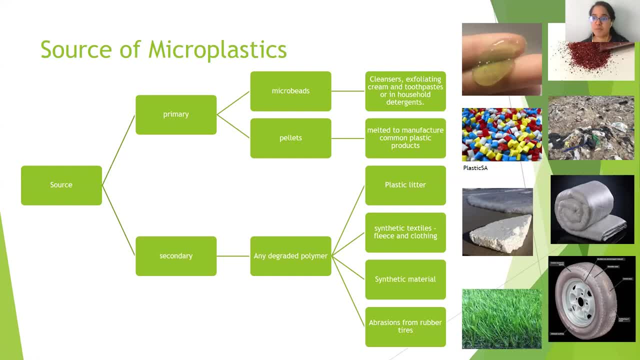 And you've also got synthetic fibers, which we've seen in your clothing items. So a lot of the PET plastic bottles they recycle and they make like micro-fleece jackets, the takeaway micro-fleece jackets, and all of them they made from recycled plastic. 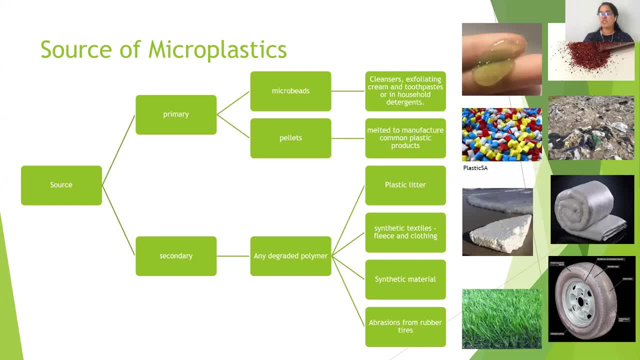 So in your washing machine obviously you now have all your clothing items and, as it's washing, you've got some micro-fibers that are indicated that micro-fibers will break down and be discharged through your washing machine water. Some studies show a study by Brown, ethylene. 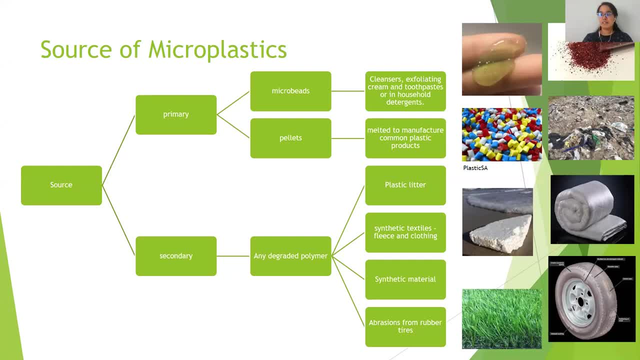 L shows that 1,900 micro-plastics- micro-fibers- can be discharged by one synthetic item in one wash. So that's 1,900 micro-fibers by one item in one wash. Just stop for a moment. think of how many times you do washing. think of how many clothing items is in that washing machine and how many people we have living in the city. 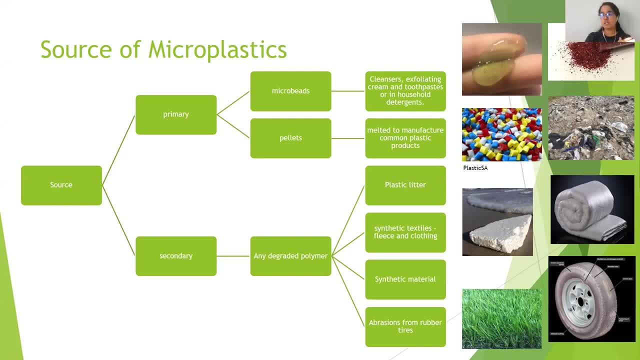 And And. we're all discharging and it all goes to our treatment plants. Again, your micro-beads in your cosmetics. we wash our faces. it discharges to our water treatment plants- The micro-beads. they say you can expect. between 4,500 and 94,000 particles can be released during a single use. 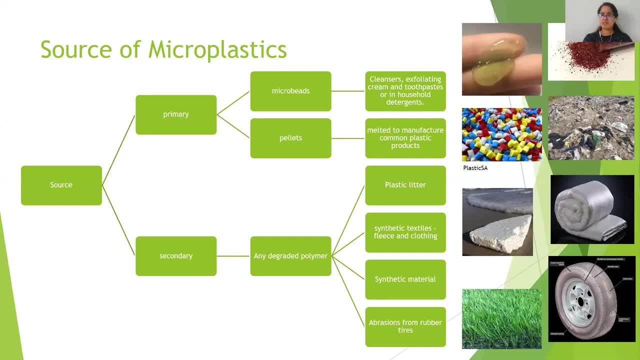 Of cosmetic products. So there's this- quite a lot of micro-fiber beads in there. And then, if you look at this diagram, we're looking at sources and we're looking at types of plastics, Which kind of also tells me where it's coming from. So if I'm finding a lot of micro-fibers, I kind of start to think. 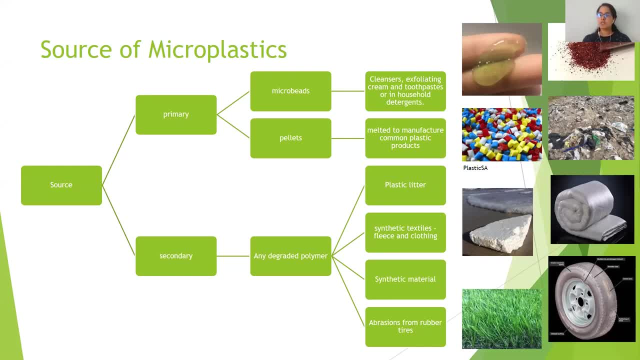 Okay, this seems to be might be more treated water or discharge coming from a treatment plant. If I'm seeing a lot of particles- fine rubber particles, maybe it's coming from stormwater runoff because of roads and so forth. So it kind of gives me some idea of the distribution pathways. 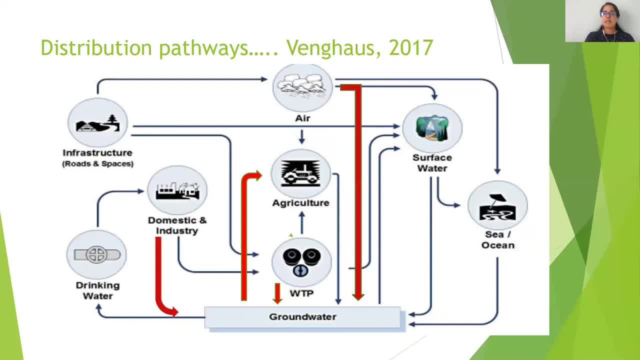 So, looking at a study, another study, This diagram is taken from the study but I've added a few extra arrows in, So we know that there could be potential distribution pathways from the atmosphere directly to groundwater. There's also groundwater if there's microplastics in the groundwater and we're using it for agriculture. 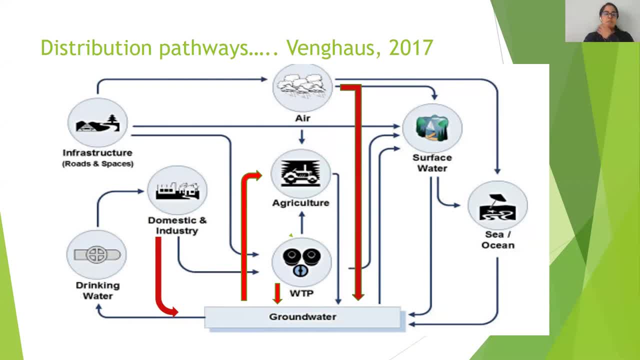 So there's a direct source. The diagram also excludes direct links between your domestic industry and groundwater. And then the diagram also excludes a direct link between your water treatment plant and groundwater. We know what the drought And it's been. I mean, it's been a practice for years already. 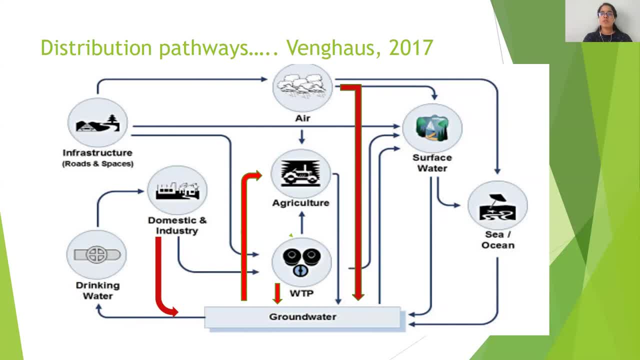 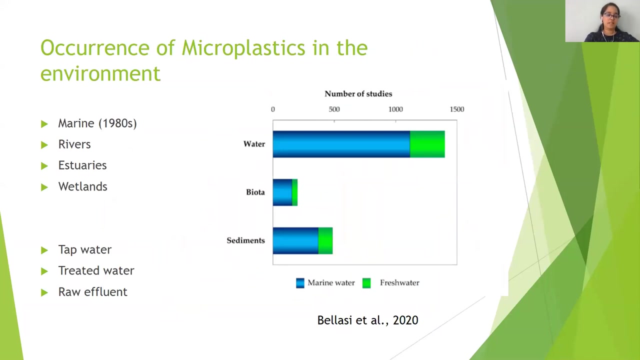 But what was the scarcity? We're now seeing a lot of drought, lot of municipalities moving into managed aquifer recharge, either with treated wastewater or with storm water. so we've added those links in as well. so just looking at occurrence of microplastic i, 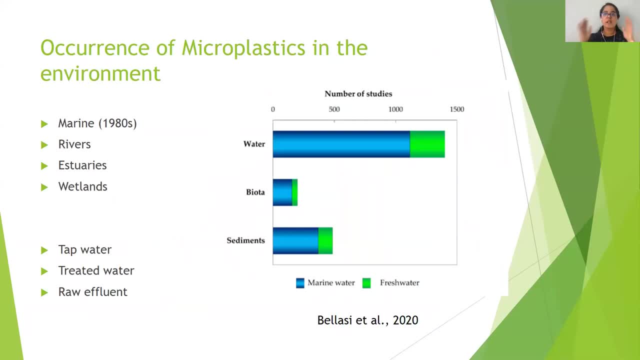 won't go into a lot of detail but studies have come about four years now in the marine environment. so some of the first studies where the term microplastics was introduced in around the 1980s by peter ryan and his team they work on on. 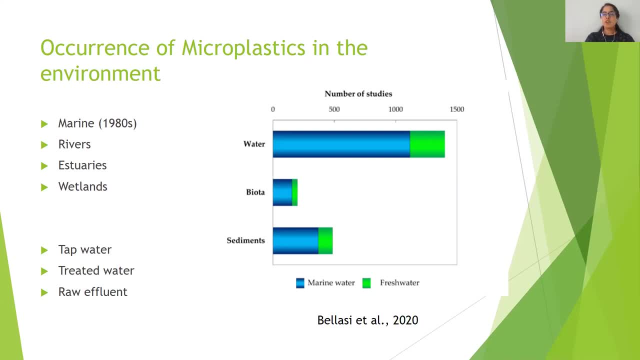 in the marine environment and so you can see there are quite a lot of studies that's been done in water, in the marine environment, and then more, more, so we start to pick up on, uh, freshwater environments. so we've seen all around the world they've done microplastic. 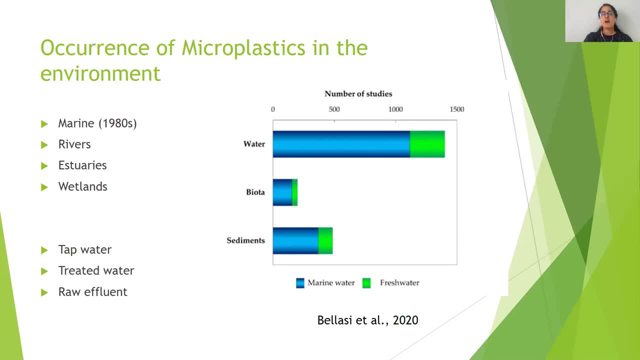 sampling in rivers, estuaries, wetlands, um, with um evidence to show that it's present in these freshwater environments, um. and then i've also added in: they've done sampling of tap water around the world, um and and they found microplastics in the tap water around the. 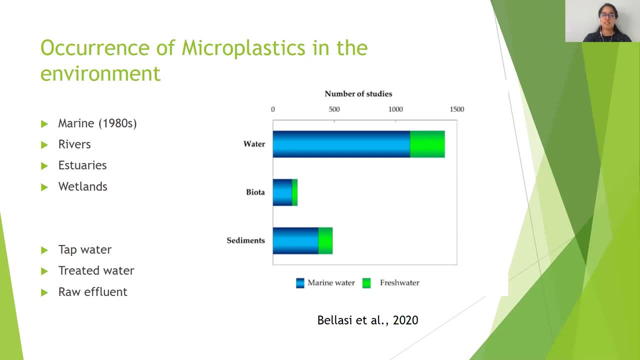 world treated water there's microplastics, and the raw effluent we know there's microplastics, um so, uh, but what about groundwater? so the study is about groundwater, um, um. so the literature that i found on groundwater, i could only find two articles, um, and so that's a little red line that i've added in. that's not the scale. 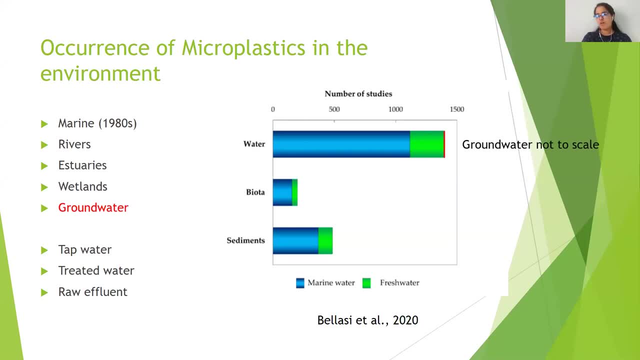 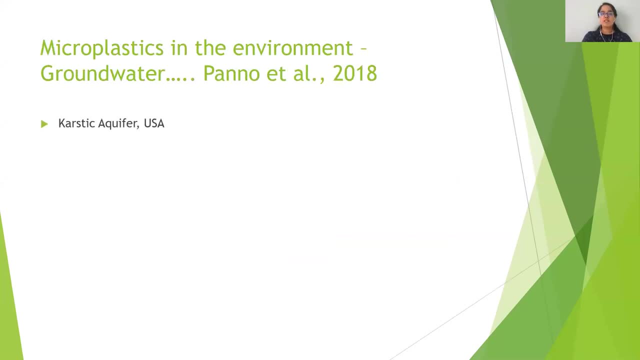 but it's. it just shows that there's very little information on groundwater and microplastics. so the two studies- the one done on a caustic aquifer, in fact both of them- and the one is in uh, the usa, um, of the 17 sites that they sample, they found microplastics in 16. 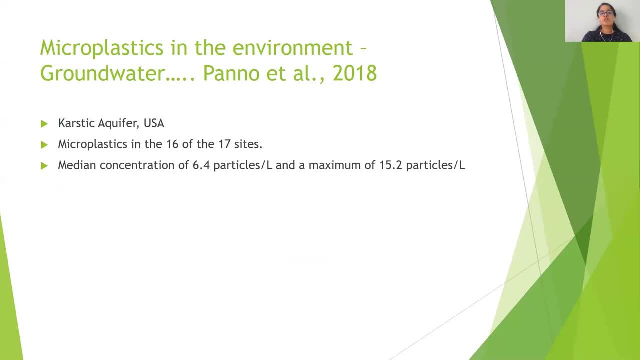 of them um, with concentrations. the mean concentration is 6.4 particles per liter um and the maximum of 15.2 particles per liter. i should mention that the the with the studies there's often people that knows standardized protocol on how to do it. it's a new thing so a lot of the studies will report. 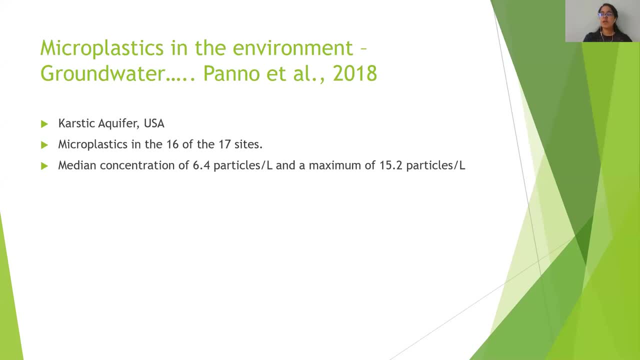 in an area and then others will report particles per liter. so it's difficult to to do a comparison between the studies because their units are not the same. and then we've got. they found that microfibers in the study was small than um 1.5 millimeters. they identified four of the samples as being polyethylene and the rest 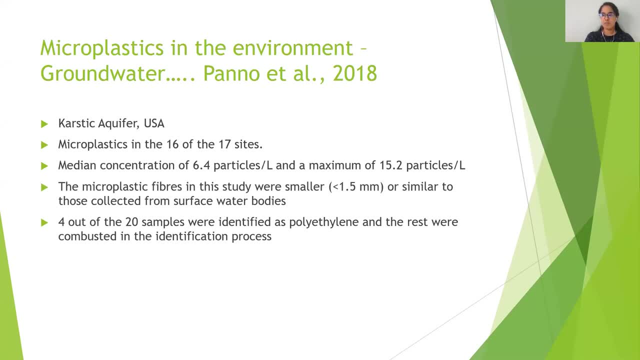 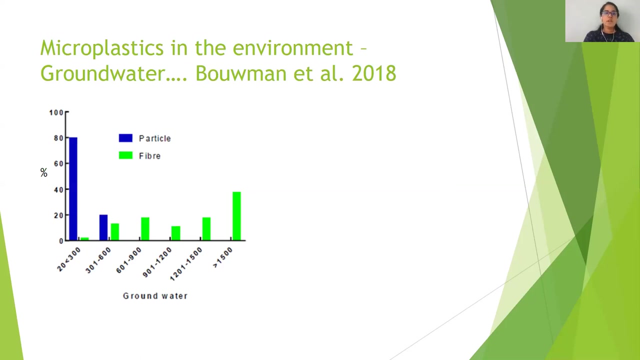 were basically destroyed during the identification process. and then this study also highlighted that fractured aquifers are also vulnerable to microplastic contamination. and then we've got a local study done by um wrc in portugal. it's a wrc study, sorry, done in portugal, where they sampled four balls. 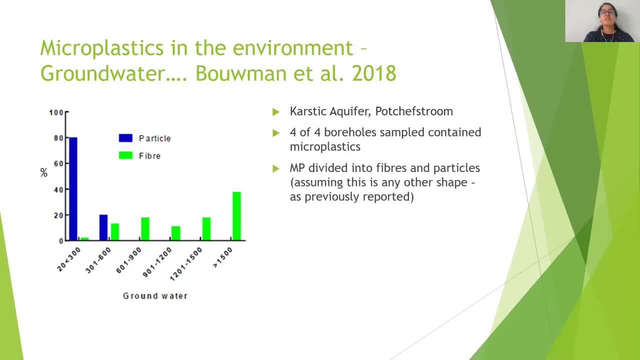 and they found microplastics um. they divided it into particles and fibers, um and i two particles is any of the other fragments and um pellets and so forth. um they found that with the particles um 80 of the particles in the groundwater were between 0.02 and 0.3 millimeters and 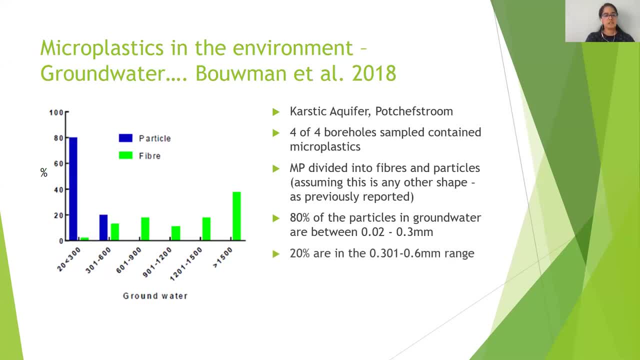 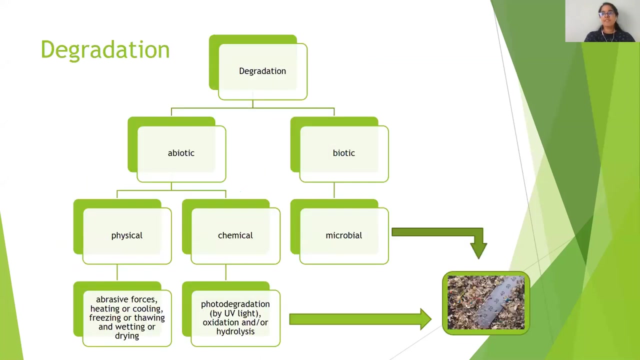 then 20% is is slightly higher. you can see from the graph, we as the fibers. they appear across all size ranges and of the, with the maximum above greater than 1.5 millimeters. so now we know that the they found microplastics in groundwater. so 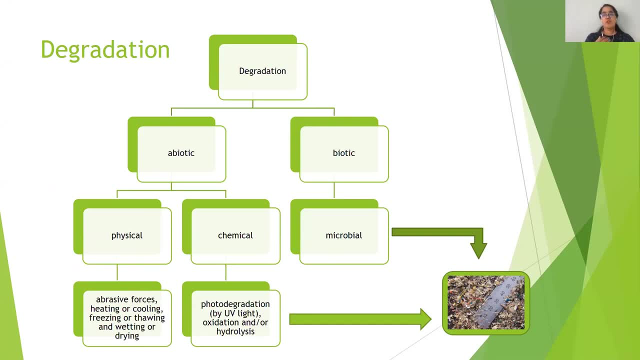 now that kind of gave me some motivation to go further and research a little bit more. so I look at degradation. so you've got your plastic, your bigger plastics. how do they become microplastics? so we've got degradation and the degradation process. the degradation process is split into two processes, so we've got a biotic. 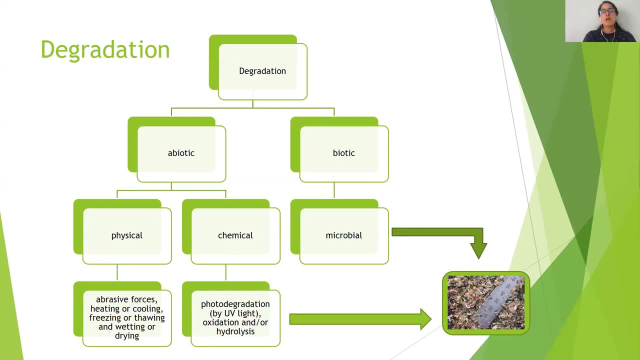 processes and these biotic processes a biotic processes are divided into physical and chemical processes, and the physical and chemical. the physical processes are indicated. you've got the rates of forces, you've got your heating and cooling that can cause particles to break down: freezing, thawing, wetting and 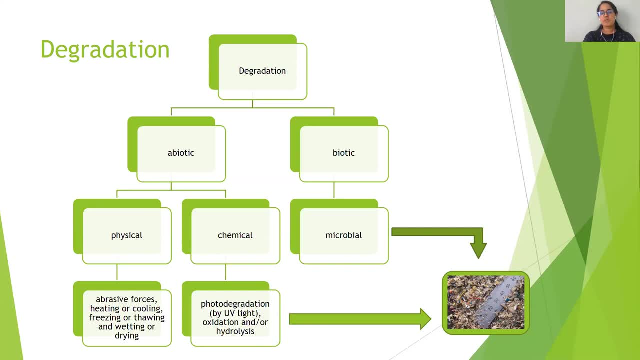 drying as well, and then with the chemical processes you've got photo degradation by UV light oxidation and or I draw the scissors. and then you also got your biotic processes, which which relies on microbials to break down the plastics. now some plastics have additives in and makes make them kind of resistant to to. 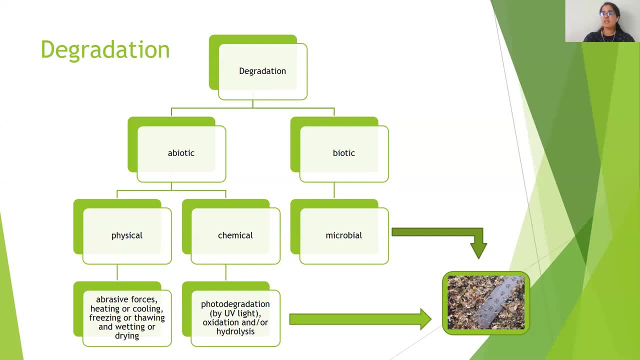 oxidation and so forth, and and and. then it makes them stronger. they don't break down. however, if you look at the degradation processes, the- the biotic process- in some instance rely on the abiotic process first. so it would go through the whole abiotic process and it would break down into smaller pieces and 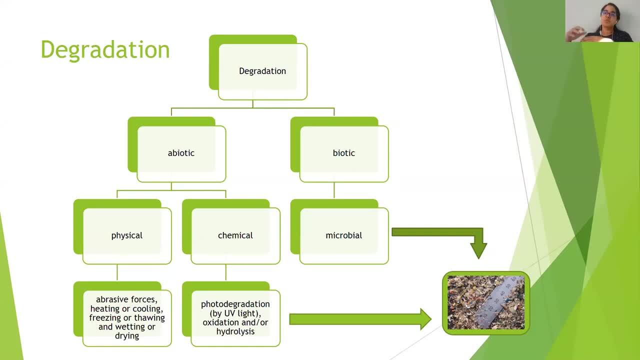 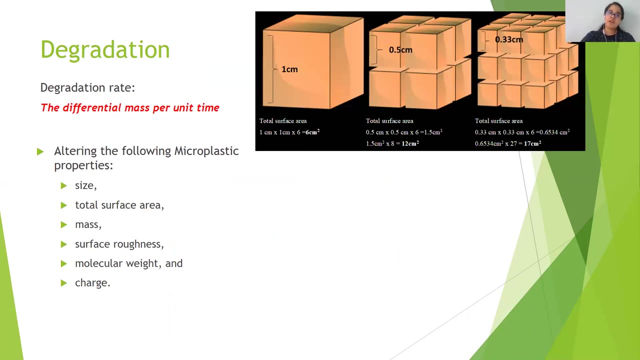 then it becomes available for microbes to degrade even further. but in some instances it's not even available for microbes to degrade because of the composition of it. so we look at degradation further and studies have showed that the degradation rate is the, the difference, the differential math per unit time. 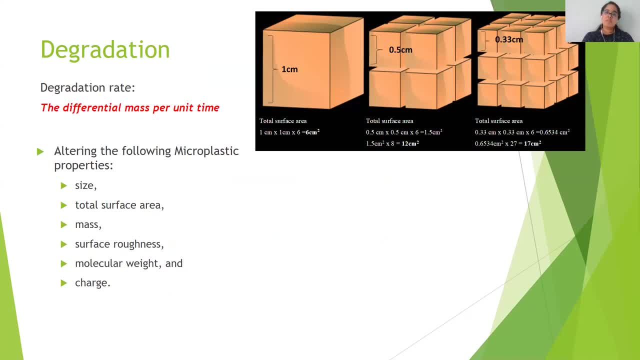 so that's how they determine degradation rate, degradation. so what does it do to the plastic? it alters the size. it alters the total surface area, the mass, the surface roughness, the molecular weight and the charge of that plastic. so the diagram just shows a total surface area. an example of total surface area. 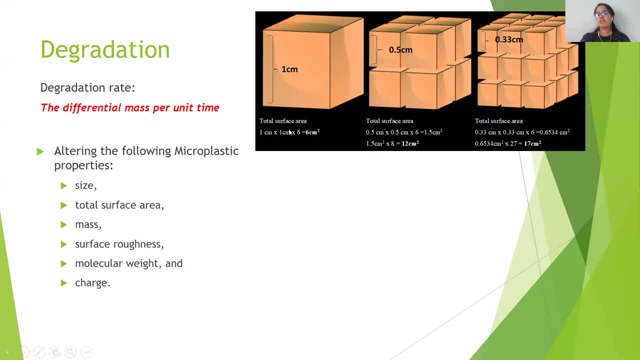 so if we have a particle that's one centimeter by one centimeter, the total surface area is one centimeter. the total surface area is six centimeters squared. however, if this particle now breaks down, degrades into smaller particles of 0.5 centimeters. the total surface area of that. 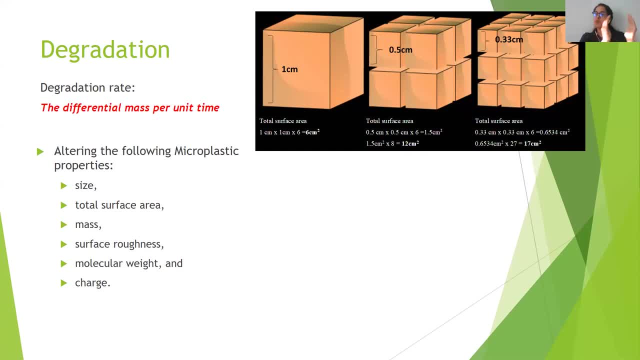 whole particle, of all the particles that now made up that. one particle is 12 centimeters squared, but if you break it down further um, the total surface area becomes 17 centimeters squared. so we can see that the volume remains the same, but the total surface area increases. now why is this important? 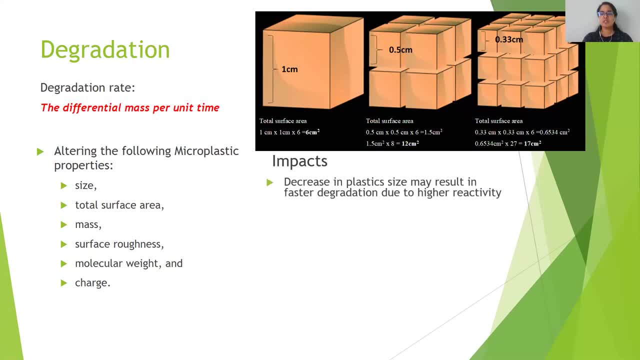 so the impact of degradation. according to studies have showed that the decrease, the decrease in the plastic size will result in faster degradation due to higher reactivities. um it also, as it degrades, it releases ketone groups and ester groups, which are additives in the plastics, and then it alters the surface roughness and it changes the charge of that. 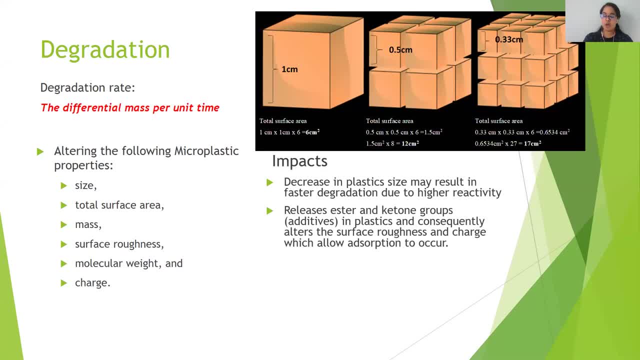 particle which now allows absorption to occur. it changes the molecular weight of a polymer, so it's technically modified from a polymer to a oligomer, to a monomer, so it's now no longer a polymer. so what are we working with um and then um? studies indicate that in some environments the degradation 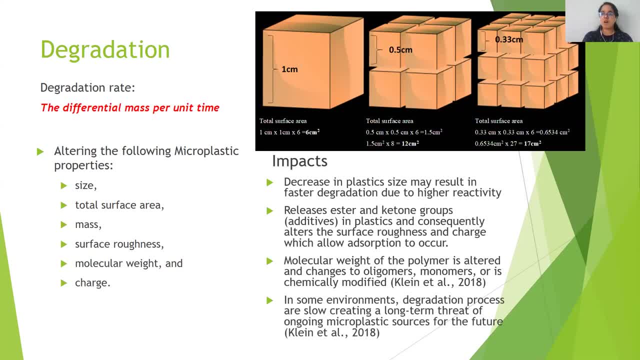 process is really slow. so if it's slow, it means that there is a constant source of microplastics, so it's a long-term threat to the environment. so it's there and it's slowly degrading, but it's continuously providing that source of microplastics to wherever. 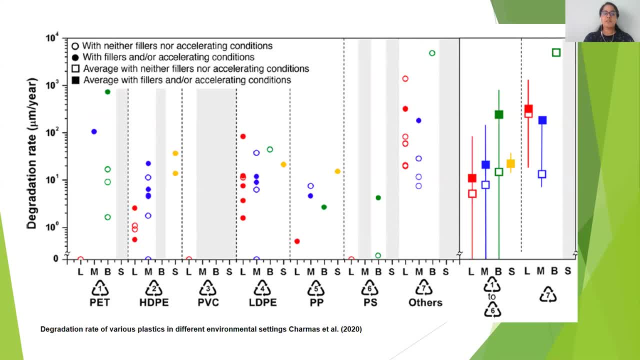 so this is just an example of different types of plastics. we can see p-e-t-h-d-p-e-p-v-c? um and then the different colors indicate different environments. so l? um represents landfills and compost soils. m? is the marine environment, b is the biological environment. s is in sunlight, so we can. 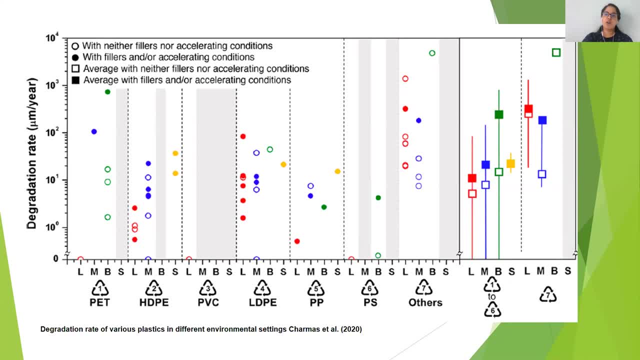 see with fillers, without fillers. they are different, different ground roots, they are different planet Biomes. so in the lab we can see marine life. participation is that different places, an environment is different depending on the seed and also it depends on the origin of the plant. we can measure the 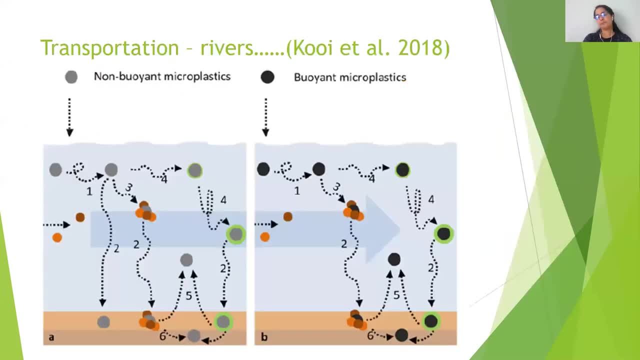 etz energy source of different monomer kinds, and how it's operating and how it can also affect proximity of environment, such as soil organizationways. so now we have been looking at different plants, as I've interested in different types of plastics, so we're looking at something that's really complex and changes really. the change is: 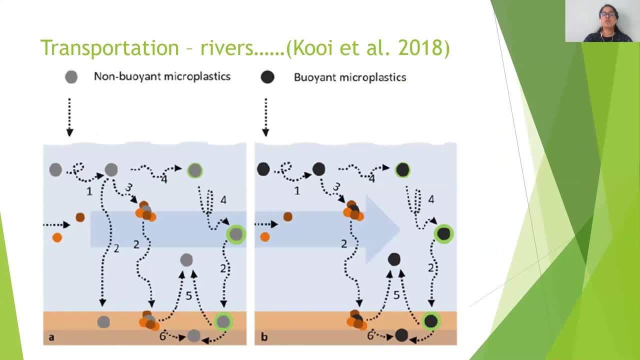 very sensitive to environments and and types plastics. So now that we know degradation, we know how the particle was formed or processes that could form transportation, And so I found transportation processes- this is just an example of transportation processes in rivers. So you've got your dense and your less dense, which would make it buoyant, or 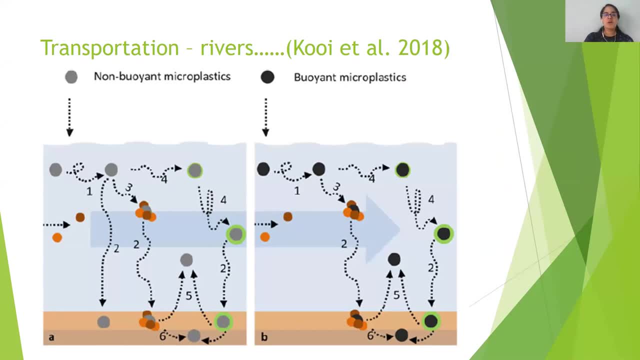 non-buoyant particles. So your non-buoyant particles, it comes into the river and it can settle immediately. So you've got number one, which refers to your turbulent transport. You've got number two, which refers to settling. You've got number three, which refers to your 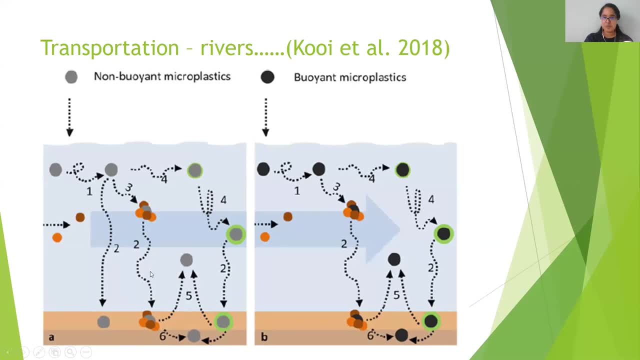 aggregation process, And then number two again, because now, even if you can settle further, you've got number four, biofouling, also leading to settling, And then you've got five, which is resuspension, and you've got six, which is burial, So it can be embedded into the 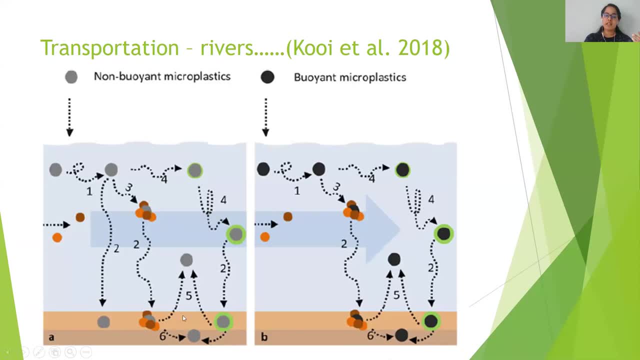 sands in the river systems, But again it can resurface, basically, and then undergo that process again. Sorry, that's non-buoyant. and then you've got your buoyant ones. So you've got your turbulent process, but obviously it's buoyant. 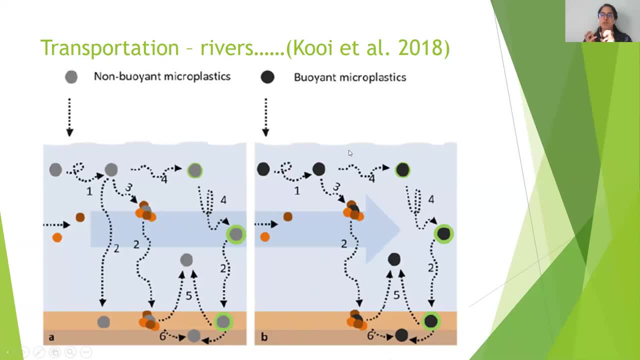 So it's not going to settle, So it needs other particles to attach to it to make it heavier, and then it settles down, And then you've got biofouling as well, And then you've got your burial and you've got your resuspension again. But also noting that these are obviously 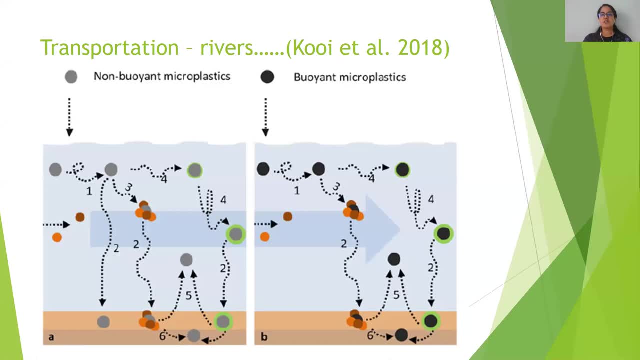 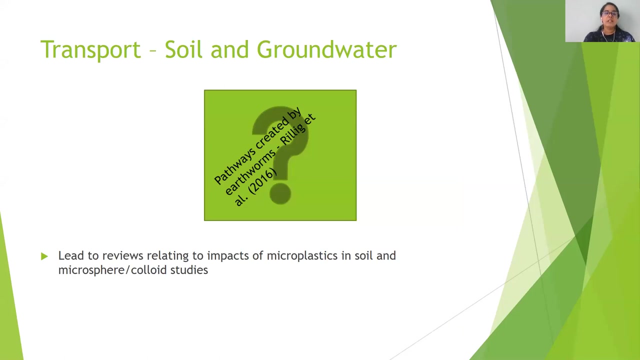 flowing rivers, but you've got rivers that dry up in some seasons, So as the level lowers in your river, you're obviously going to have settling of those microplastic particles into the beds of the rivers. Okay, so now we look at transporting groundwater And basically I couldn't find anything about. 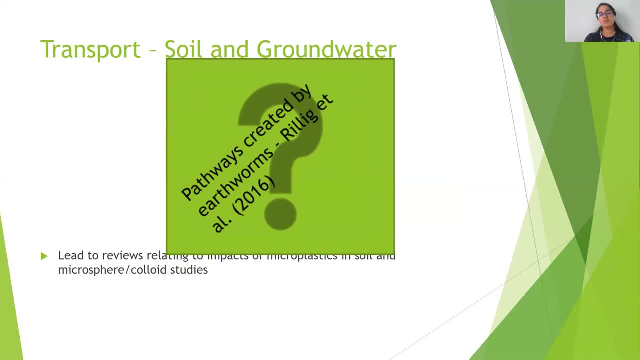 transporting groundwater. I did find an article that refers to earthworms creating preferential pathways and the microplastics could attach to the earthworm and the earthworm basically takes it lower down in the soil horizon. That's all I could find, And so it led to further studies. 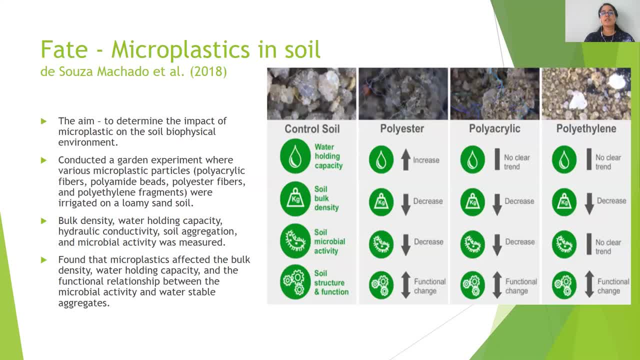 And it led to the study where he did an experiment. they did an experiment on the fate microplastics in soils. so the aim of the study to determine if there was an impact of microplastics on the biophysical properties of the soil. and so what they did was they conducted like a garden. 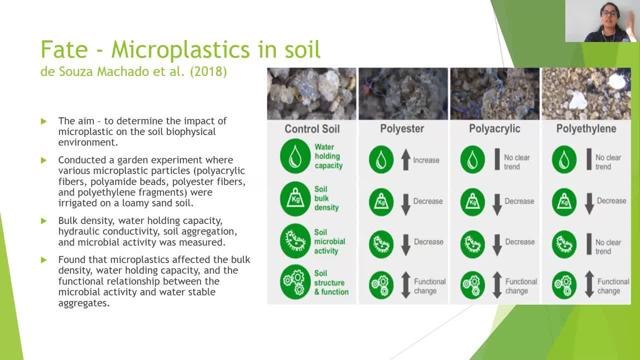 irrigation experiment and irrigated with water mixed with polyacrylic fibers and beads and polyester fibers, polyethylene fragments, but this was for a loamy sand soil and then they measured certain properties and they found that the bulk density was affected and the water holding capacity was affected. the functional relationship between the microbial. 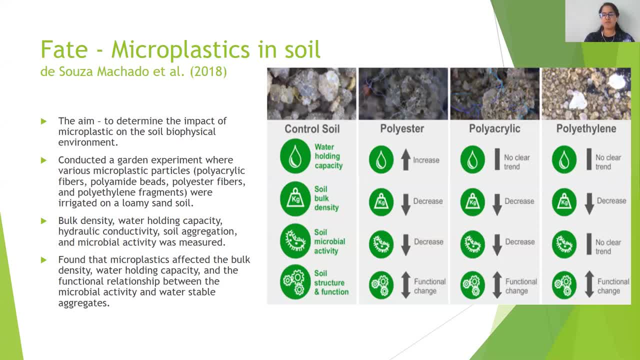 activity and water stable aggregates were were affected. they did not see any change in hydraulic conductivity. but the study highlights that again, they used specific types of plastics, specific sizes in a specific soil. so this it doesn't imply that irrigation of a source with microplastics will not have a change on hydraulic conductivity. it's just in this specific 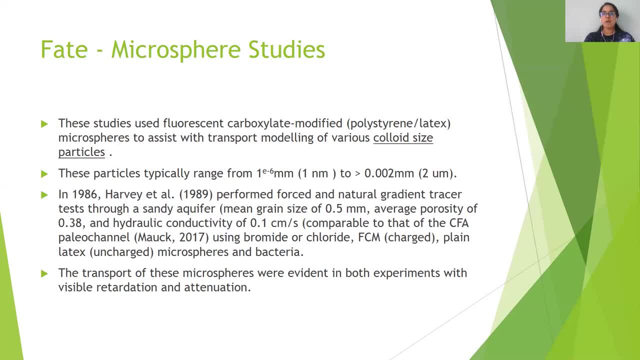 environment. so it leads to microsphere studies. so we know that microplastics are small particles. we know the sizes, so we look at studies, colloidal studies or microsphere studies in groundwater, which are particles more in the lower range of microplastics to nanoplastics, and so there's been studies over the 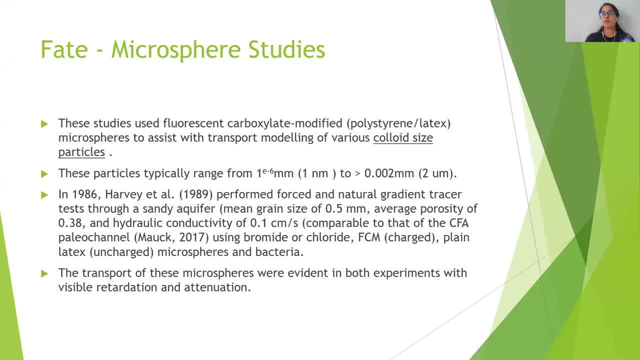 past few years where they used a fluorescent carboxylic modified microsphere which is polystyrene or latex latex beads and they use these as traces in in in groundwater experiments to determine the transport model of bacteria. so they use the tracer with the bacteria with another tracer. 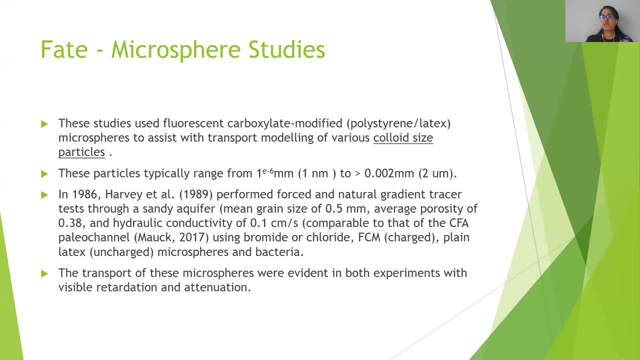 to capture the soil and they use that to to see if that specific microsphere could be used as as a substitute or tracer to which would resemble bacteria in in groundwater. and so the study in 1986. they performed a forced and natural gradient tracer texts using these microspheres. 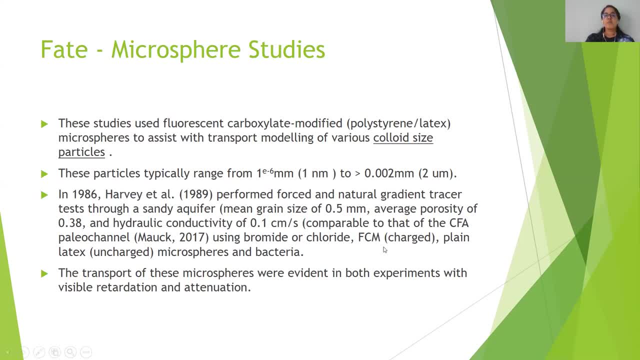 as well as bromide and chloride. the microspheres were uncharged and some of them were negatively charged as well, and they found that the microspheres were moving in in in the aquifer and there was visible retardation and attenuation as well, and the the the other. 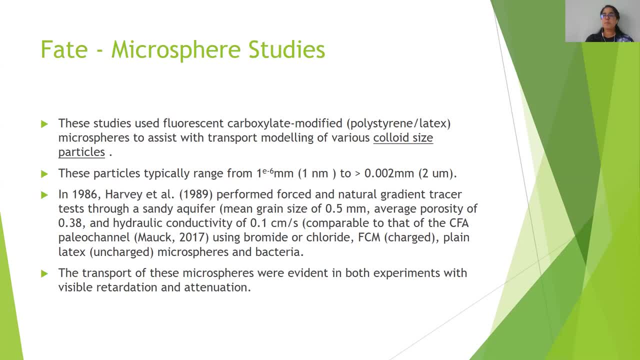 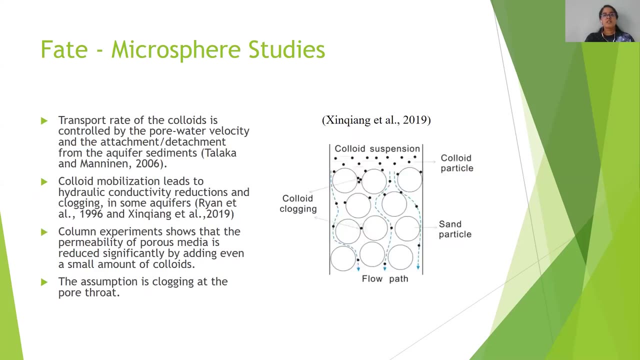 places, the bromide and chloride, um their peaks, came through faster, like several nine, nine, eight to nine days faster um than the microspheres. uh, the bacteria also came through faster than the microspheres. so we went further into microspheres because it seems as though there's some resemblance between the 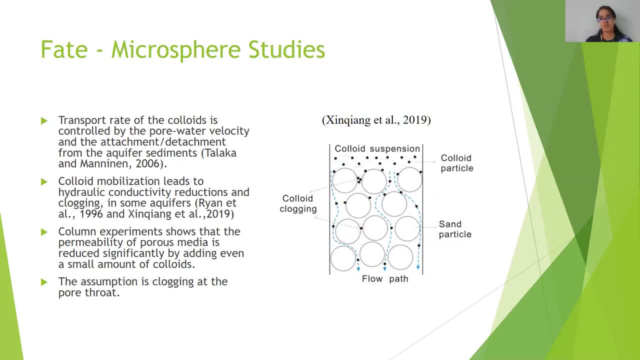 microplastic that they use, between microplastics and the microsphere that they use, went further into these studies and we found that the transport of these microspheres was controlled by the water, the poor water velocity and the attachment was detachment to the aquifer sediments. 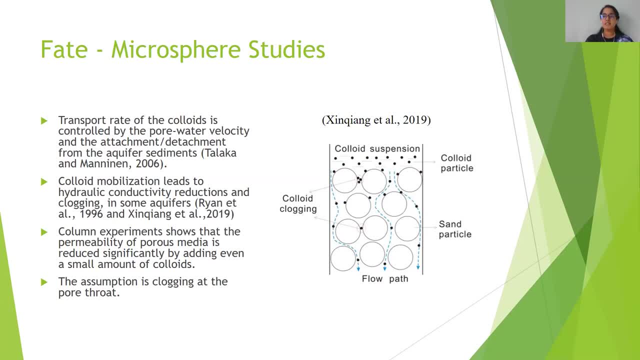 it led to in some of the studies. they did column experiments and they found that there was a decrease in in hydraulic conductivity when they injected these microspheres um into the, into the, into the columns um and then the. the column experiment also showed the fact. the permeability of the porous media is reduced significantly when they 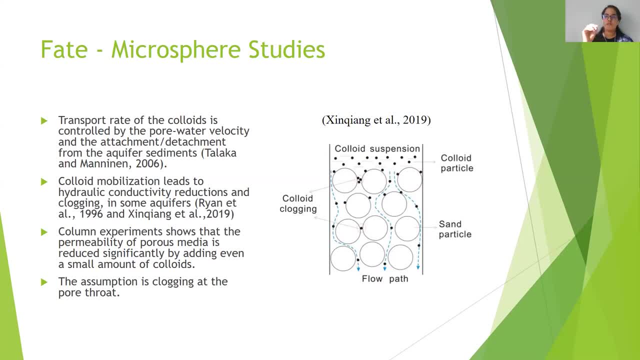 just add like even the smallest amount of of these microspheres into the into the the experiment. they immediately noticed a change, um, and so they assumed that if it was because of um clogging at the poor throat. so this is just an image of the, the microsphere that was used. 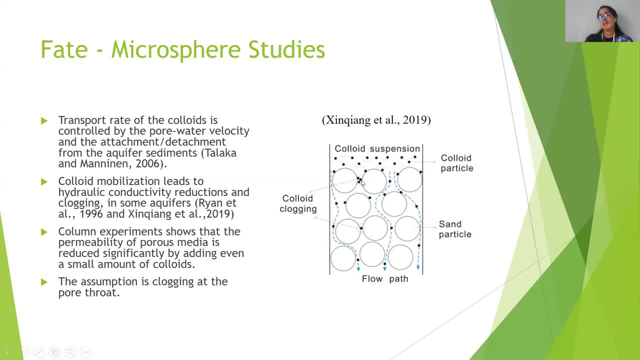 and they. there's an assumption that at the poor throat the colloid will kind of clog that core and then reduce that flow, and so, um, it's also the. the clogging i mean in in these studies is also referred to as straining in an aquifer. 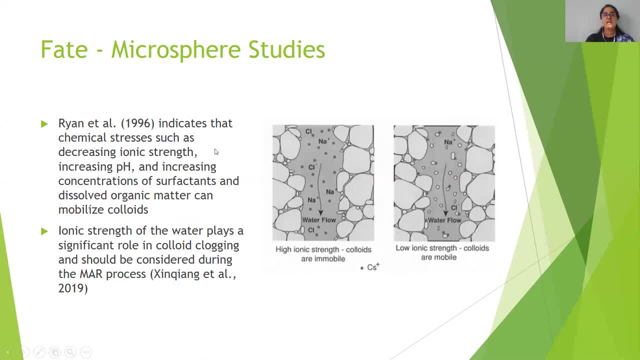 um, and then we looked at different chemical stresses, um, what could change or impact the movement of these microspheres, and it was found that if there's a decrease in the ionic strength of the water, then there is mobilization, so um, and then there's also with an, 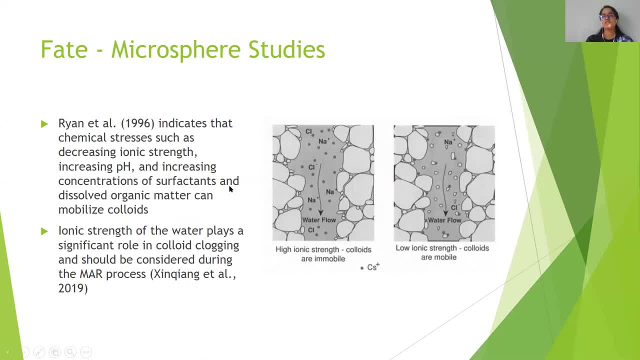 increase in in the ph uh, increasing concentration of surfactants and dissolved organic matter- all of these can mobilize the microsphere. um that the ionic strength plays a role in the clogging as well, so, um, it is something that must be considered um when you are doing managed aquifer recharge. 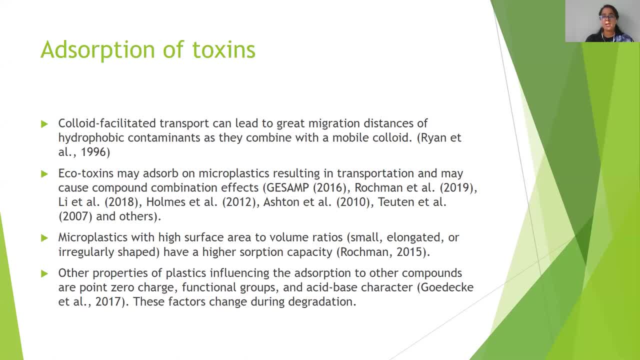 so we get to one of the other questions: um, we have some hydrophobic toxins, um, and we are going to go back to the previous slide. in the next slide, we are going to go back to the previous slide. in the next slide, we are going to go back to the previous slide of the. 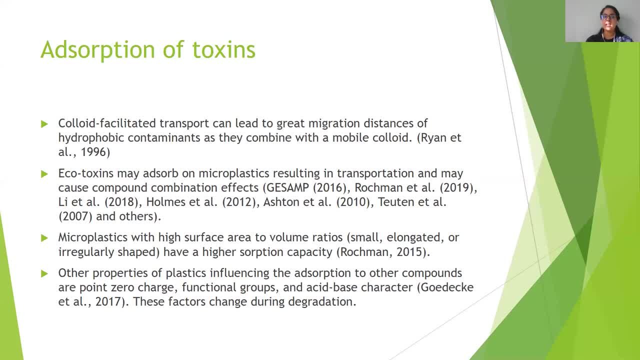 and they don't travel, they stay there. However, we are now thinking that if microplastics do have the ability to move in an aquifer, will it absorb and allow that toxin to move as well. So we found that colloid facilitated transport. 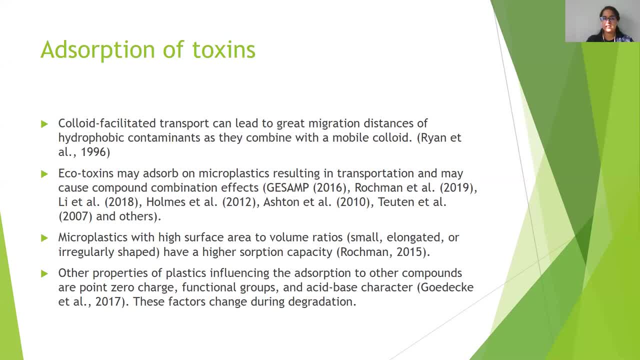 can lead to great migration distances of hydrophobic contaminants. So we know that these microspheres contaminants do absorb to the microsphere and it moves it. And then further studies on microplastics itself found that ecotoxins also may absorb to the microplastic. 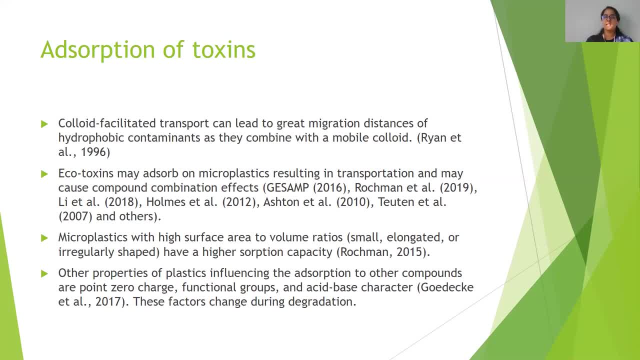 and resulting in transportation. That is the first thing we found, Specifically in the marine and surface open fresh water environments. The microplastics with a higher surface area ratio, higher surface area to volume ratio, have a higher absorption capacity. So I showed you the diagram where you have a particle. 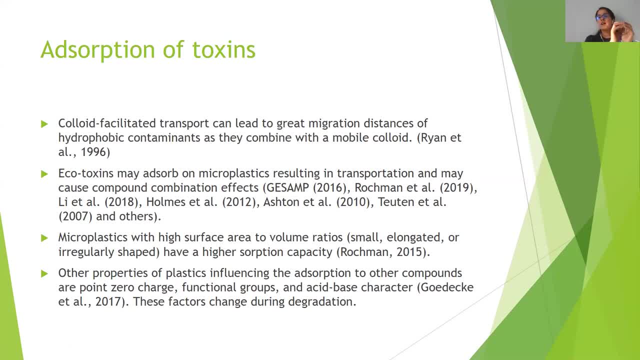 of one centimeter surface area. but if that particle break down the surface area becomes bigger. and the more it breaks down the bigger the surface area becomes. So if it has a bigger surface area there's more areas for the toxin to absorb. to now, 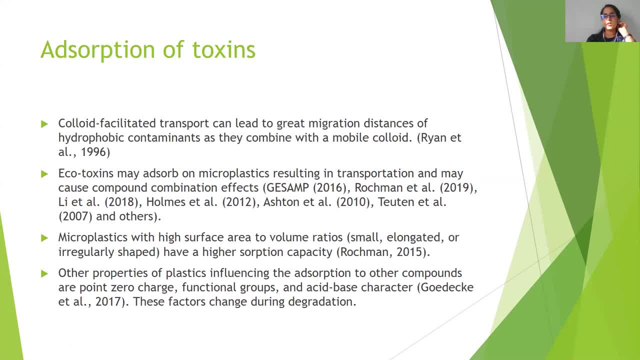 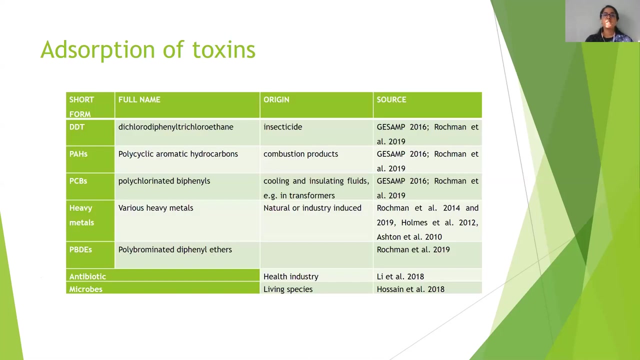 And then other properties of plastics influencing adsorption. So when a particle is, compounds are 0.0, charge, functional groups and acid-base characters. So these factors are all changed in a micro, in a plastic when they degrade, So obviously making it available for adsorption. 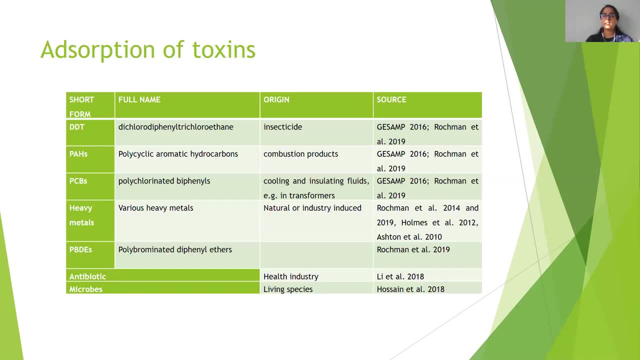 So we looked at different types of toxins and this is taken from various studies. I'm not gonna say these names, They are really big and really complicated to say, but we are all familiar with PCBs, PAHs, We know them. 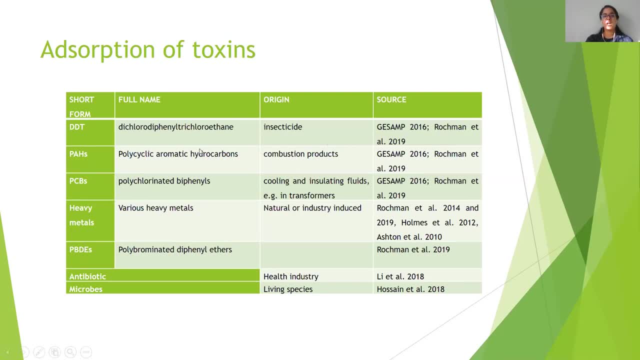 They can absorb to microplastics. And then there's also a study that shows that they can absorb to microplastics. And then we had a study in between where they absorb to microplastics and then it was found that they are. 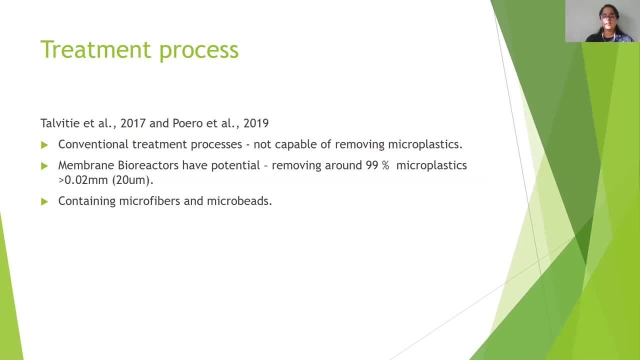 they all absorb to microplastics. And then there's also a study that shows that antibiotics and microbes also absorb to microplastics. So just quickly looking at- I'm not gonna go into treatment processes- microplastics. and then there are a few studies which which show that the membrane bioreactors 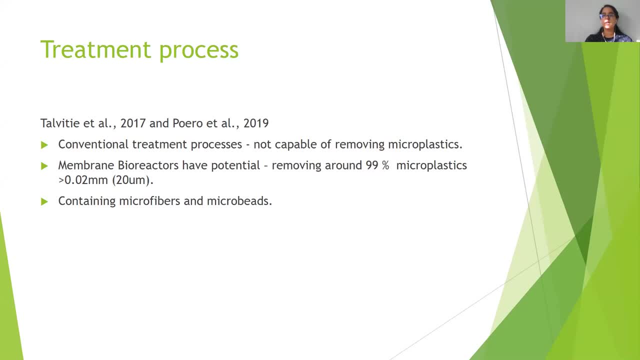 have a potential to remove. a large percentage, like most of the studies, are between 95 and 99 percent of microplastics, but these are all still anything that's greater than 0.02 millimeters, so anything smaller than that there's a potential that it's not going to be removed, so possibly 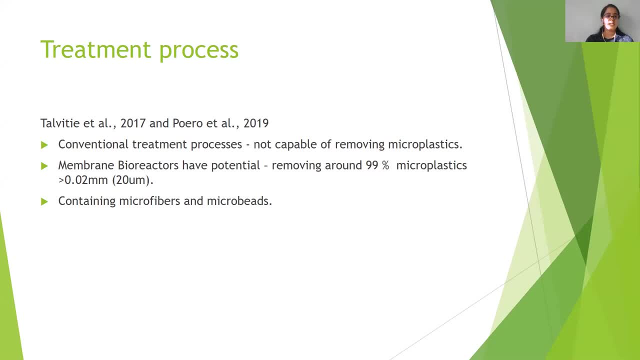 your nanoplastics and then the in the in. in the studies they showed that the common microplastics were microfibers and microbeads and and, as I've indicated, your microfibers are coming from your synthetic clothing items and then your microbeads coming from your cosmetics and also your some of your detergents. 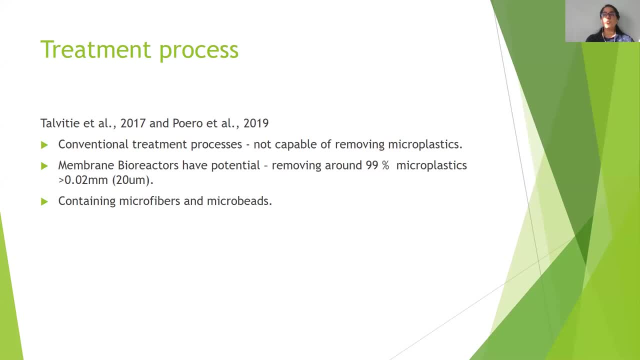 like your dishwasher and your your washing machine pods as well. so, as I've mentioned, what about nanoplastics? it's the bio membrane. bioreactors do not have the potential to remove that and we haven't gone into this yet. and then it also raises question about how do we manage or dispose the sludge coming from. 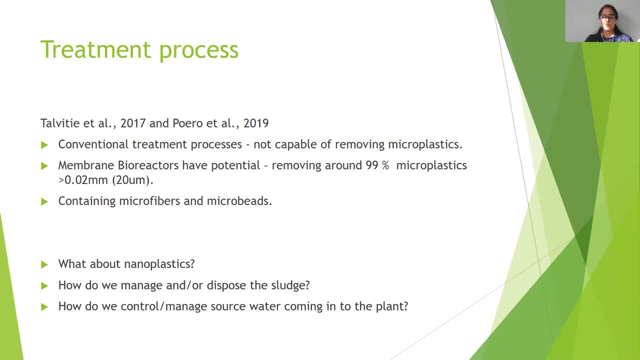 the treatment process. and also another thing to consider is that sludge is now being looked at to reuse as fertilizer in the agricultural area. so definitely we need to consider microplastics, because that can be a direct link to your groundwater. and then how do we control or manage? 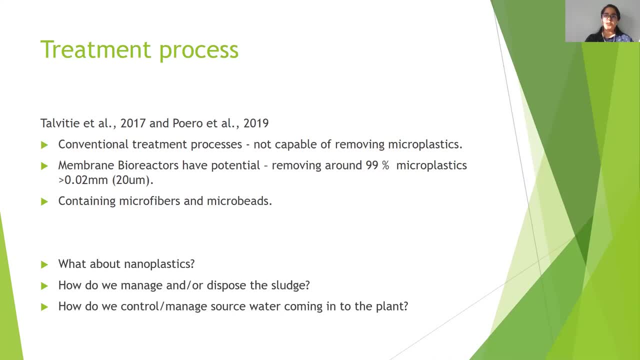 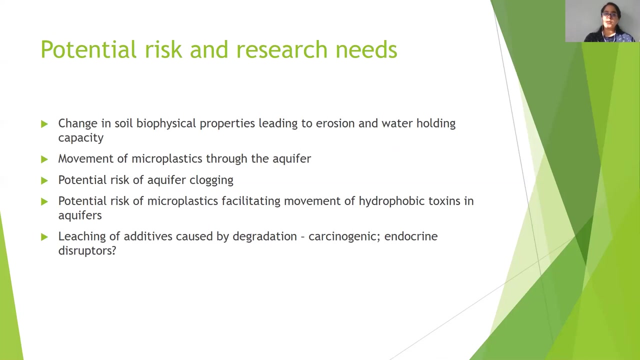 the source of the water coming into the plant. these are some questions that obviously need to be answered, because you've got washing machines, you've got your discharge from your facial products and stuff, so how do you control that coming into the to the treatment plants? We looked at the potential risks and research needs so we know that there's a change in. 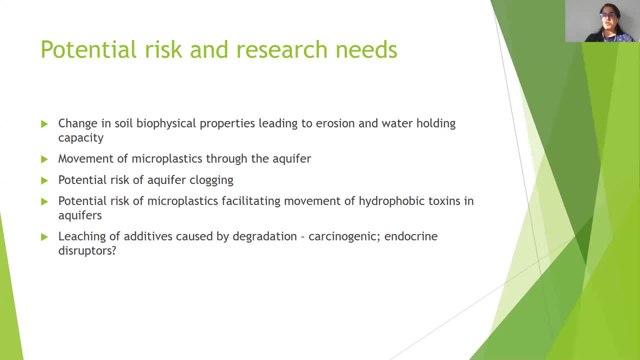 the soil biophysical properties which can lead to erosion or water holding capacity or affect the water holding capacities. Movement of microplastics through the aquifer: that's a potential risk here: Potential clogging of an aquifer and the potential risk of microplastics facilitating 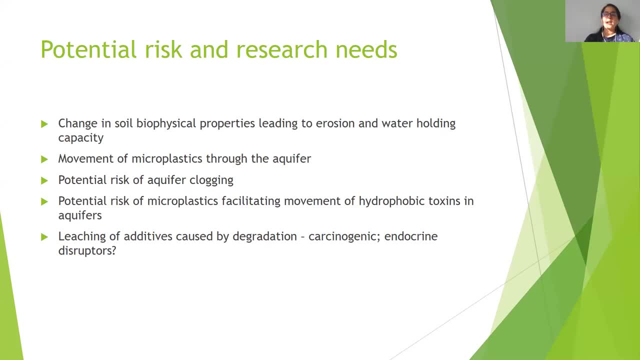 the movement of hydrophobic toxins in an aquifer. And then, as I've indicated to you previously, you have additives, which makes the plastic, you can mold it, you can make it hard, you can make it flame resistant. So these additives, they could leach during dengue. 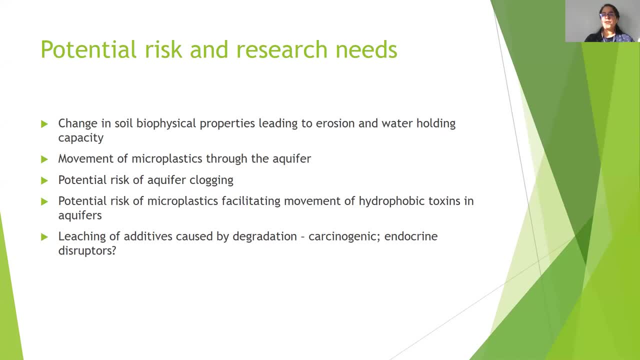 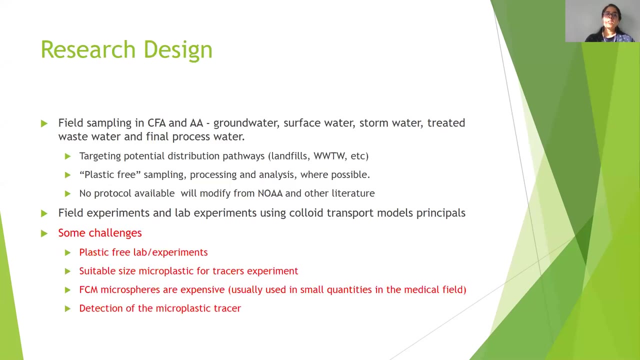 And we've also found that some studies show some of the additives that are used in your PET bottles or so forth are carcinogenic and also they are endocrine disruptors. So the research design, after all of the research literature reviews that we've done, we're 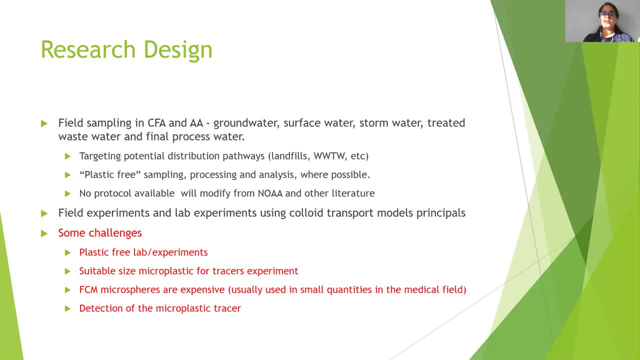 now looking at microplastics As a microsphere And, as we've seen in the microsphere studies, they do move, they do reduce hydraulic conductivity and they do have the ability to clog. So we are going to be doing field sampling in the Cape Flats and the Atlantis Aquifer. 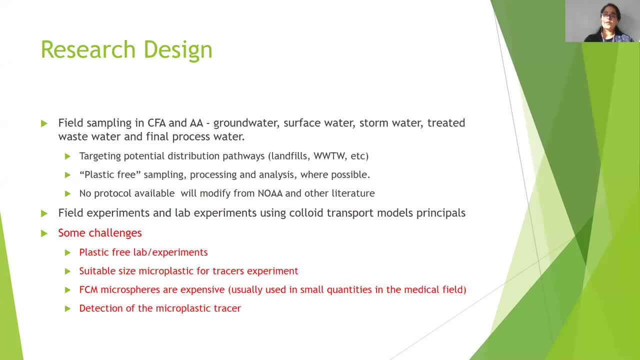 in the Arctic Ocean, Okay, And we are often going to be in this area, but we won't only focus on groundwater, obviously, because the source comes from above. So we'll do groundwater sampling, surface water sampling storm water, treated wastewater. 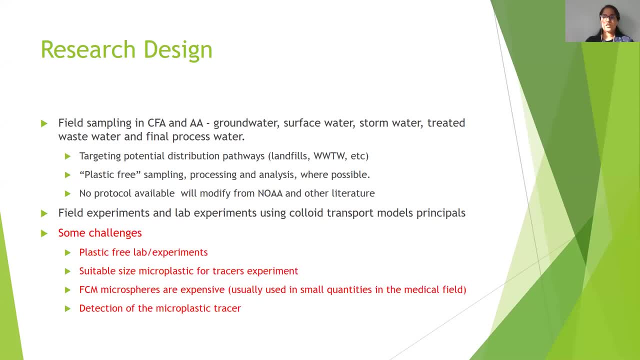 and final process water. We'll target areas that we think would have a higher potential of contributing, like your landfill sites, wastewater treatment, discharge points and so forth. we are looking at a plastic free sampling process and analysis- processing and analysis, which is really really difficult because everything has plastic in. 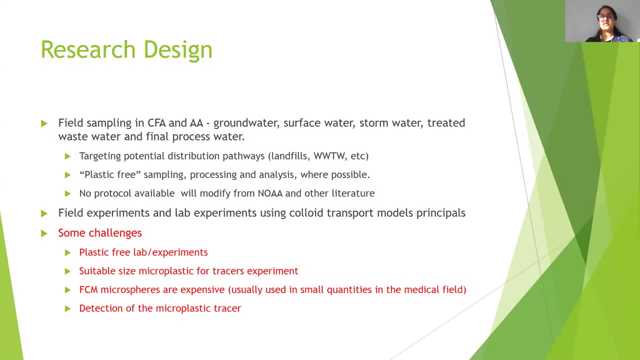 so with the sampling process, you have to look at your equipment. what equipment are you going to use? does it contain plastic? is this plastic that you would think would be in that environment? do I now have to remove that plastic as something that I should also analyze for, because it might? 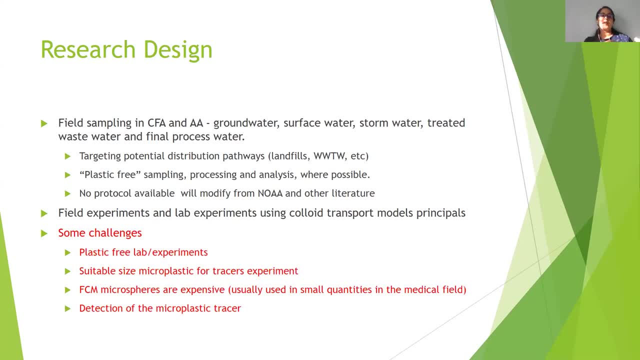 be compromised by the equipment that I'm using. the clothing that you're wearing could have plastic fibers in them, so we are looking at getting pure cotton- PPE, and then there's also no protocol available for groundwater. there is some standard guide that everyone is using, and so we'll use that guide and adapt it. 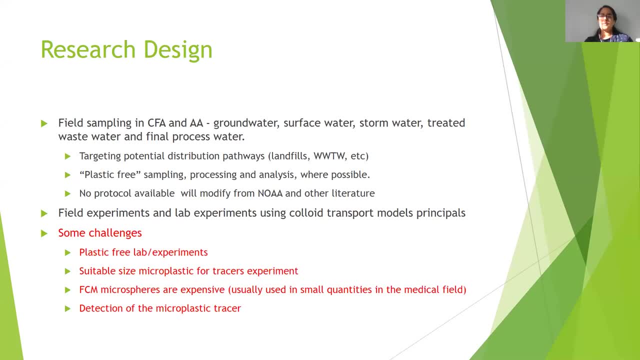 and then also there is a guide for the microsphere studies to sample, but from what I've seen, the equipment contains plastic as well, so again, we can't use that. and then we've got field experiments, and we've got lab experiments, and we'll we'll use the following transport model principle for these lab experiments: 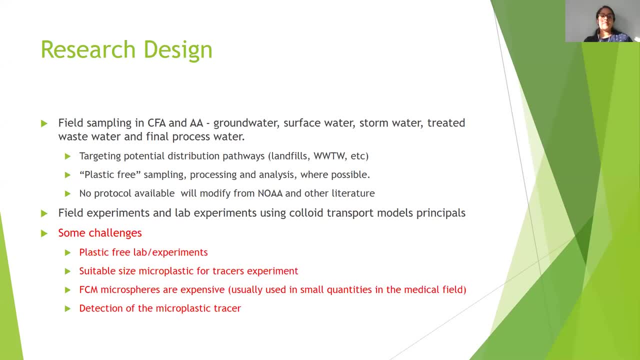 but we'll use microplastics. and then some of the challenges again: a plastic free lab and the and the equipment, and then finding or at least getting a suitable size microplastic that you can use as a tracer. and then, sorry, FCM is the fluorescent carboxylate modified microspheres. they are 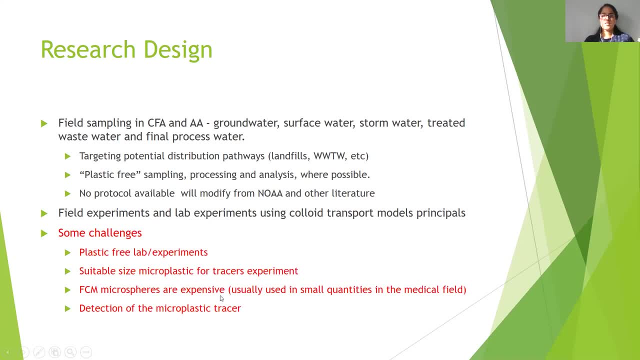 really expensive because their purpose is actually they use it in the medical field, so you need very small concentrations which they would inject into your body to use as a tracer. however, these microspheres have been used in the groundwater environment doing experiments, but they are very expensive. and then how do we detect the microplastic in these experiments or during 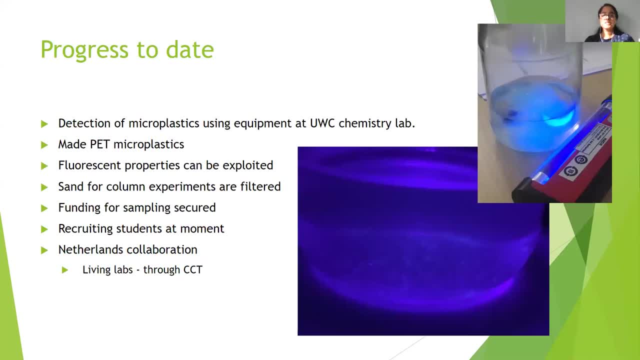 these experiments. so progress to date. um, we are going to be using a lab at UWC to to to analyze the microplastic. but before I talk about how microplastics can cause it to detect microplastics, we've made some microplastics with PET material. 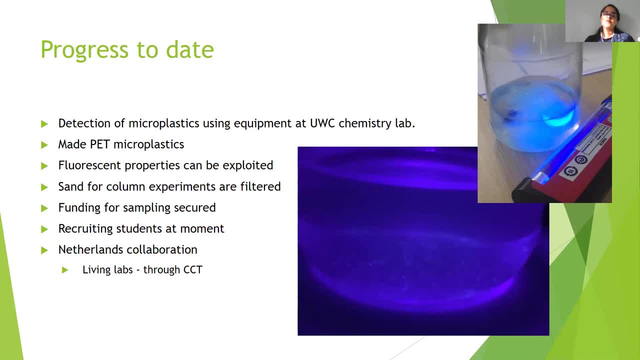 and we also are exploiting the, the fluorescent properties of microplastics. so um you can see in this image um the PET is is quite dense. it's- i think it's got a density of 1.2- definitely sink in water. you can see the, the small fluorescent particles. these are some of the. 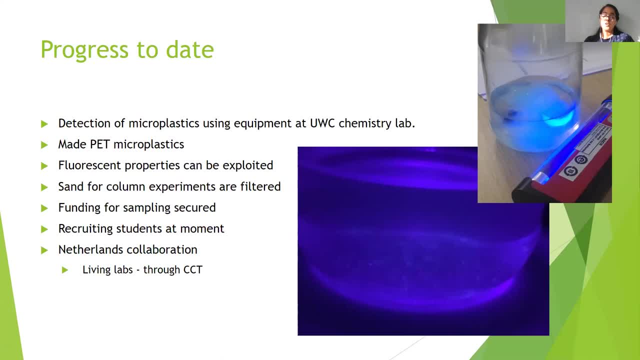 microfibers that we've made in the lab from using pet, and then we've also collected sand in the cape flats aquifer and we filtered them and it's in preparation for the column experiments. and then we've sourced funding for for the sampling and then we've also- we are in the 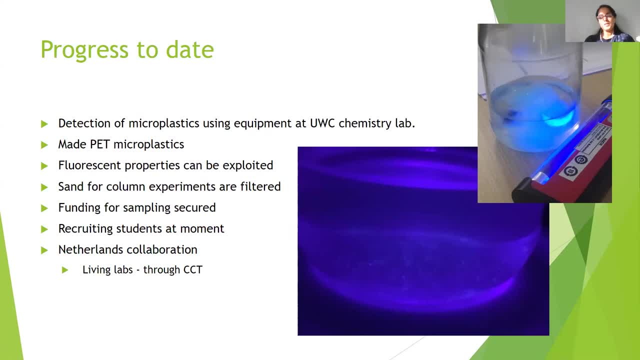 process of recruiting students. so if anyone's interested, please pop me an email. and then the city is also supporting me with the studies and they've now formed a collaboration with the Netherlands, so there will be a living lab. it's, it has formed one of the living labs topics and and it's done through the city of Cape Town as 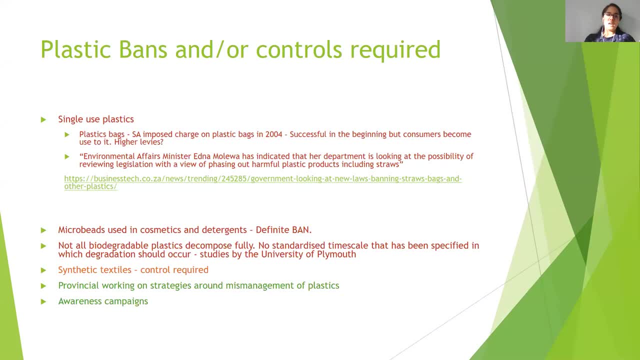 well and then- sorry I didn't put that in the outline, but just looking at plastic bands or controls that's required. so you know some of the issues. we know, and we see it all the time, is referring to the single-use plastic which end up on the landfills and all over. 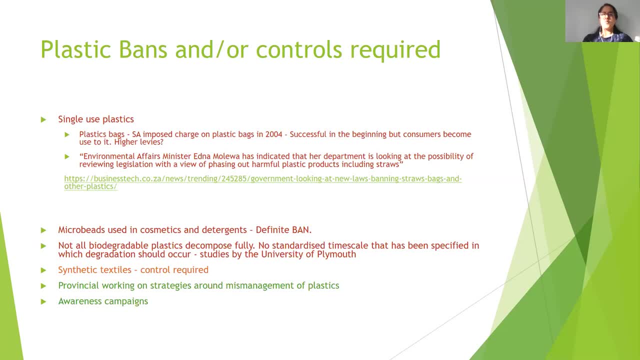 the city, and so there was a charge imposed in 2004 on plastic bags, but consumers just became used to buying that, and so the charge now means nothing. the plastic bag use has increased again, so it's either they need to increase the levy on that or they need to increase the levy on that. 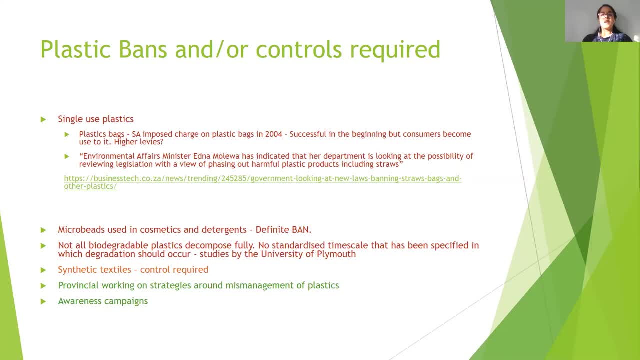 charge or do something else. and then there is the, the national department, environmental department of environmental affairs. they are busy looking at, sorry, re-looking at- the, the plastic bag legislation and also including all the other single-use plastics, like your straws and so forth. and then- this is maybe just my opinion, but microbeads used in your cosmetics and detergents. 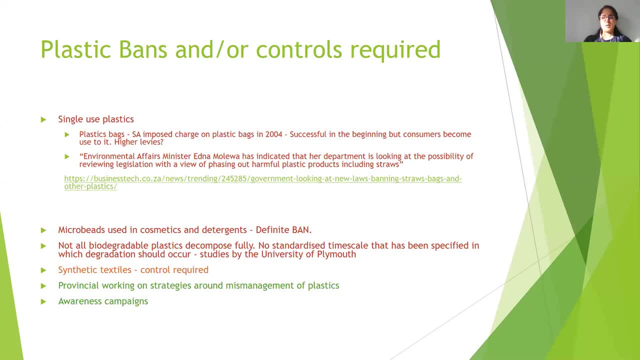 my opinion that it should be banned. I'm not sure how they're going to manage that, but I would prefer it to be banned. and then we also look at biodegradable plastics, which is now picking up. the research is picking up in that, but I've also found that some studies show that. 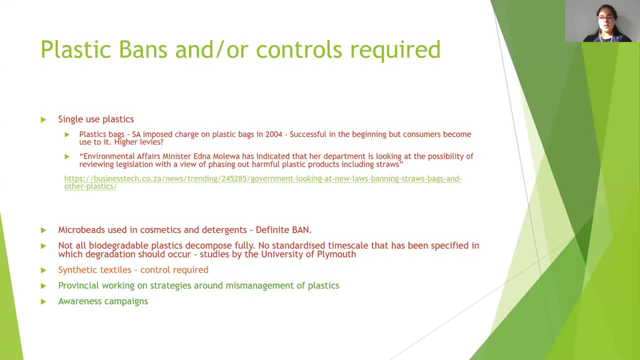 they don't always decompose fully. and then also the there's no standardized time scale for the degradation in which the degradation occurs. and then we've got the synthetic textiles, which is your clothing items. we'll have to determine how to control this and, coming in from 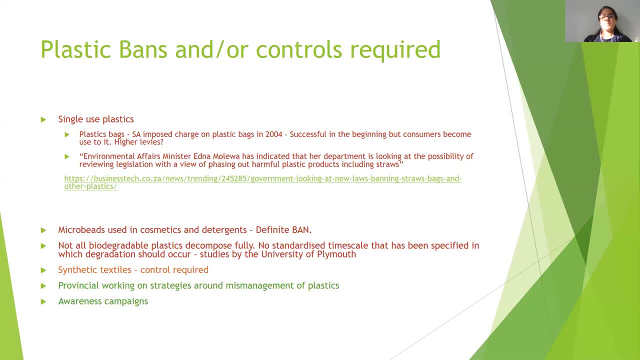 from your domestic areas. provincial department of environmental affairs is working on a strategy and looking at the mismanagement of plastic, so hopefully, whatever comes out from the study will also assist them in making decisions. and then, well, we can all do our work by awareness, letting people know. 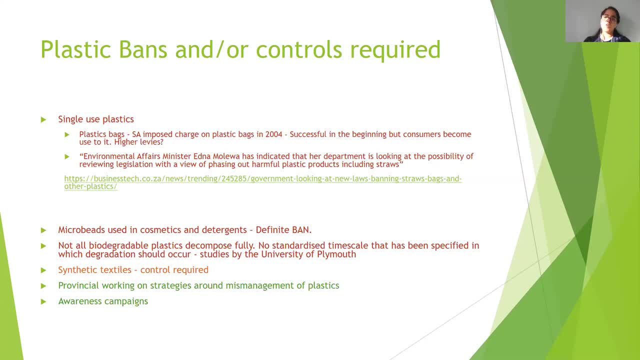 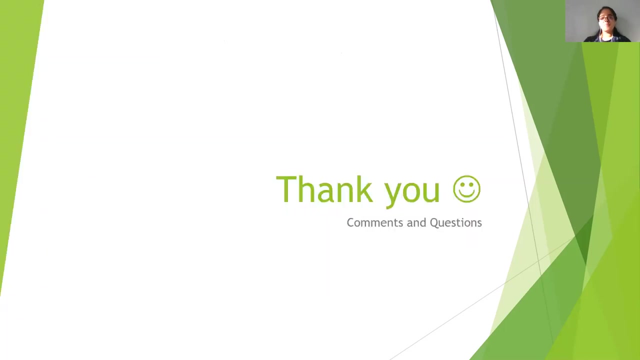 what the the impacts of plastic are, just being aware yourself of what you're buying, what you're using. is it necessary? do I really need to buy that bottled water or can I just take tap water? and that's coming from a city of Cape Town employee working in our water? so that is the end of my presentation and I think, Sumeya, we can. 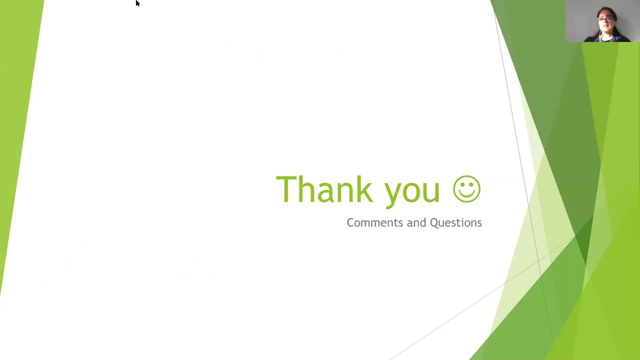 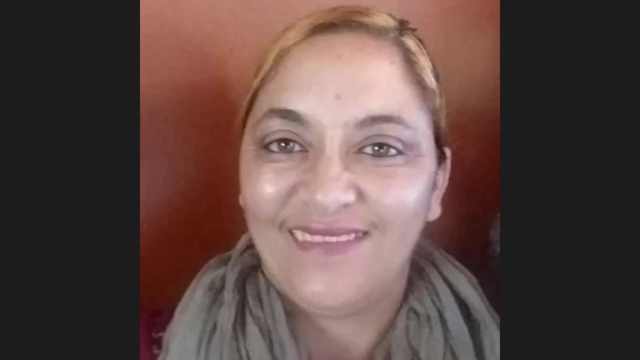 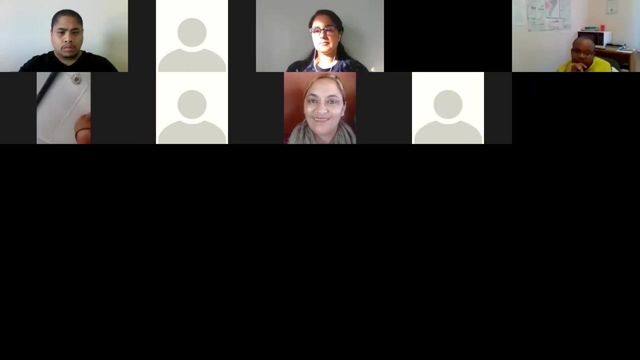 open up for questions. please, any other questions? thank you, Candice, for that very informative presentation. we really enjoyed it. so I guess we can welcome any questions or comments from the attendees. we have quite a number of you, so you could either raise your hand, which you could find under reactions, or if you're using your 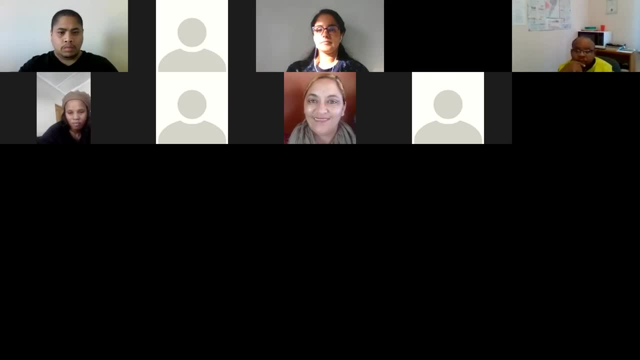 contact information, cell phone- there's something called more, where you can raise your hand: um, yeah, as can say: please go, go easy on her. well done, candace. this is a really good presentation, thank you, do we have any? we have many comments? okay, we have melissa. 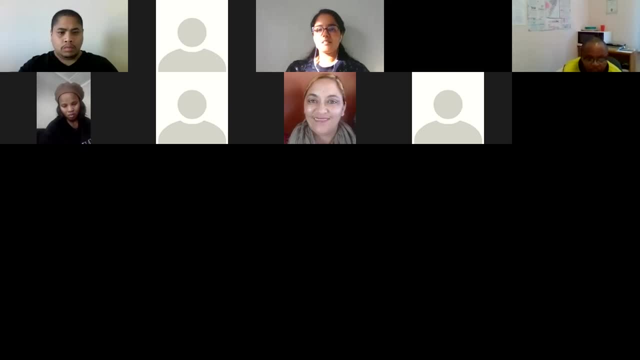 with a comment and she says: microbeads in europe is already banned in cosmetics. maybe candace? you can find out from the dutch how they went about that. it's a good question. um, yes, we have a question. i can't just i don't feel like a good presentation. 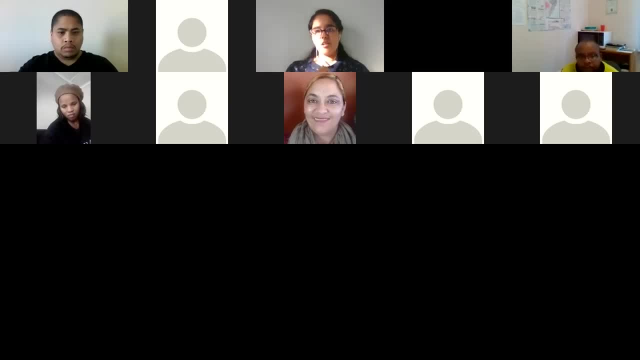 about this? uh, just a question, i don't you. you're breaking up a bit and you're really soft. can you hear me now, can you? i was like, yeah, you're perfect. thank you, yes, are there any? are there any ground with, uh, uh, ground with the sick chemistry signature related, uh, associated with the 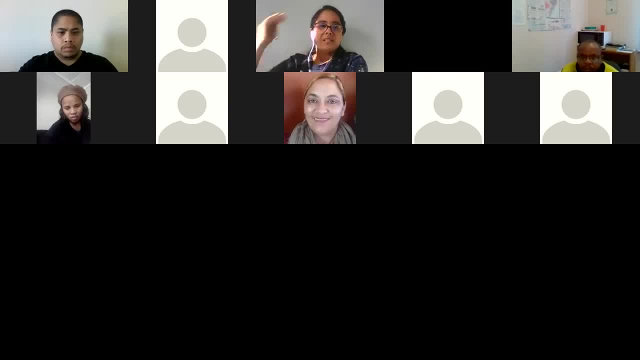 so i mean, you can obviously look at your total suspended solids, um, but remembering that there are other particles, um, floating around as well, which could then pick up when you are measuring total suspended solids and your turbidity, um. so, uh, we are looking at um, something, um, and it's 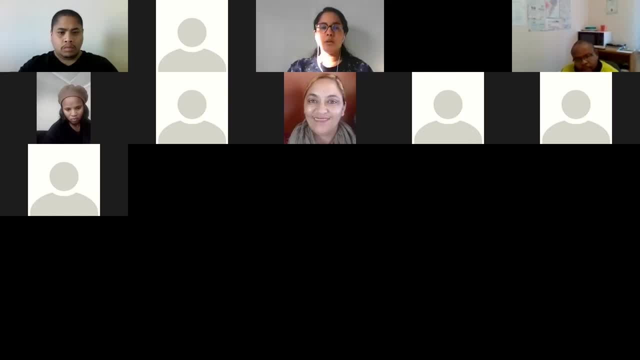 work in progress and um we we will hopefully present um to you guys in the near future. um what that results. we are trying to determine if we can pick up a signature using specific parameters. question from john weaver. yes, can i go ahead? yes, you can go here, john. thank you um john weaver here um. 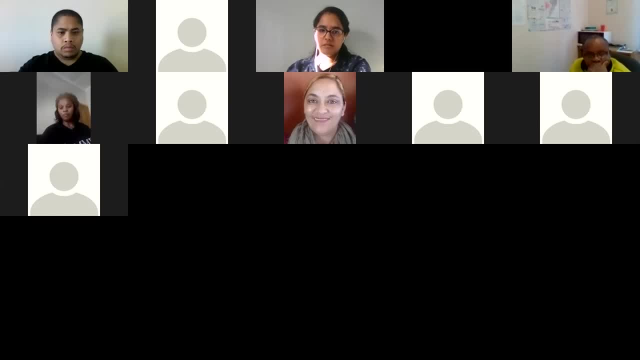 i'm obviously uh, very uh involved in the bottled water industry as i'm chairman of the of the bottle water association, and this uh story of microplastics in water has been very much in the forefront of the bottled water industry for the very simple reason that the only substance that researchers and microplastics can really look 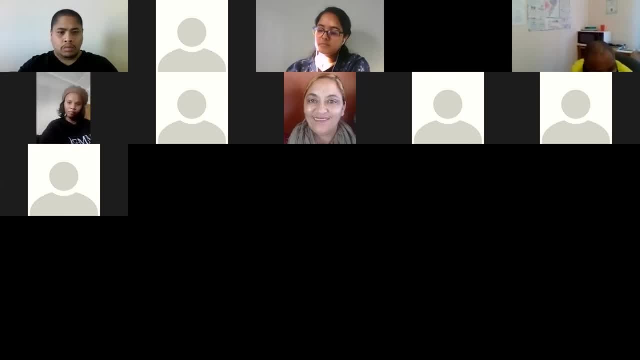 at is water. you can't really look at any other stuff that we consume, like hamburgers and coca-cola and whatever, because you can't see the things. so they're always, always looking. they're always looking at water. so one of the things to be careful of is not to get to. 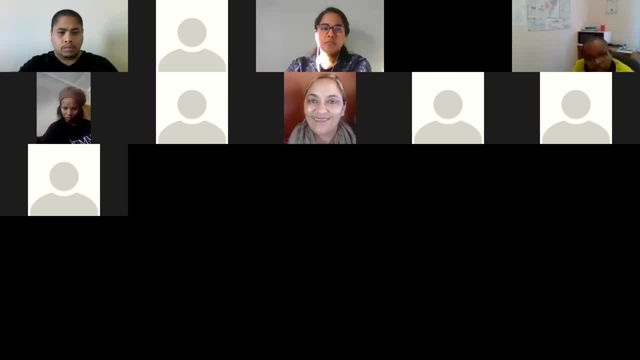 to take the world's worries on your shoulder because everybody's looking at water. um, it's just because they can that they do, and, of course, with the bottle in bottled water industry, we really you're breaking up with the water industry. um, it's, it's a target of a lot of, a lot of uh uh attacks, but 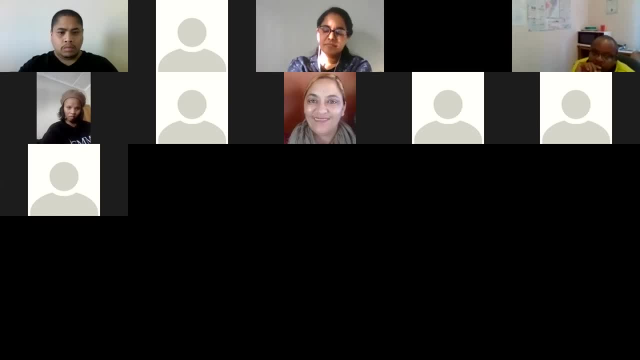 Okay, let's move away from that. One of the positives that I've picked up here is- and it only really struck me now, thank you, Candice, for your talk- is if your microplastics start clogging up in the aquifer, then they are going to absorb harmful organic chemicals and retard them and let them flow through the aquifer much slower than they normally would. 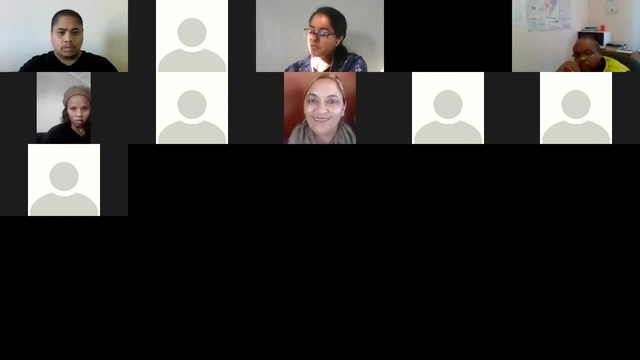 Which is a really good thing. So microplastics is not necessarily in the groundwater, it's not going to be such a bad idea. That's a comment I've got, And last one. I've got one more other comment to make. if I make- sorry- two comments: One comment and a question. 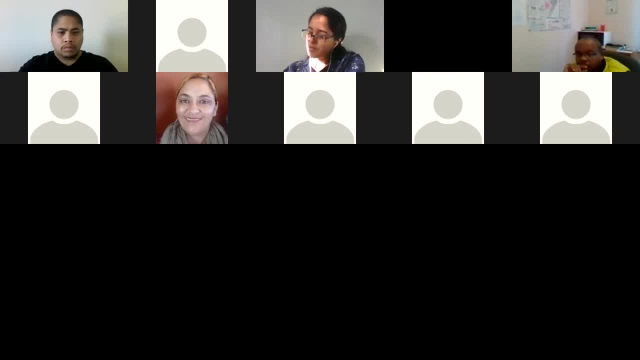 The other comment is that the two biggest contributors to microplastics- And then I'll start again- The biggest contributors, John, would you maybe like to type your question? It seems to be breaking up Your comment. sorry, Candice, we have quite a lot happening in the chat group. 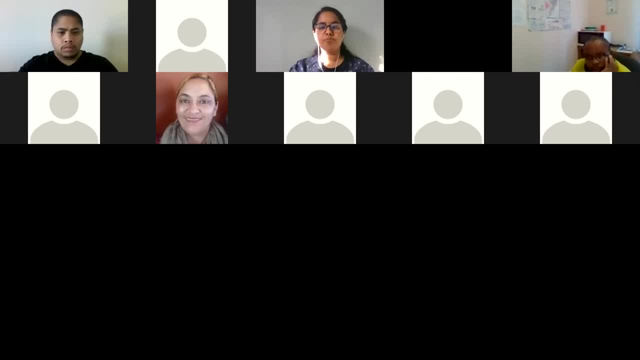 There's a few questions here from Alana. I'm not sure if I'm pronouncing that correctly. Will the city do any social research on willingness to change? Are you able to comment? So I can't comment on that that. um, obviously the city of cape town is really huge. it's got many departments, directorates. 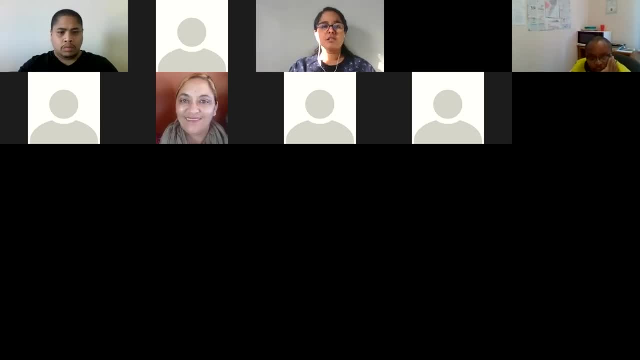 branches, units um. i am really just within a very small unit um in the bulk water branch and we are looking at this because we are doing managed aquifer recharge um in in these in the cape flats and the atlantis area. so um social, i can't, i really can't answer. 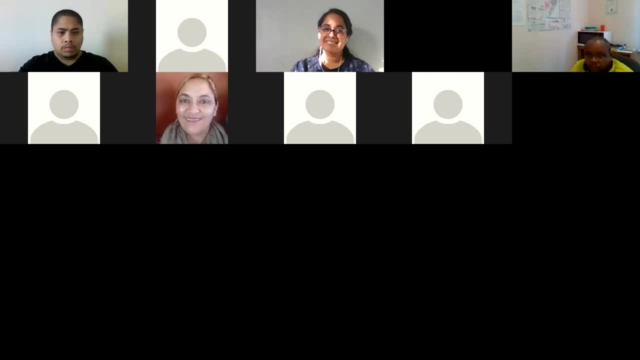 okay, thank you. i hope you've addressed the question, for i'm not alana. they may have case. who's asking: have you come across anything about whether the pvc casing used in primary aquifer four holes could be a concern with regard to your sampling? so it would definitely be a concern. um, but we are not targeting walls with pvc um paintings. 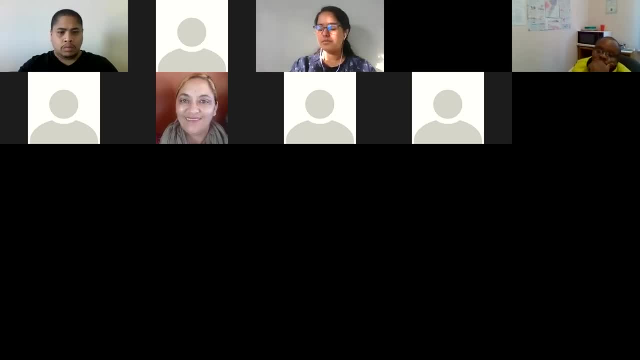 i mean i see kyle clinton added to that one um also looking at various equipment used at wastewater treatment plants. yes, yes, so that also i mean, if you look at equipment used in even in the about quarter, you've got your hdpe pipes um used for your interest. linear infrastructure. 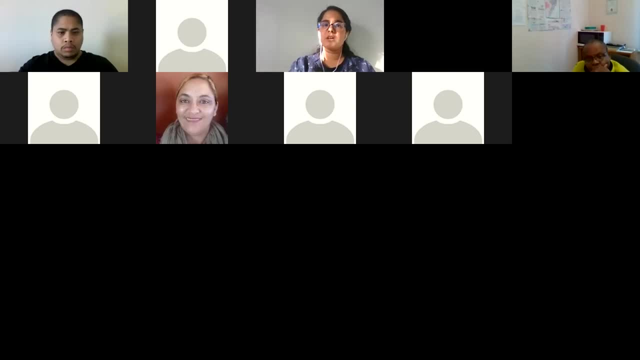 and stuff like that. so there are many contributors. um, it's, it's. the fact is we the? the objective of the study is not to determine where it's coming from. um, it's more an issue of what the impact will be and if there is an impact. 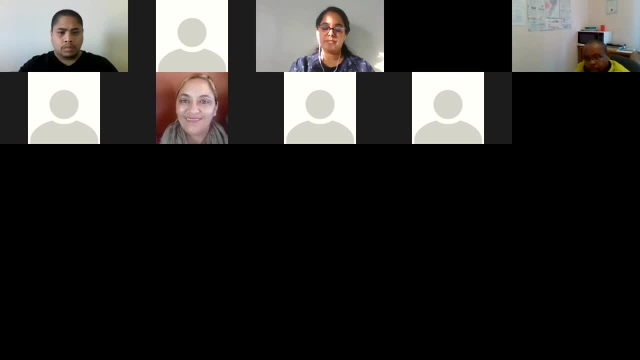 okay, thank you, um, but there are many questions. yeah, i'm gonna go one at a time. then we have majula asking: when do microplastics become a health risk relative to exposure period of the long-term exposure or even short-term exposure? at which point is this described as a health risk? 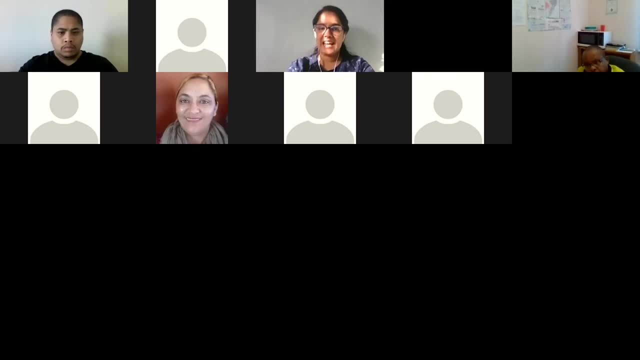 again. sorry, but i can't answer that. um, there are other people doing studies on um the toxicology. um you know whether it is toxic to uh human, i mean to the human health to a human. um, and and i haven't looked at at um the risk to humans. 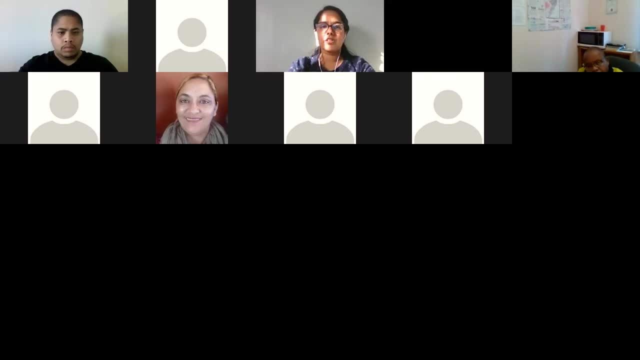 the research is only looking at the risk to aquifer properties, so, apologies, i can't answer that. okay, i'll give it this, the question to the for the person: um, there's another quite a few years candace. um, uh, i have a question since microplastics. 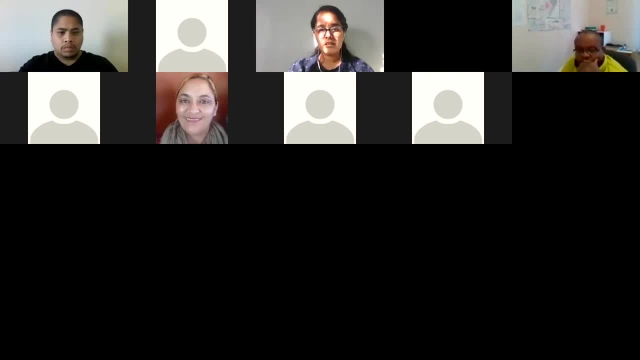 is a relatively new contamination source in groundwater. can they be simulated using the current available geochemical transport and reactive modeling methods? um, i'm trying to look for that question as well. okay, at 0334 pm. the person wants to know. oh sorry, hello hi, i'm sorry, my, my dog is barking like a dog. 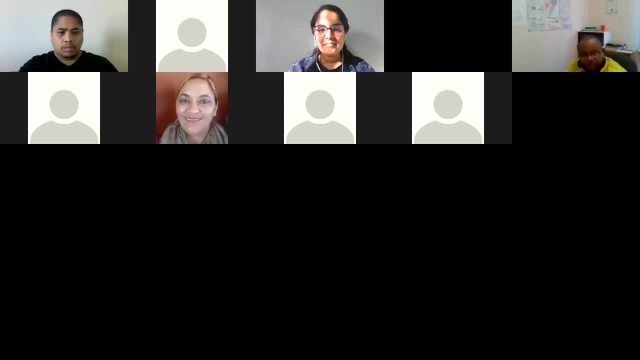 oh, wow, uh, i'll try to look the live at the background you can see it's very loudly. okay, they want to know if it's possible for you to model microplastics transport and reactive modeling. that's been modeled and we can use that to model to model microplastics, so but 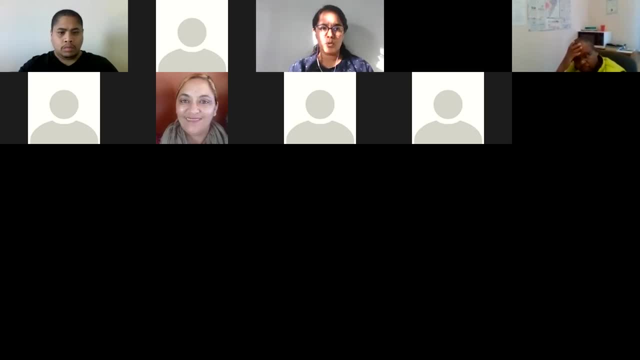 we have looked at the colloid transport models and and hopefully they they respond in a similar manner to these microspheres and we can use that. okay, there's another question here: is there a way to determine whether microplastics detected is from PVC or from the aquifer itself? okay, so I'm trying to understand that question, so you. 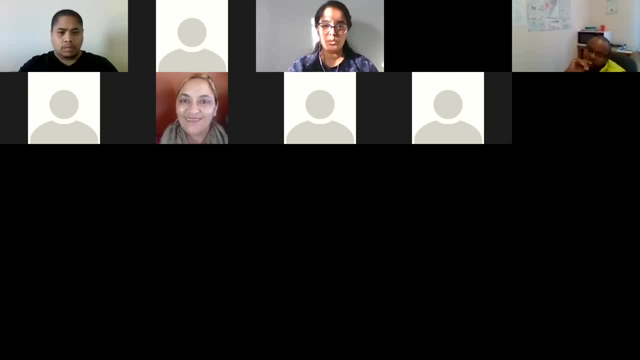 want to know if it's from the PVC that the casing used or if it's coming from from the aquifer itself. so for now we we don't in terms of detecting microplastics. there are processes in detecting it. the source thereof we don't know. but I mean, if you 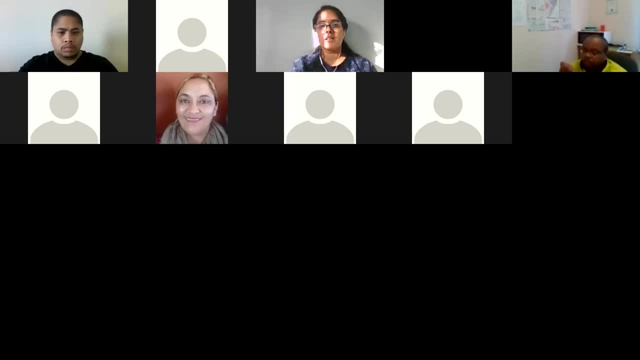 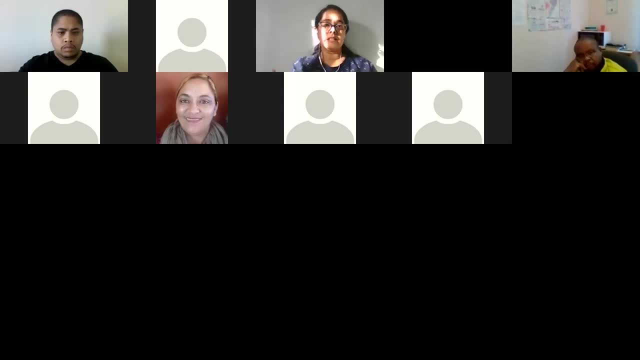 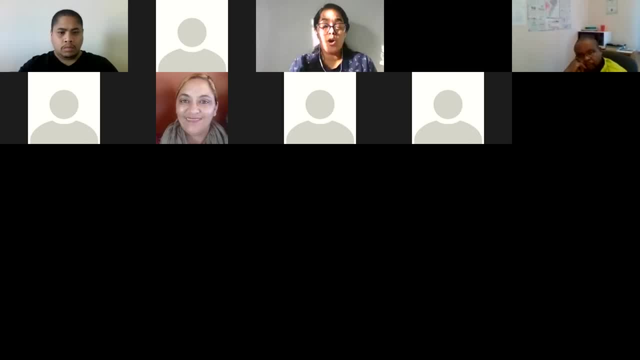 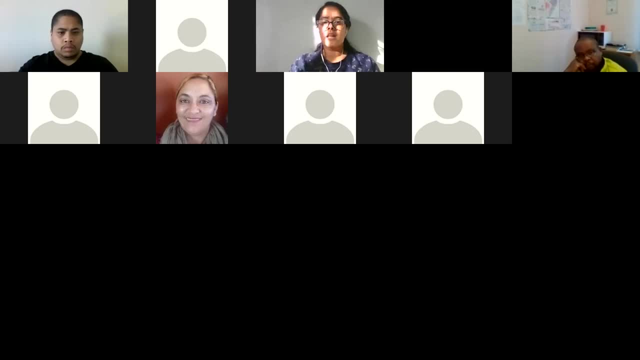 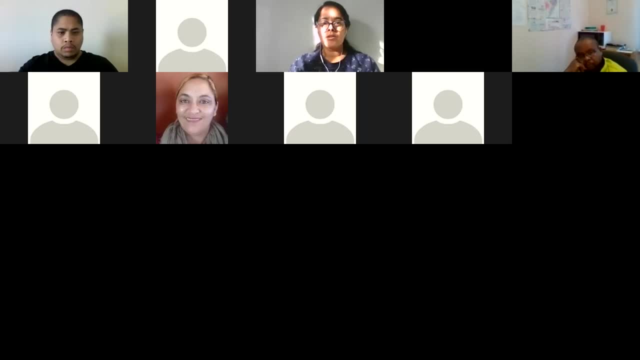 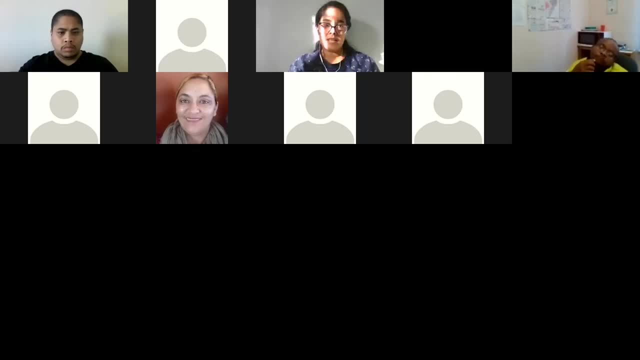 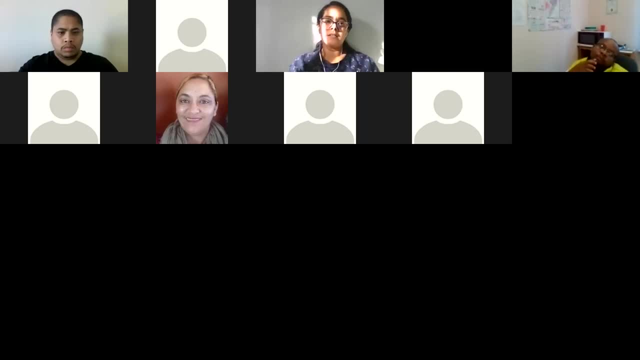 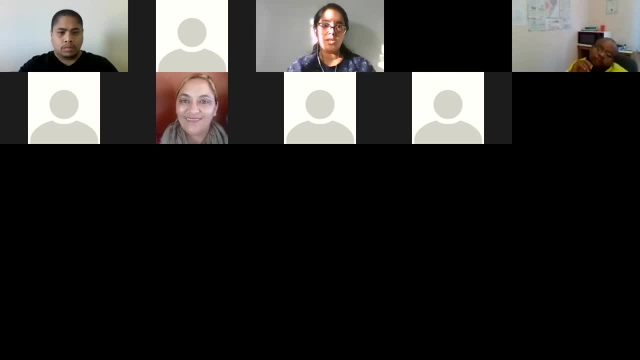 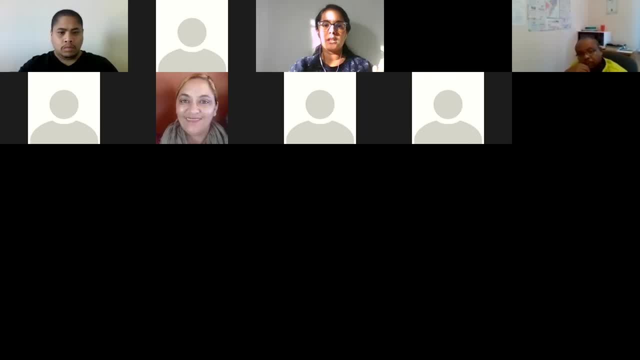 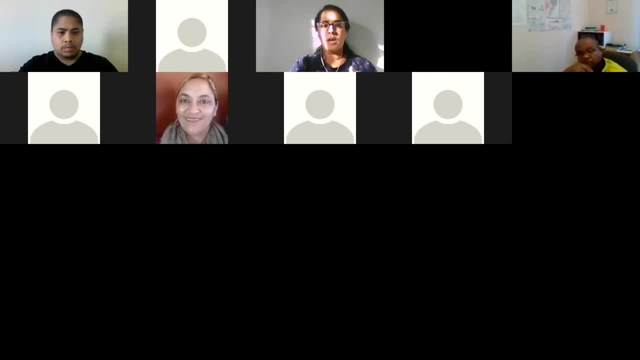 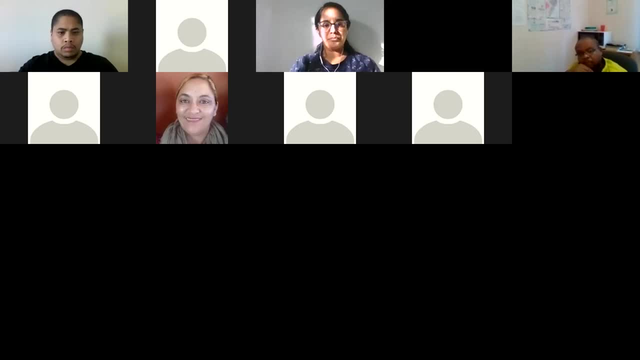 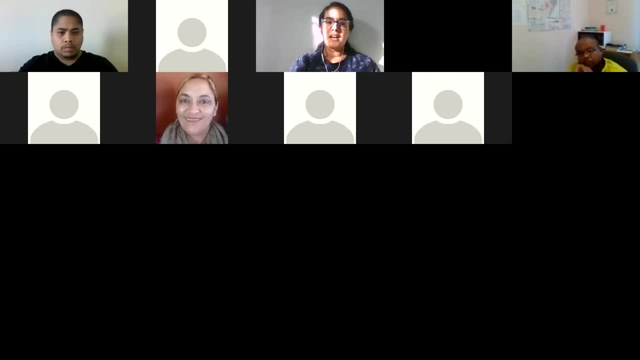 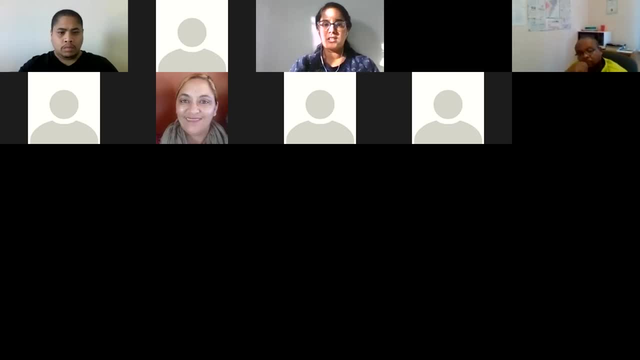 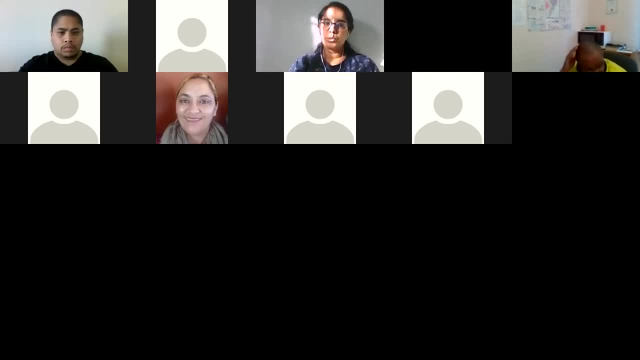 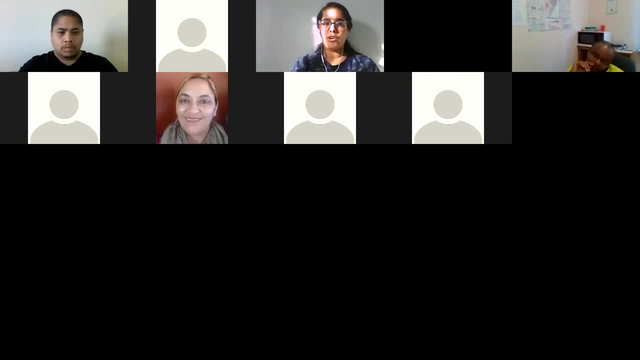 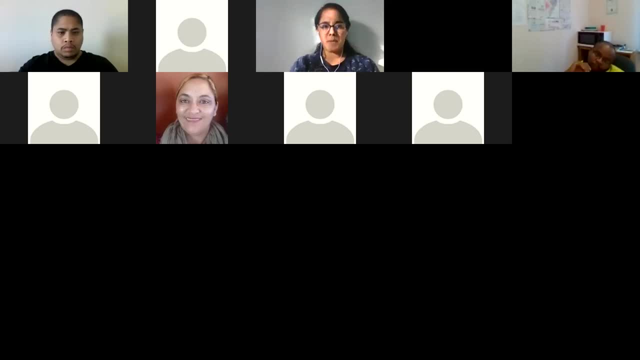 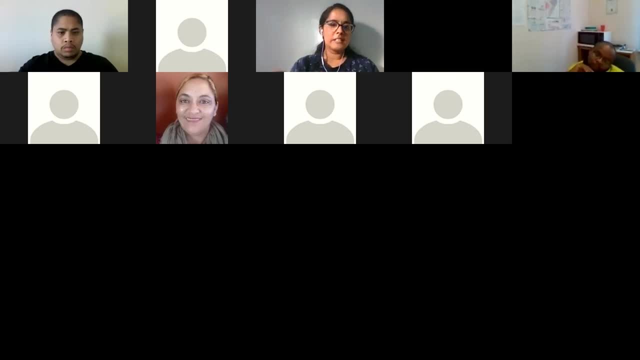 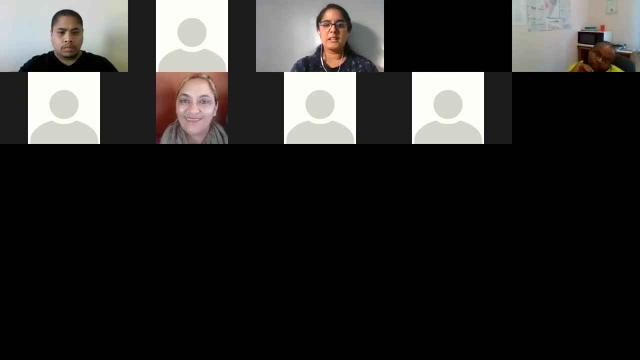 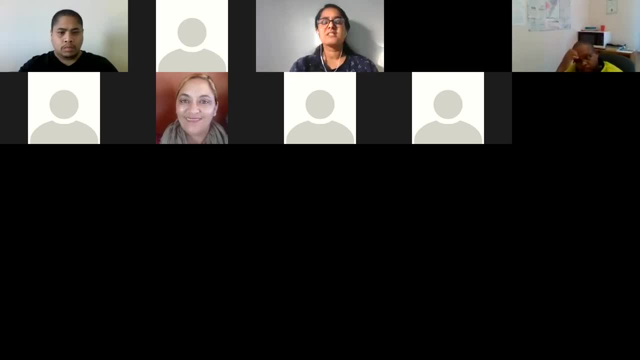 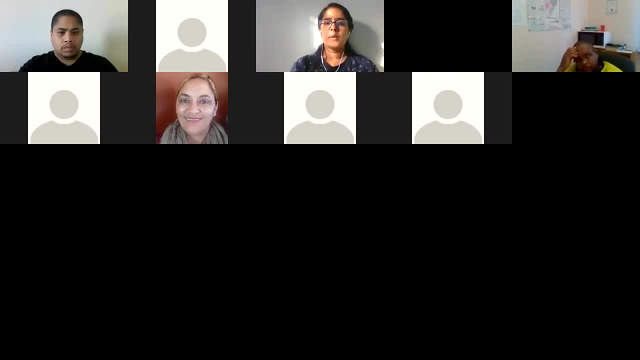 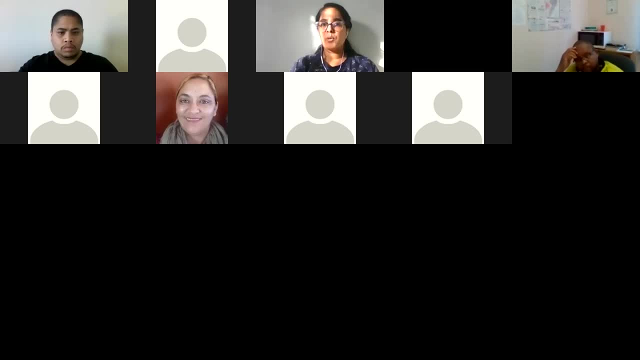 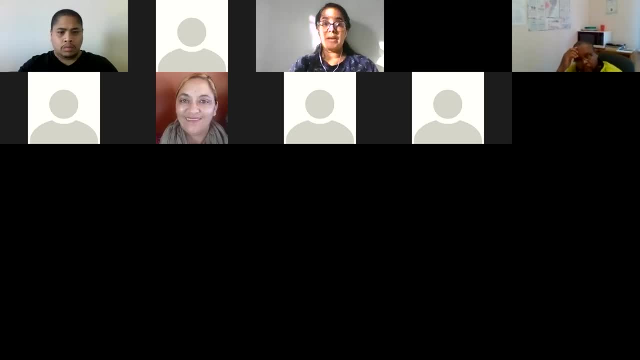 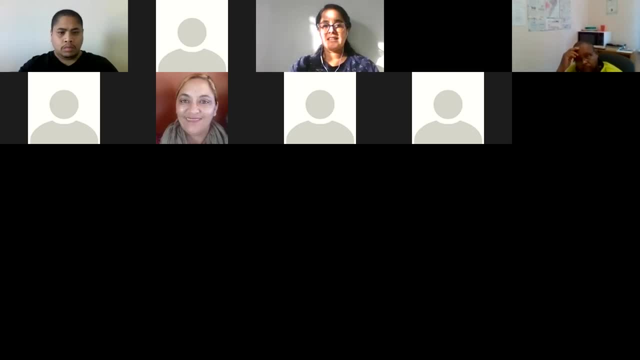 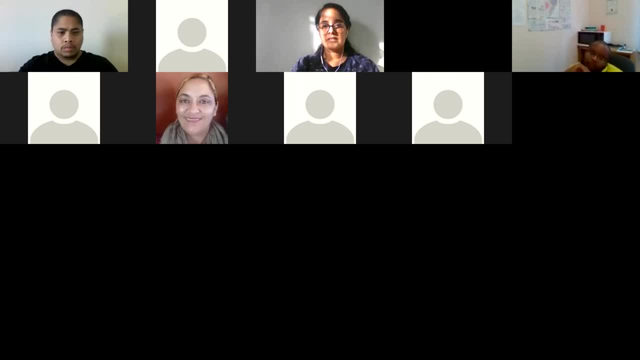 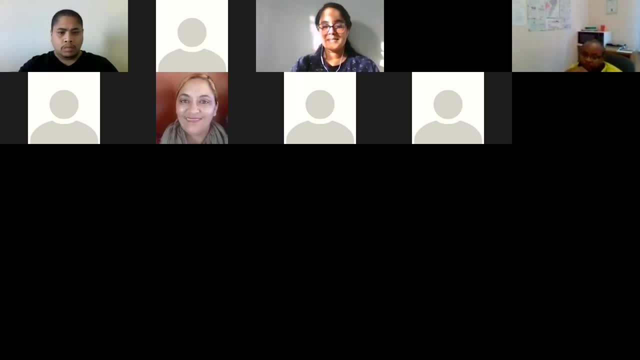 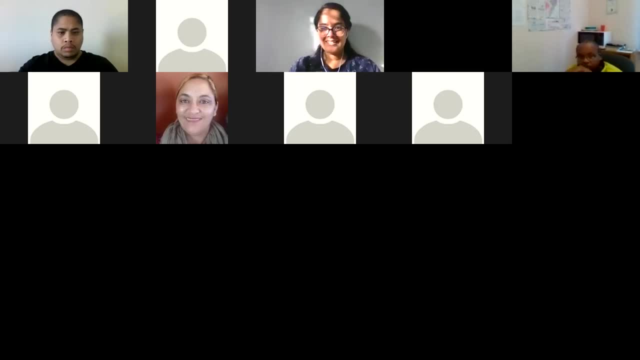 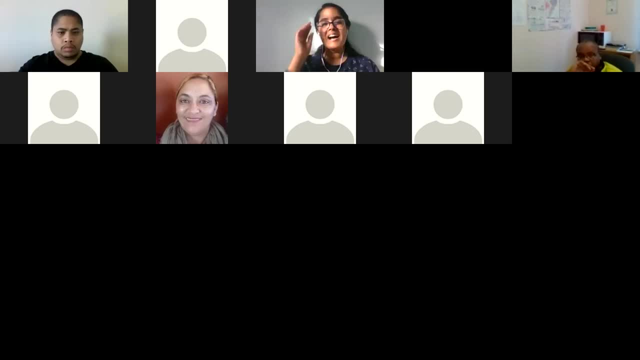 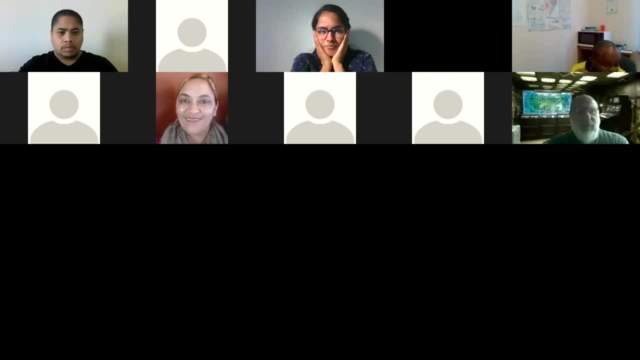 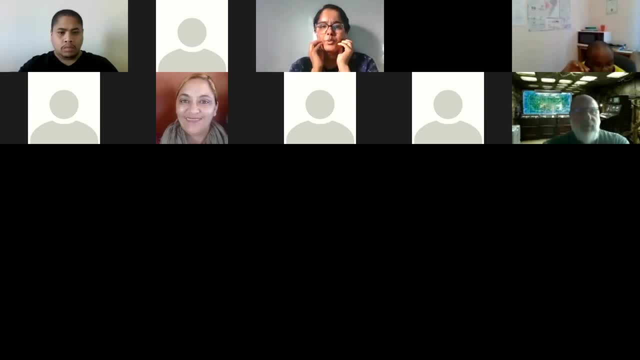 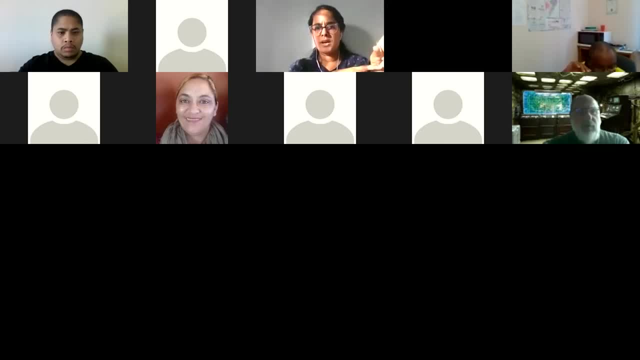 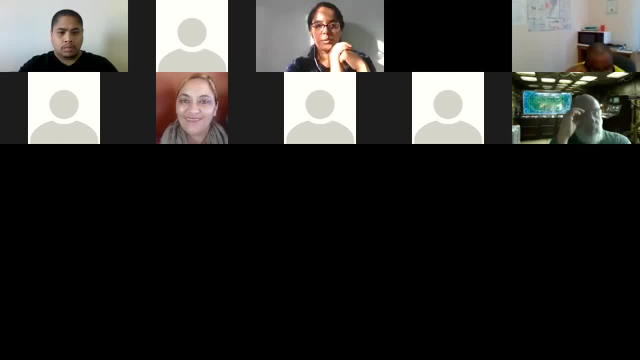 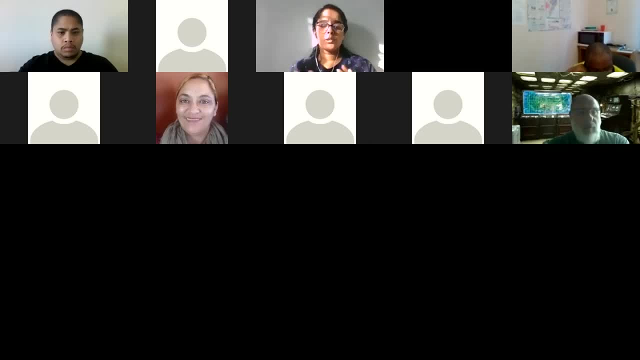 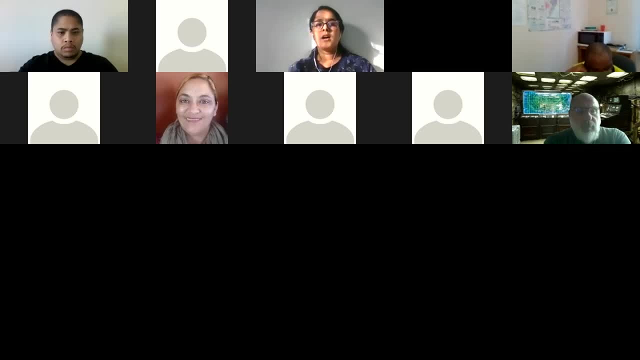 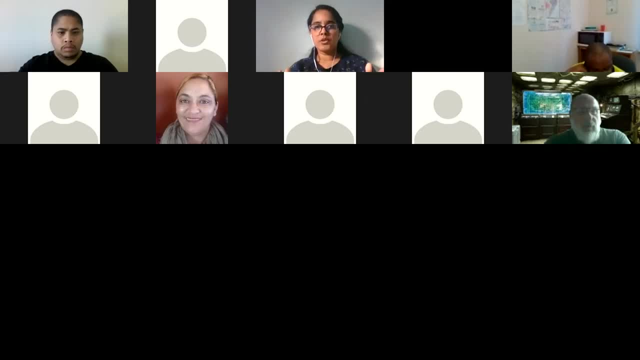 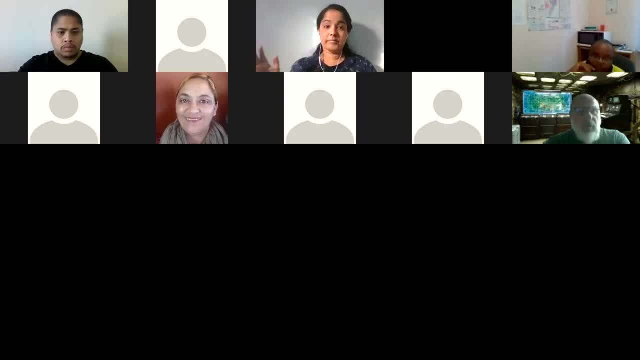 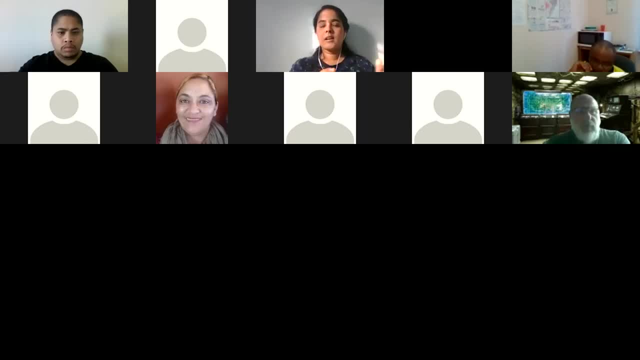 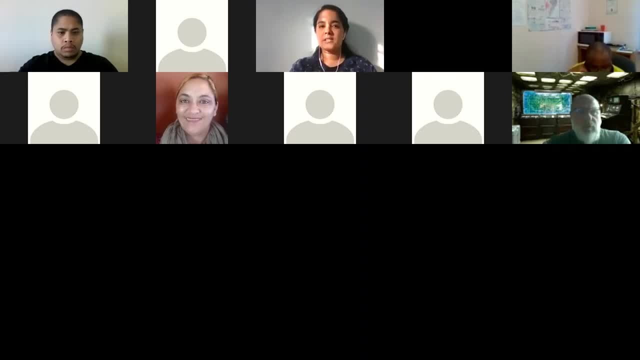 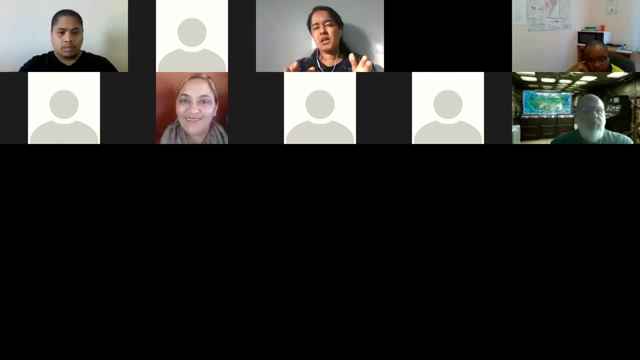 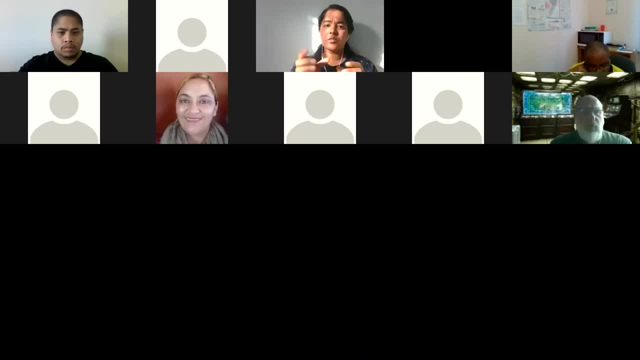 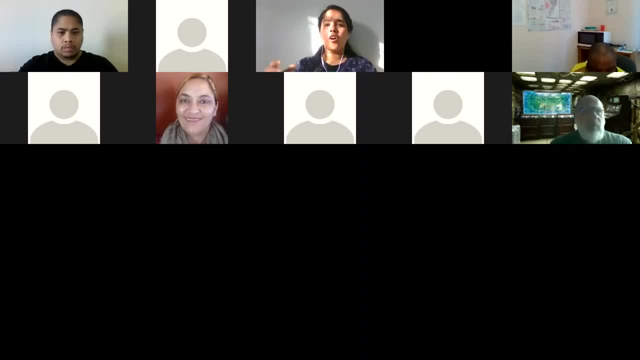 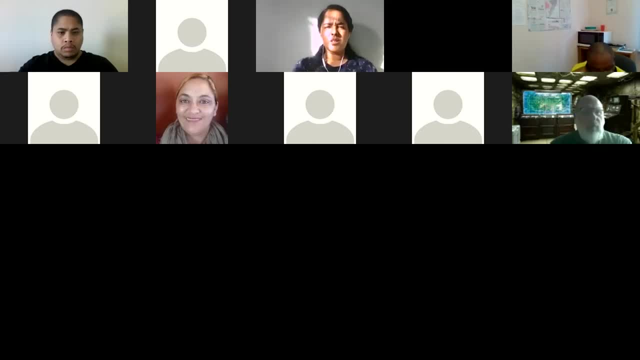 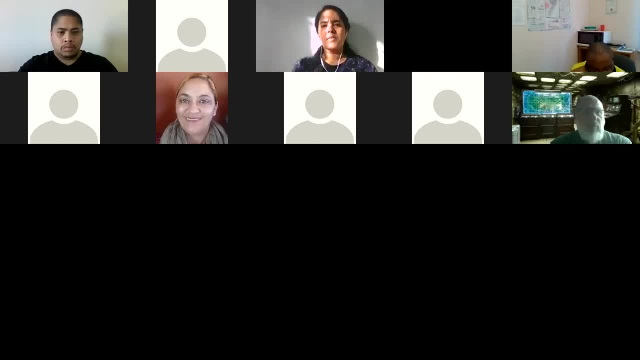 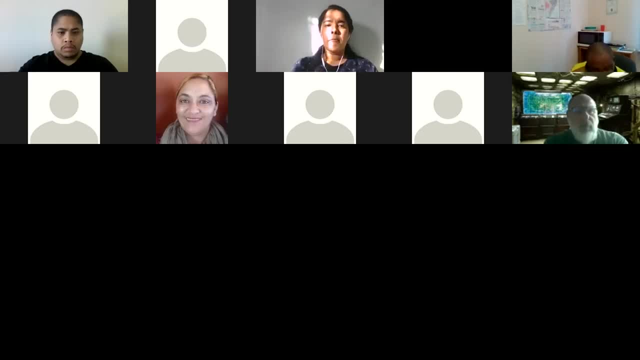 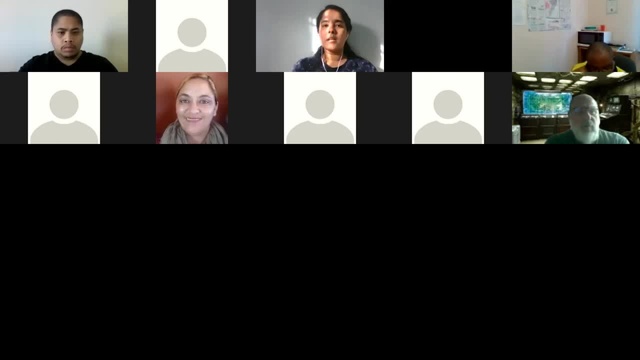 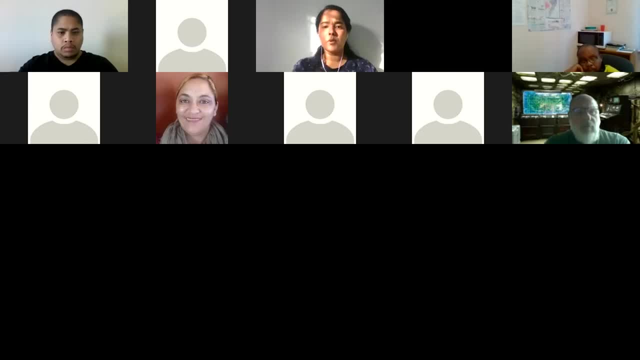 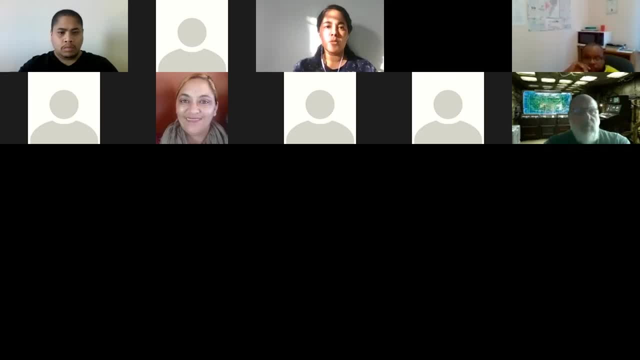 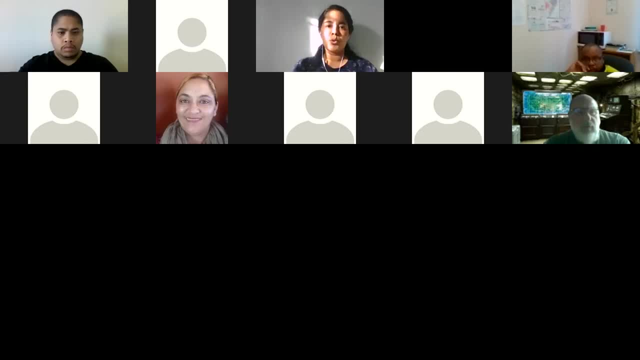 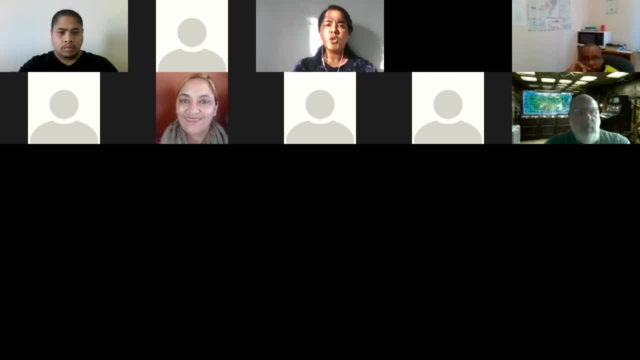 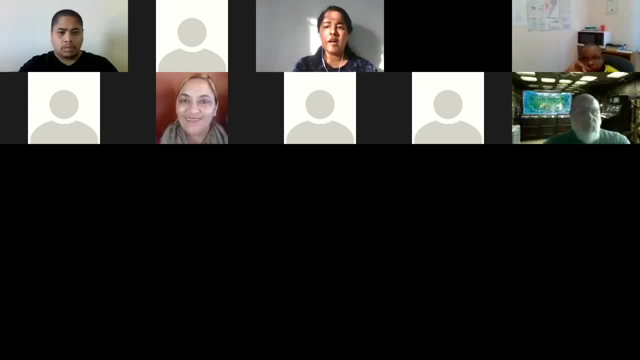 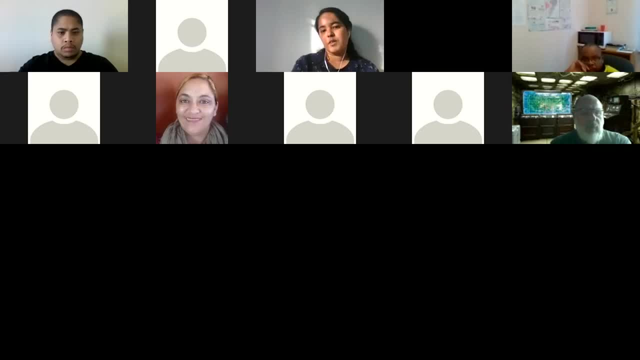 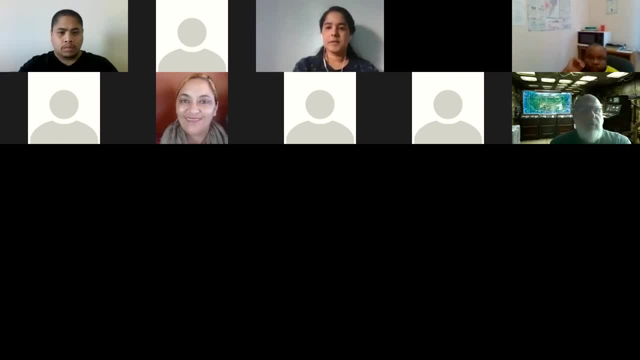 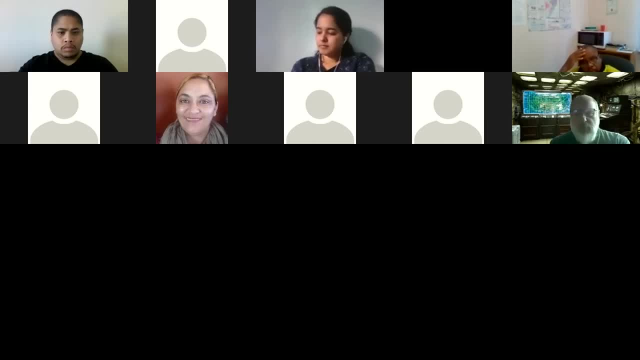 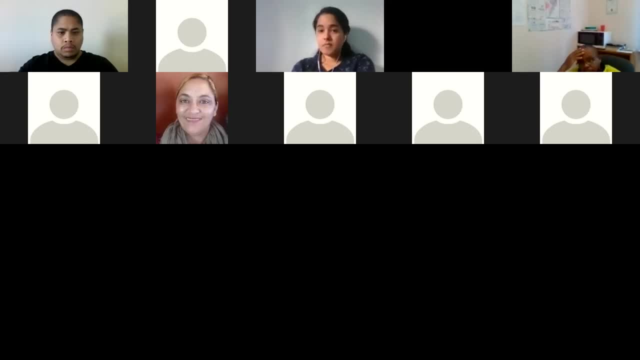 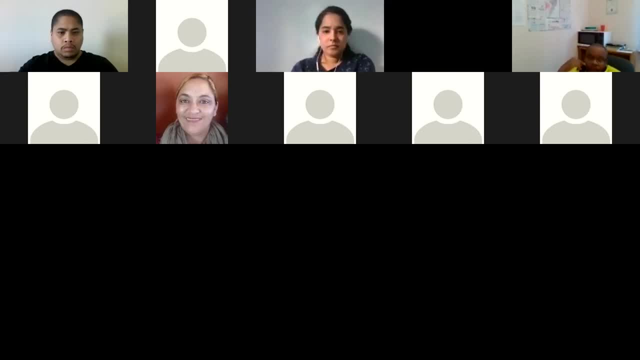 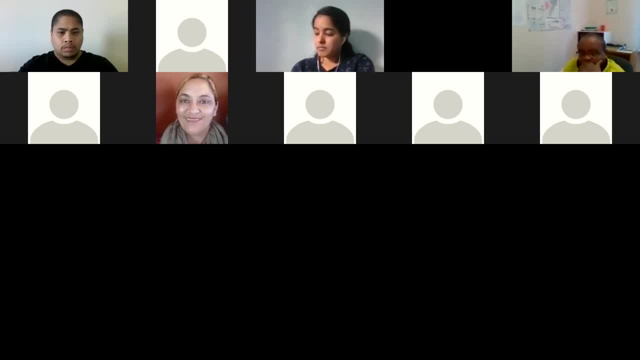 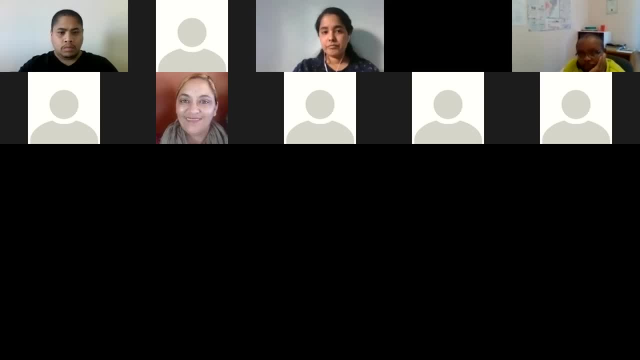 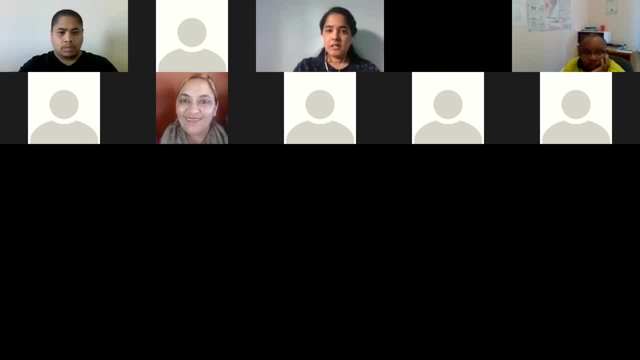 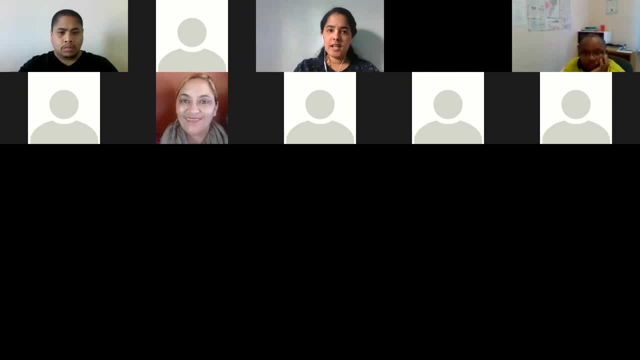 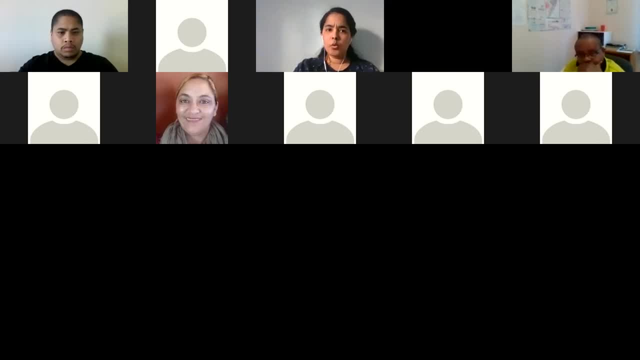 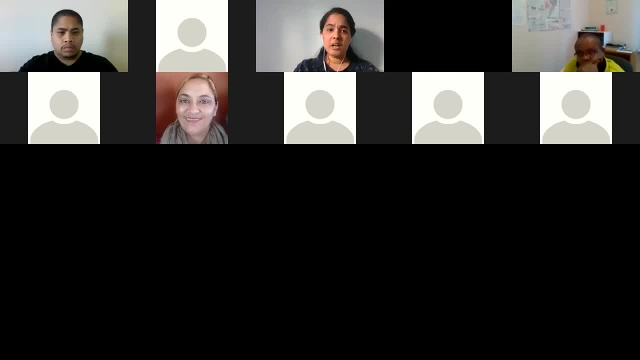 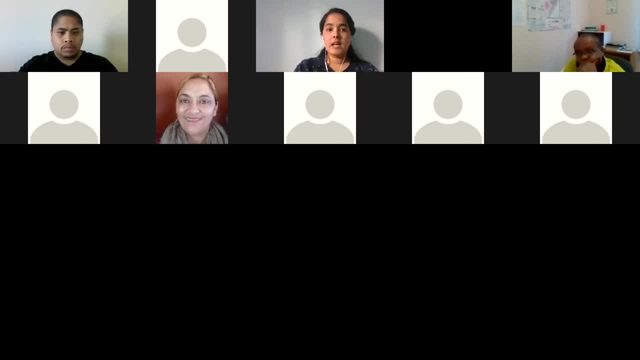 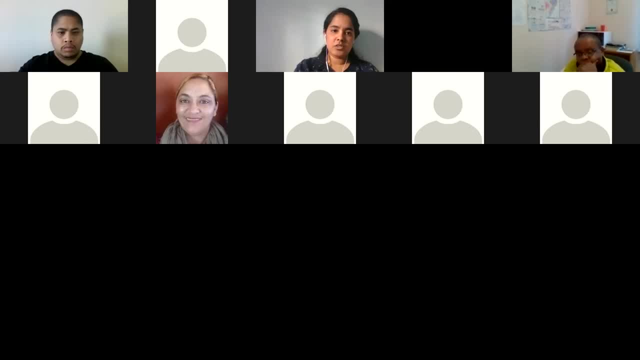 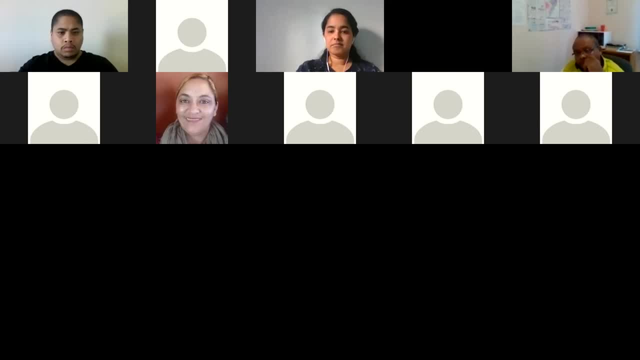 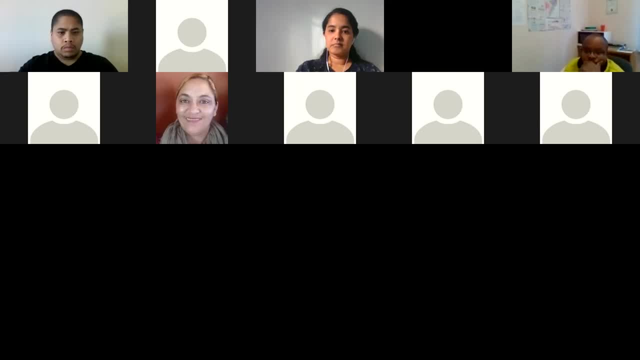 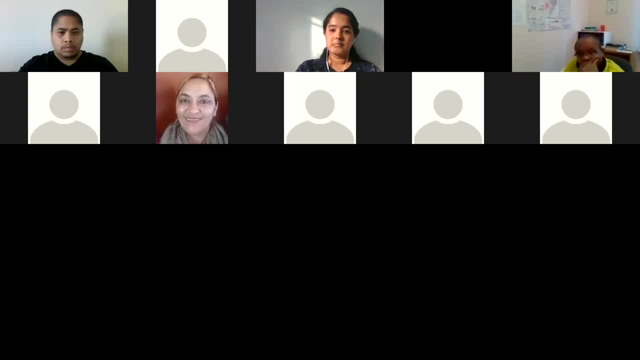 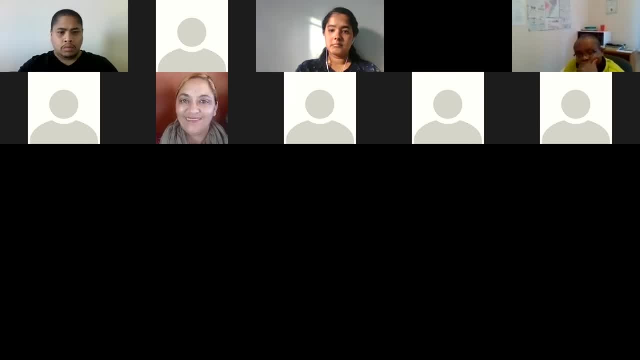 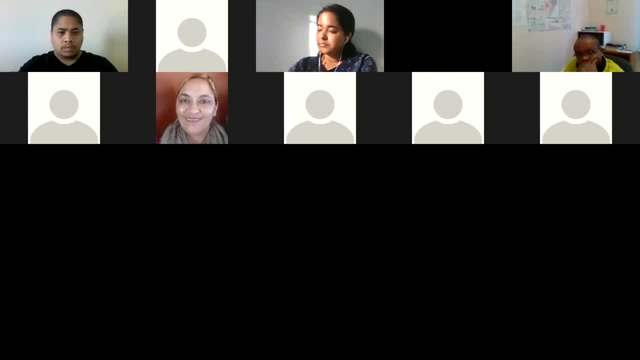 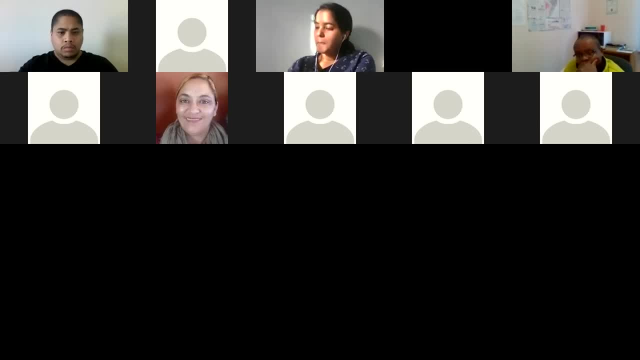 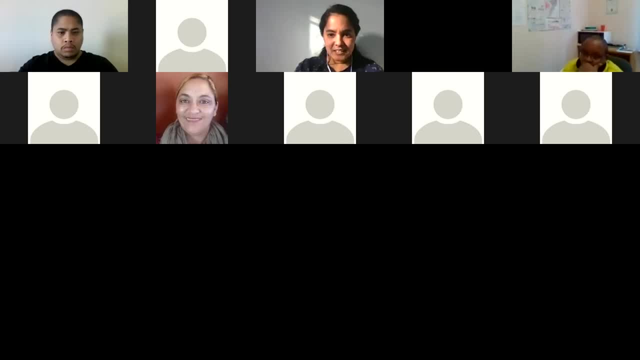 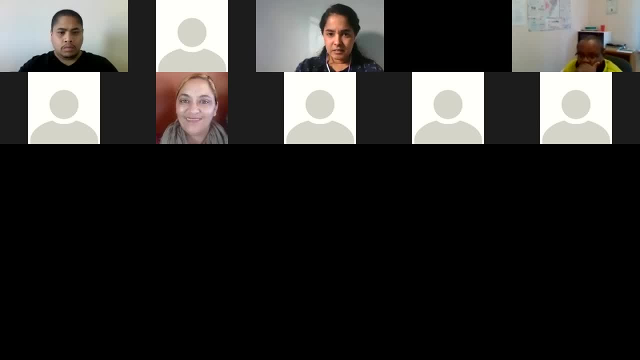 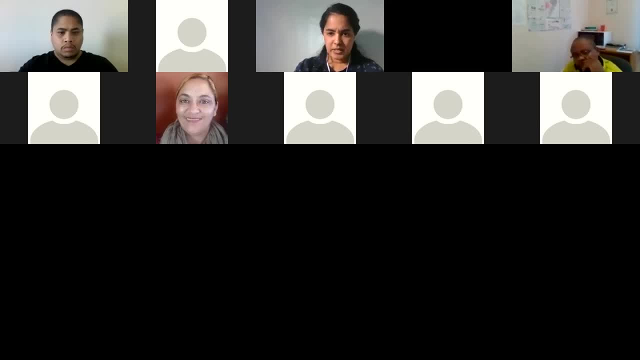 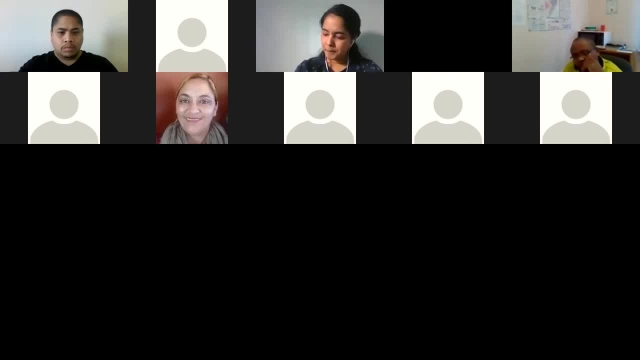 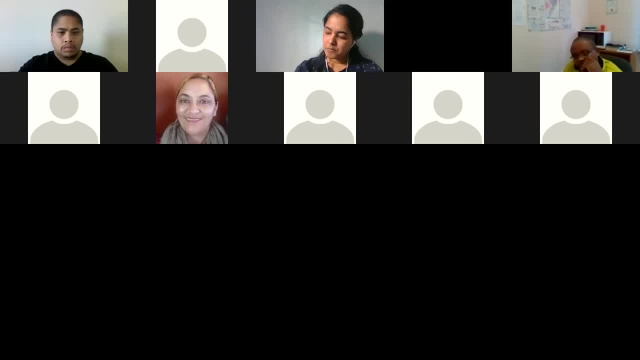 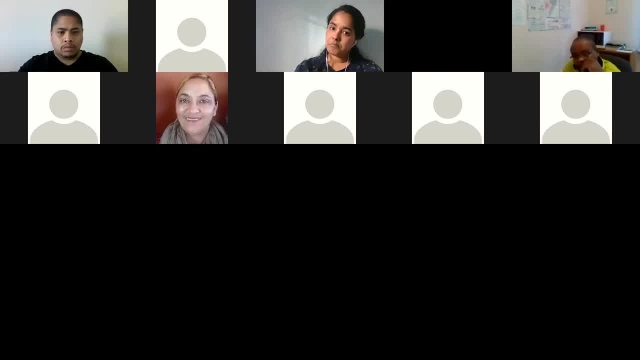 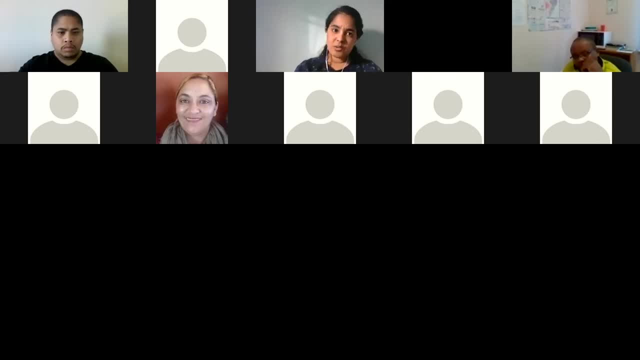 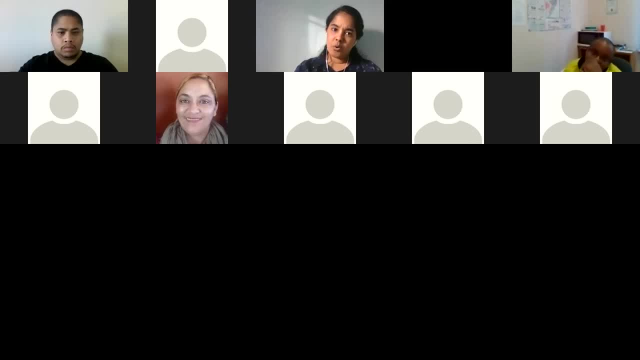 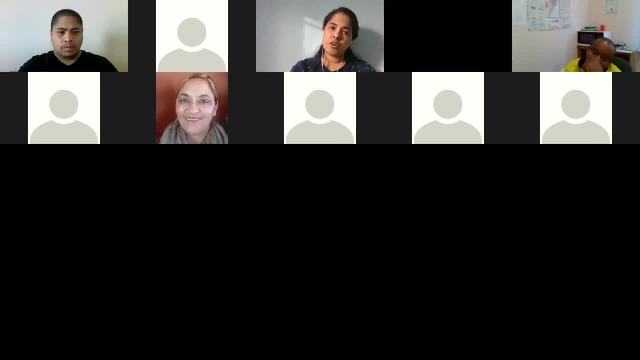 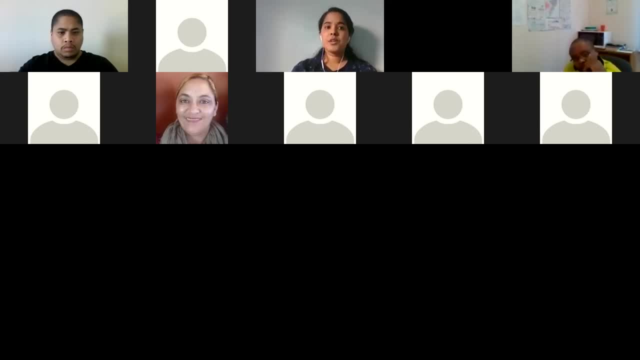 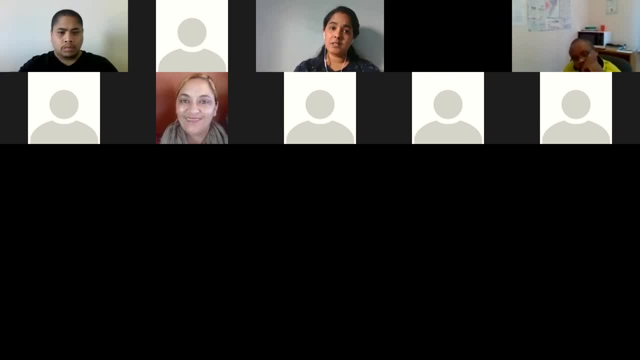 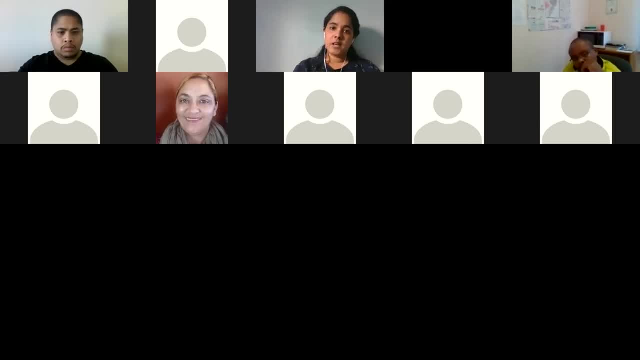 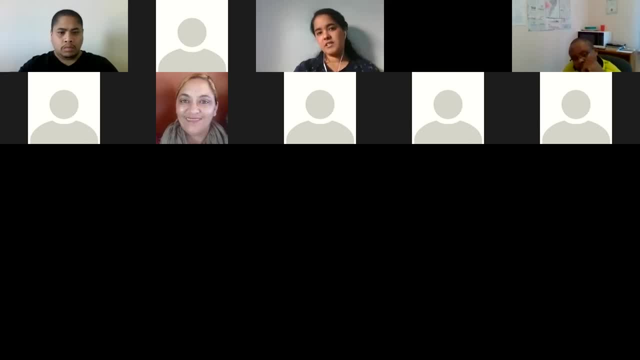 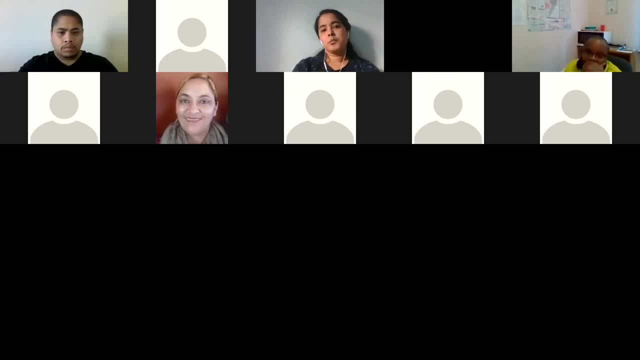 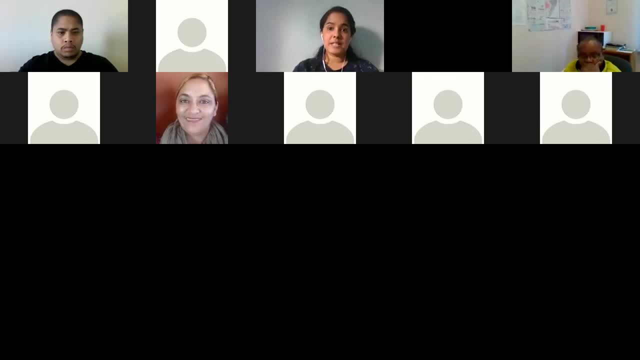 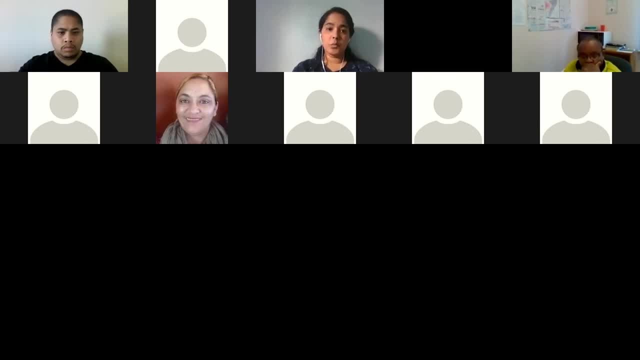 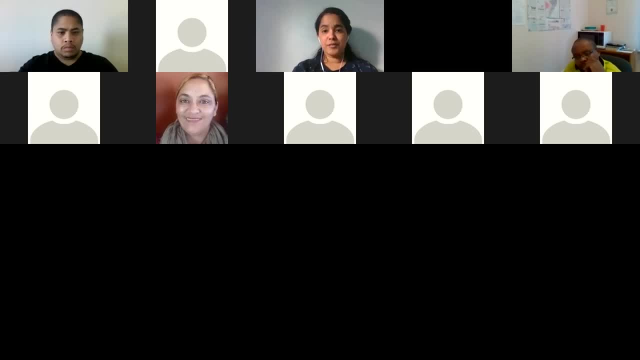 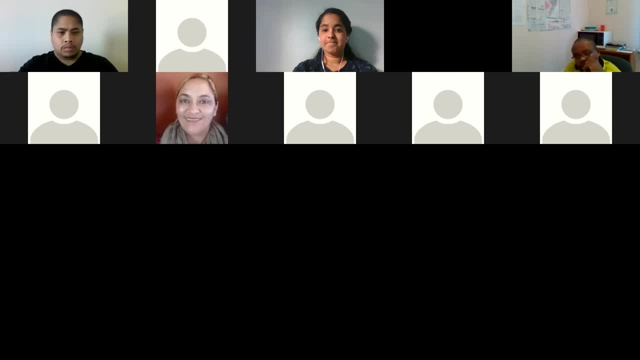 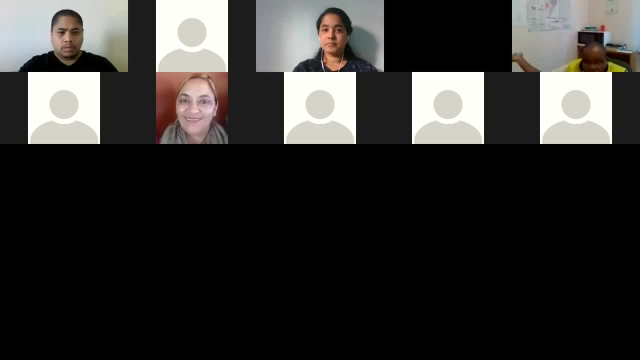 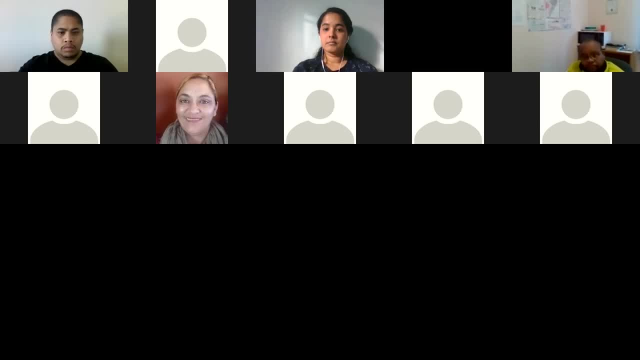 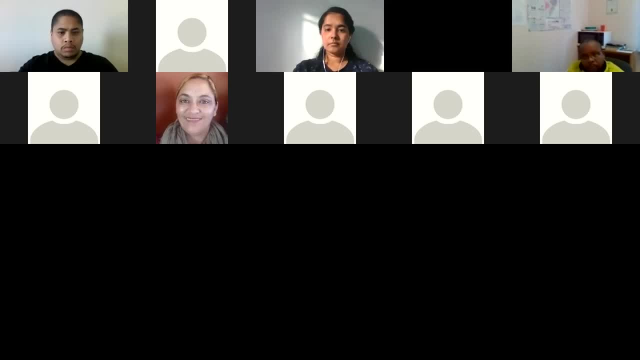 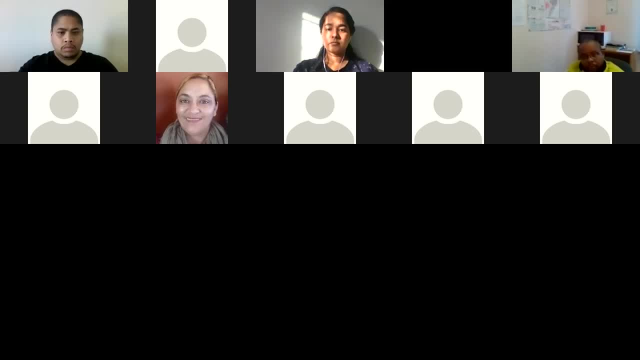 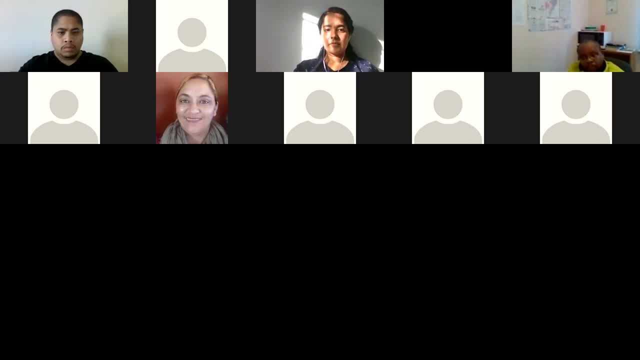 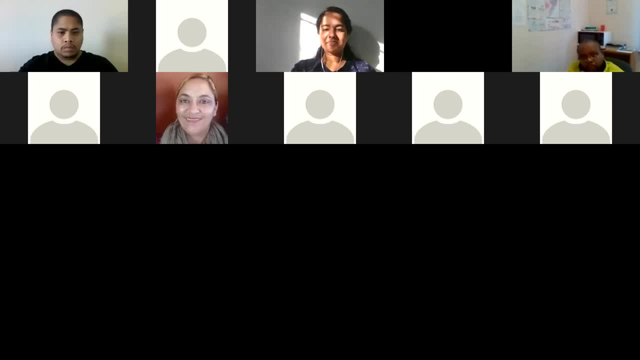 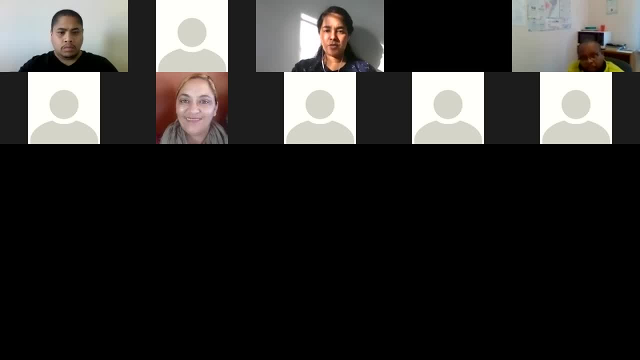 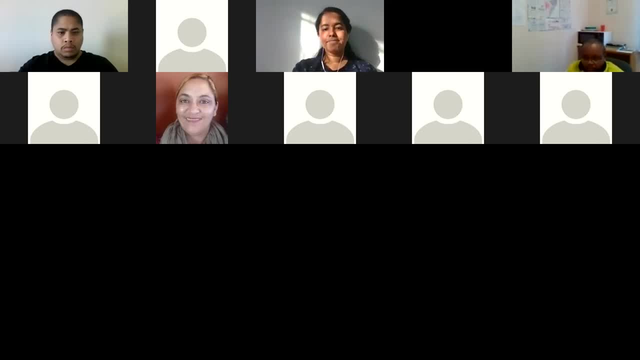 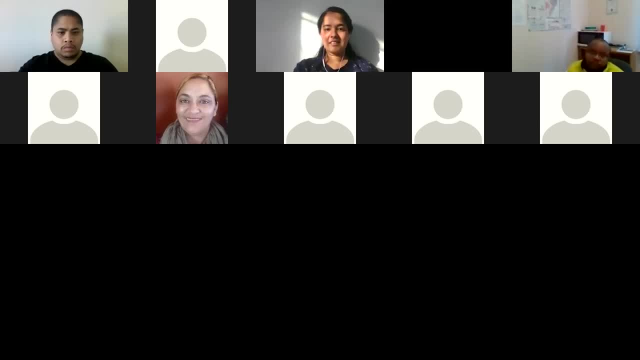 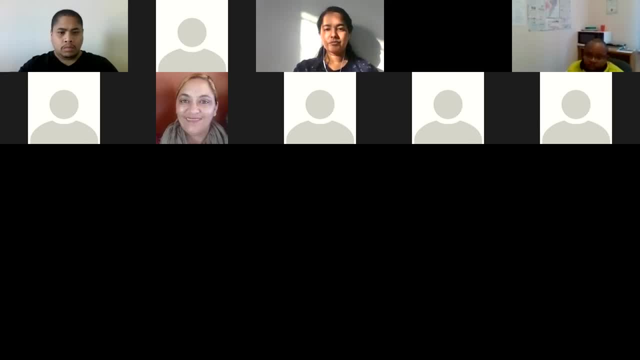 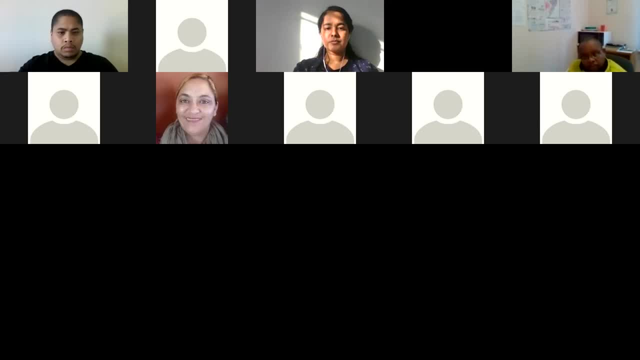 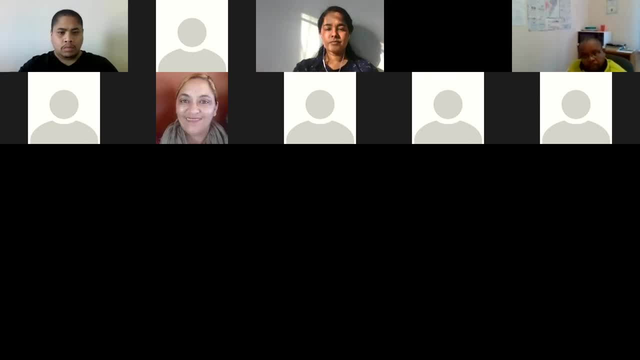 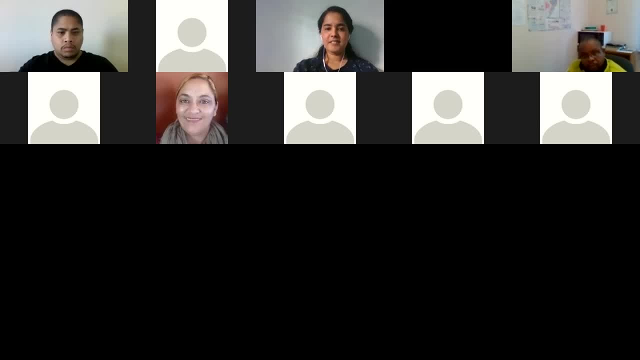 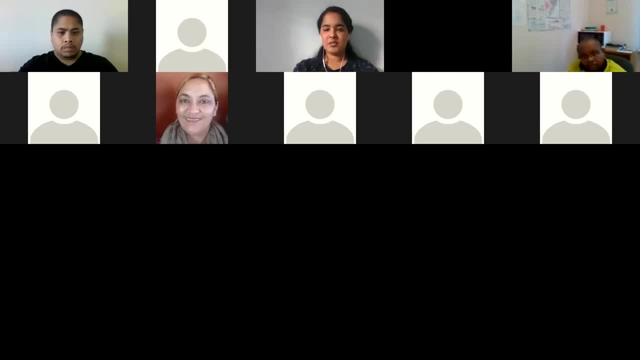 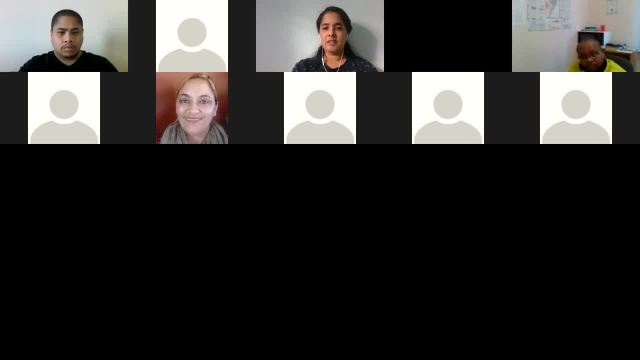 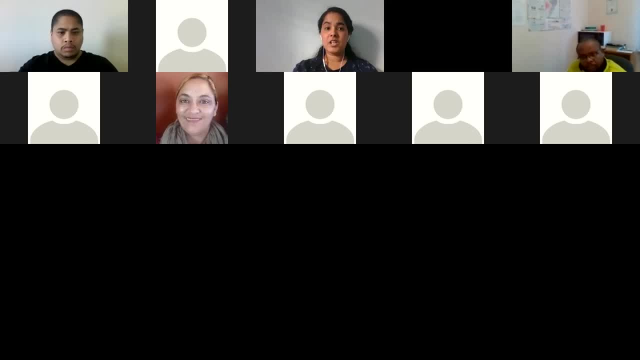 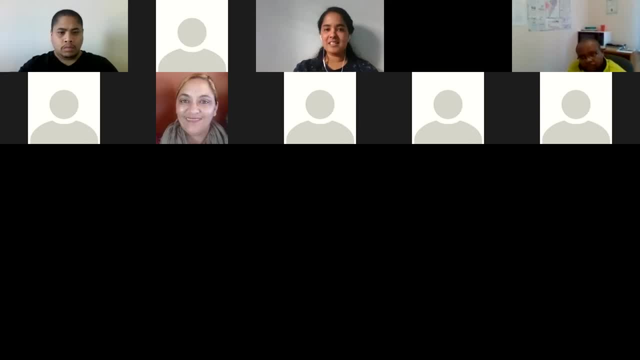 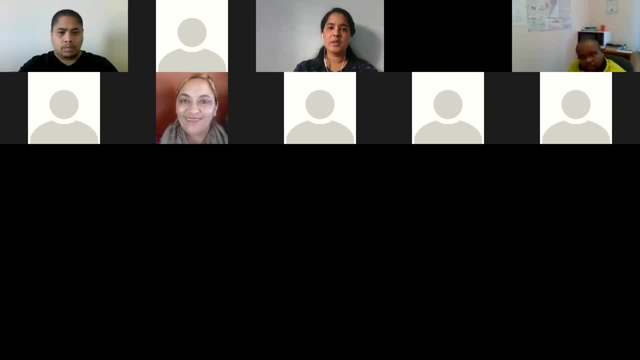 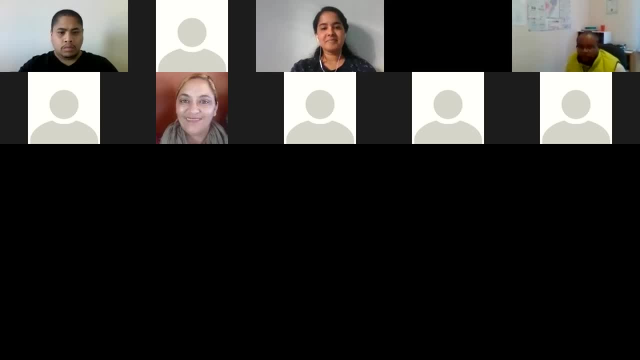 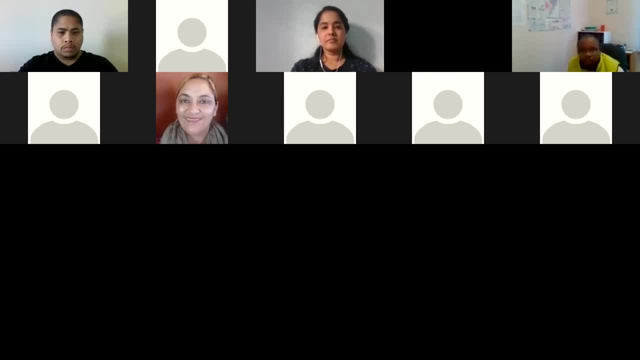 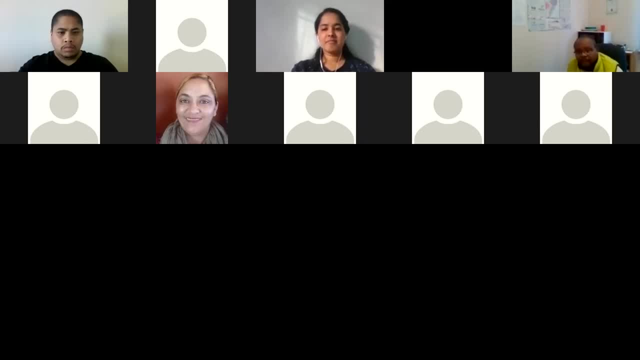 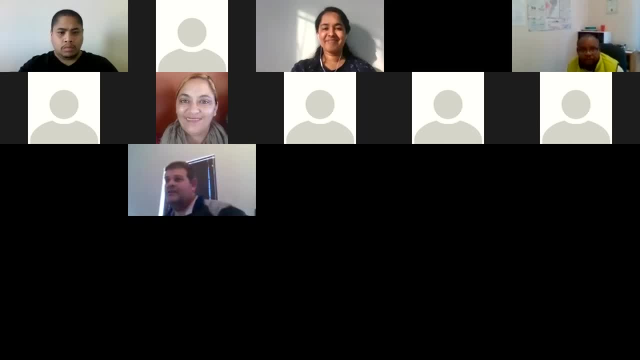 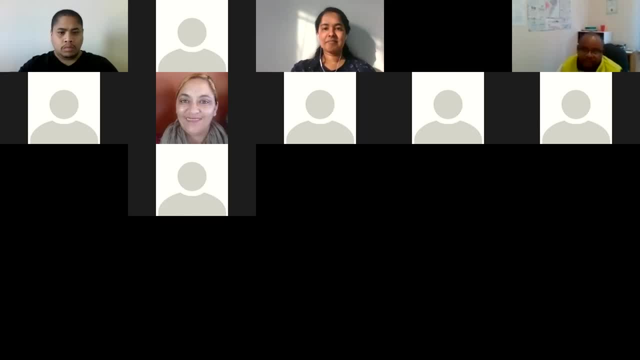 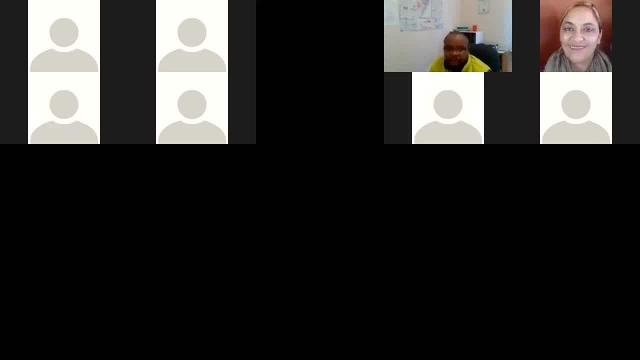 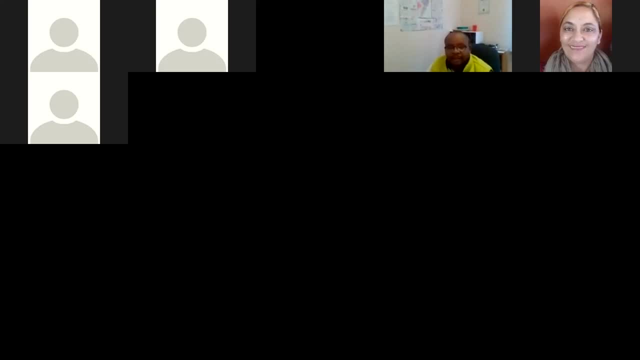 understanding of that. and if you do find microplastics in that specific area and it was a PVC casing, maybe broaden your your understanding of that. and if you do find microplastics in that specific area and it was a PVC casing, maybe broaden your your, your. 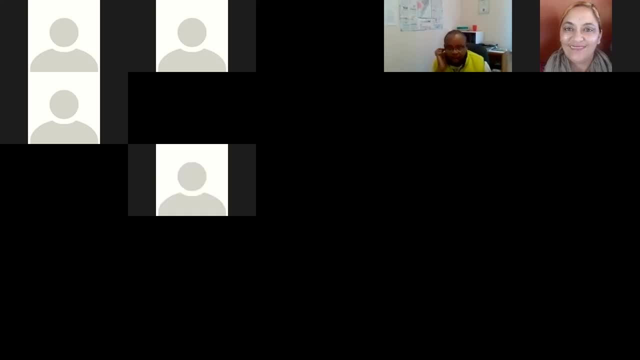 understanding of that. and if you do find microplastics in that specific area and it was a PVC casing, maybe broaden your your understanding of that. and if you do find microplastics in that specific area and it was a PVC casing, maybe broaden your your understanding of that. and if you do find microplastics in that specific area and it was a PVC casing, maybe broaden your your.